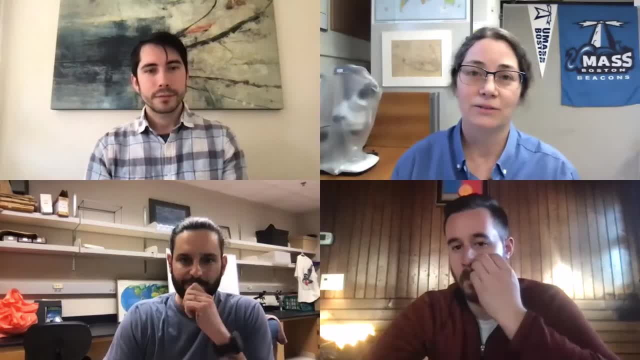 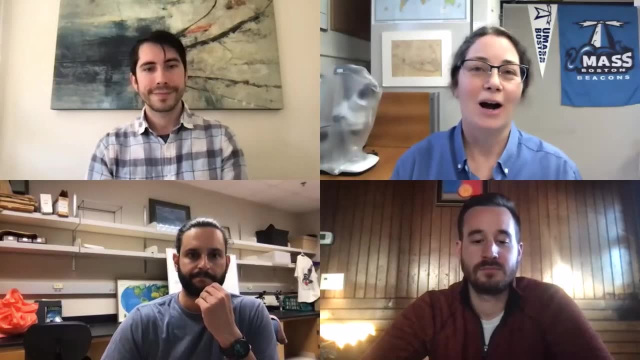 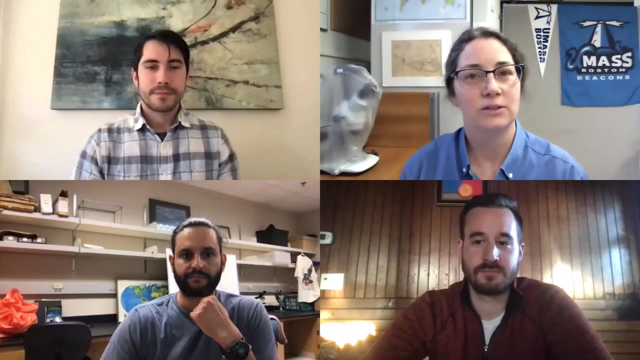 I would first like to say a word about the format of this webinar. We will have two short talks- or maybe not so short- and if you have questions as you listen to each speaker, please use the question and answer chat box. Type your question in. 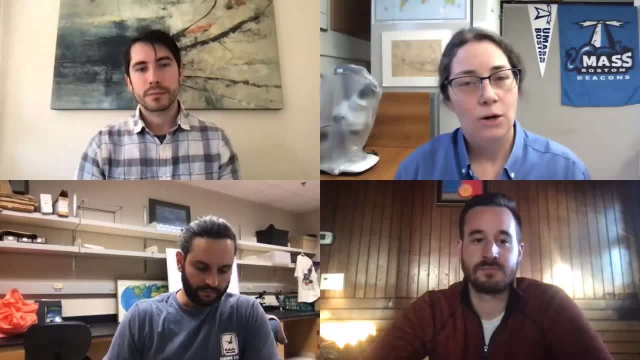 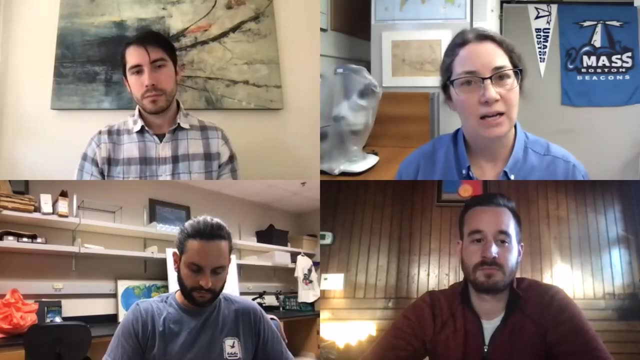 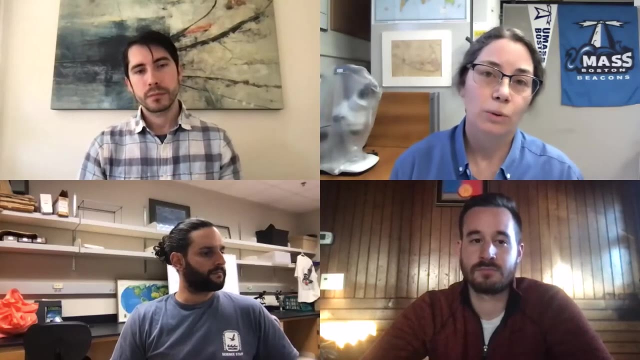 there and include the person's name who you're posing the question to. The sooner you put the question in, we'll be able to ask directly after the speaker finishes the webinar, And that question will be facilitated by Leo. Leo Stella is a student from UMass Boston. 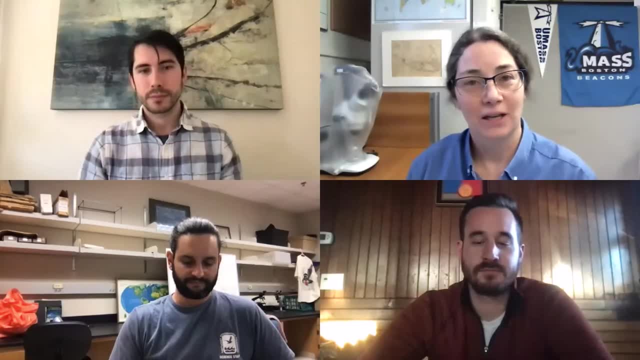 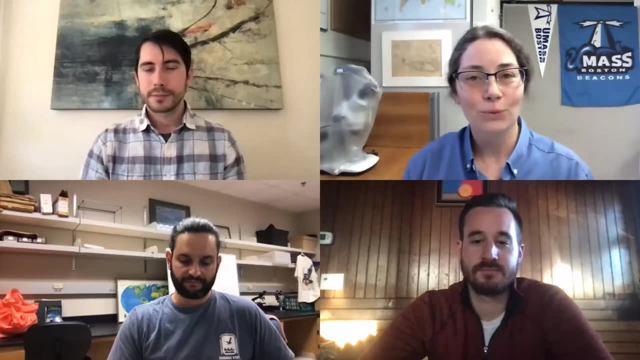 from the Department of Urban Planning and Community Development, and he is assisting us with these webinars, and for which we are very thankful. So, without any further ado, we are being joined by two people who both are part of the Jerry's Program. 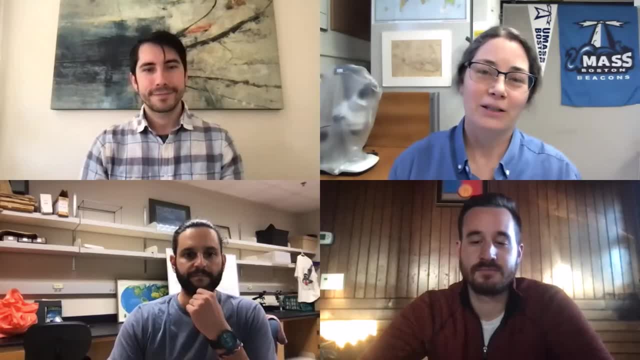 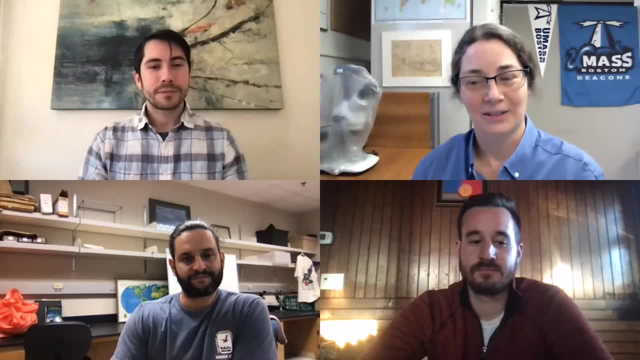 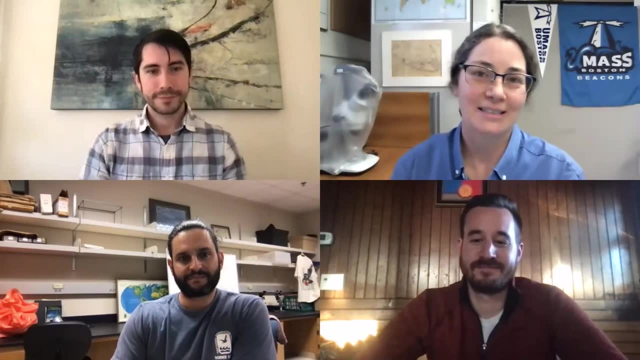 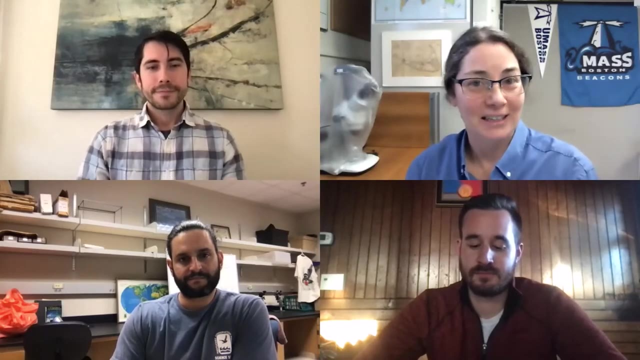 So our first speaker tonight is Mark Hensel, And though he is currently a postdoc at the Virginia Institute of Marine Science, he was part of UMass Boston where he completed his PhD, And people from Nantucket you may recognize his face because he spent a significant 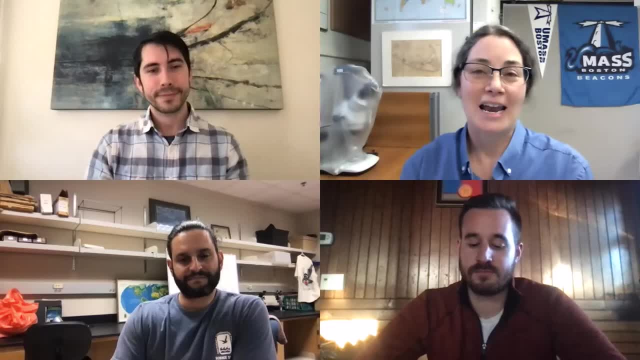 electronic of time on Nantucket and Folgers ensembles, Rather than listen to me. keep going onright now. Okay, Thank you so much. And as always, thank you, You did that. and thankgeois: All hands. Sorry, Thank you. 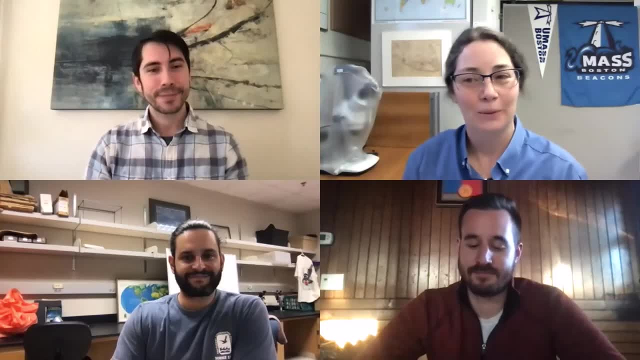 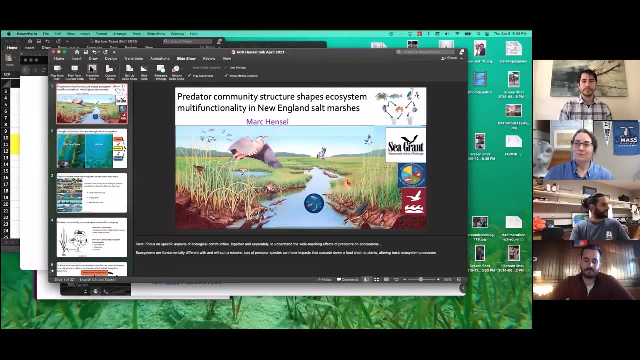 You've now heard what we just learned, So thank you. I will turn the floor over to Mark, so please welcome Mark Hensel. Thank you, Thanks, Yvonne. Let's get this all set up. All right, we looking good. 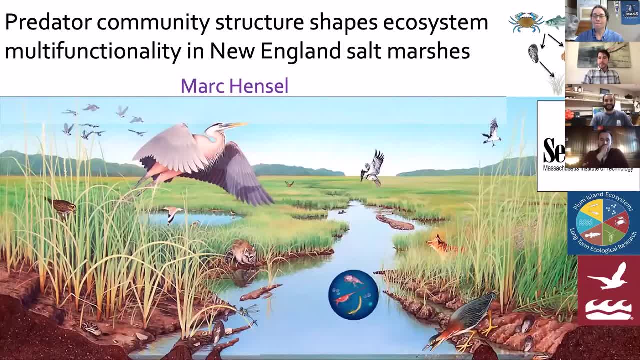 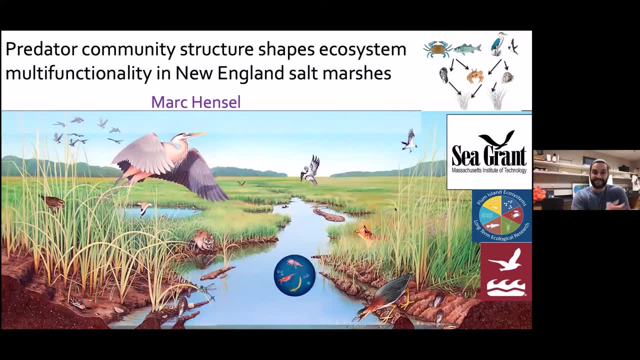 Cool, Okay, so thank you very much for that introduction. I'm really excited to tell everybody about this research today. So this is some research I did during my dissertation at UMass, like Yvonne said, where a big chunk of this was done out on Nantucket And oops. 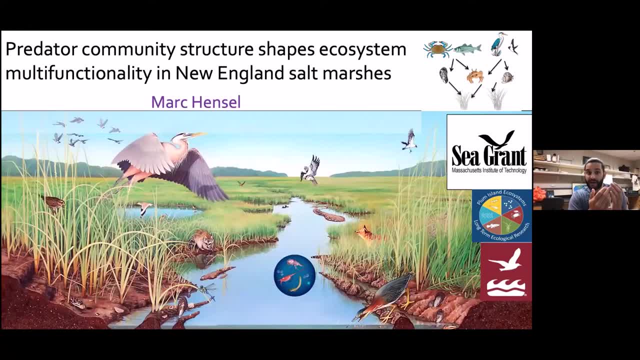 I clicked the wrong thing And basically this is a part of my dissertation that was seeking to understand and describe the wide-reaching effects of predators in New England salt marshes. So ecosystems are fundamentally different than they are in the United States. So ecosystems are fundamentally different than they. 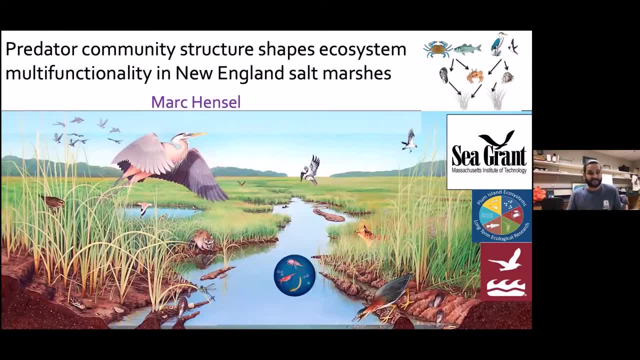 are in the United States, So ecosystems are fundamentally different than they are in the United States. So ecosystems are fundamentally different with and without predators. The loss of predator species can have impacts that cascade down a food chain to plants and altering basic ecosystem processes. A famous example of this is the kelp sea, urchin sea, otter food chain. 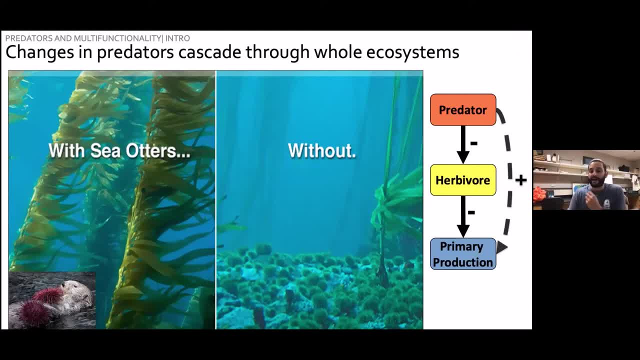 in the Northeast Pacific, where the hunting of otters by fur traders caused a huge increase in their sea urchin prey, which overgrazed kelp forests. This led to the loss of a number of other species that depend on kelp and, importantly, had not been able to survive. 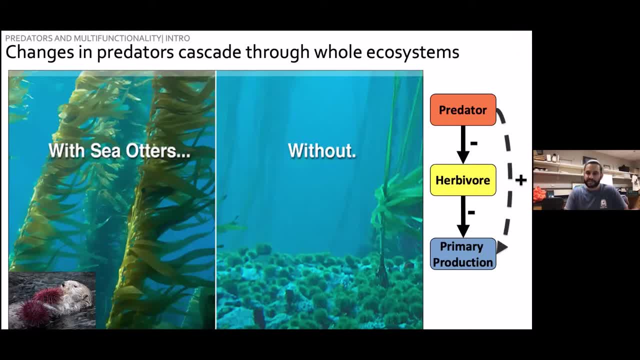 This led to the loss of other species that depend on kelp and, importantly, had not been able to survive. This led to the loss of other species that depend on kelp and, importantly, had not been able to survive. At this point, the 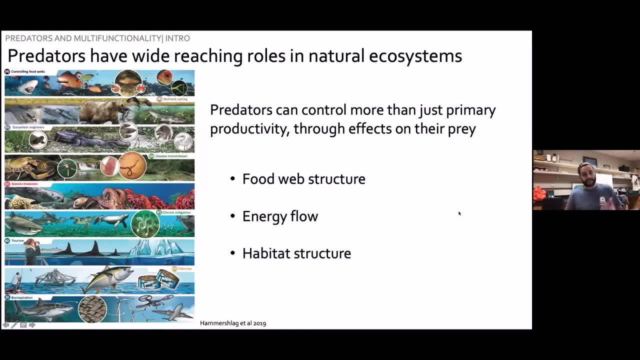 new research had already started to understand that predators actually affect more than just primary production, because predators have wide-reaching roles in natural ecosystems through effects on their prey. So by both consumptive effects- eating- and non-consumptive effects- scaring- predators can control a lot of different ecosystem processes. Predators can control whole. 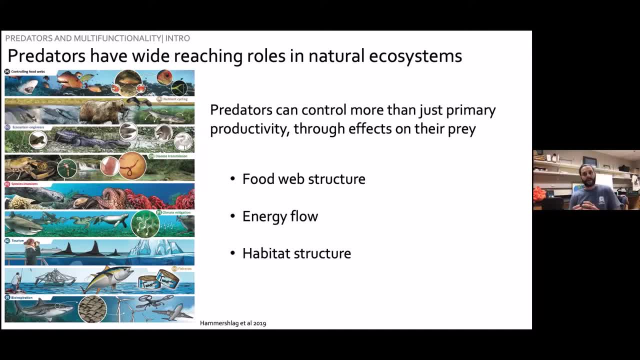 food web structure, not just their prey, but other species as well. The amount of predators in a system can determine energy flow, nutrient cycling as well, and even the structure of habitat in the case of ecosystem engineering predators, And so out in nature, how predators. 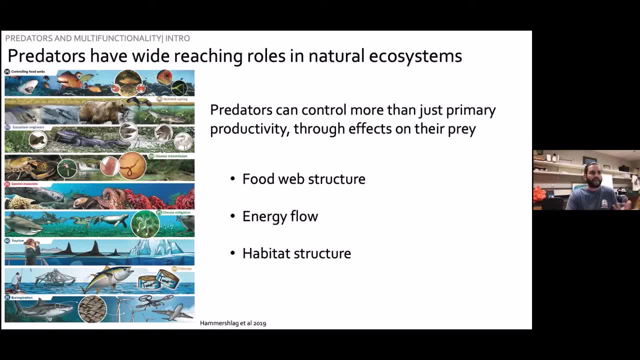 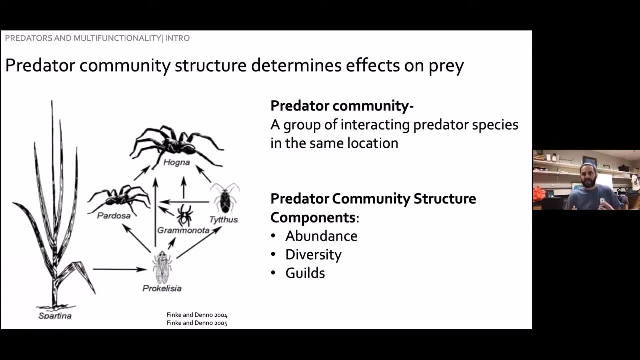 affect their prey is totally determined by what that predator community looks like. So the broad role, the strength and scope of predator effects really depends on basically the group of interacting predator species in a given area. An awesome example of this is in New England salt marshes, where the trophic control of a sap-sucking insect 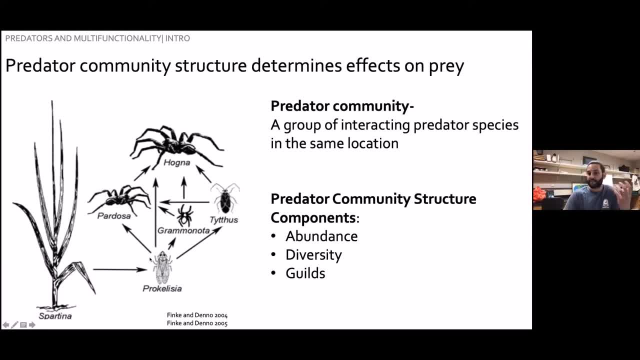 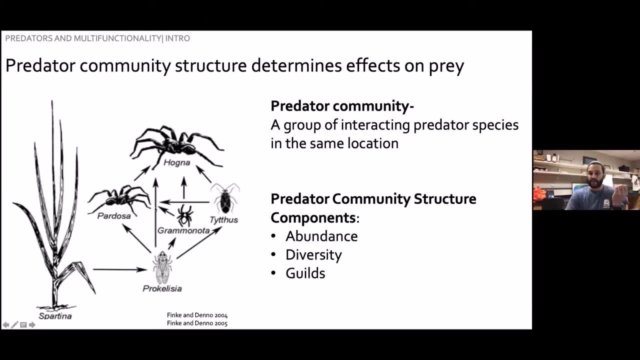 eat the plant hopper, And so plant growth in these areas is totally dependent on predator diversity, the number of species and predator identity which one is present. So these key components of predator community structure really need to be understood to figure out basically how. 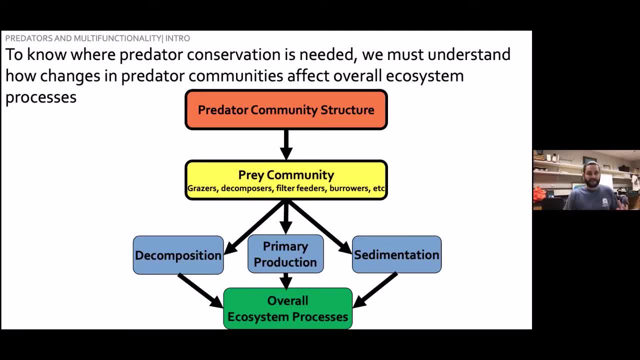 predators affect whole ecosystems and where predator conservation is going to be needed most. So the way that I approach my research on this subject is sort of like this here in this diagram, where predator communities control prey communities and the prey communities do different things: There's grazers, decomposers, filter feeders, burrowers that all affect different. 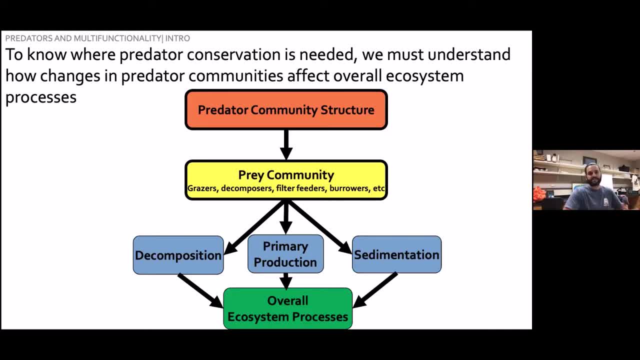 ecosystem processes- we can sometimes call those ecosystem functions, and then, of course, overall ecosystem processes are effective, And so we know a lot about these arrows that I've drawn, but we do not know a whole lot about this arrow here, the indirect effect of predator community structure. 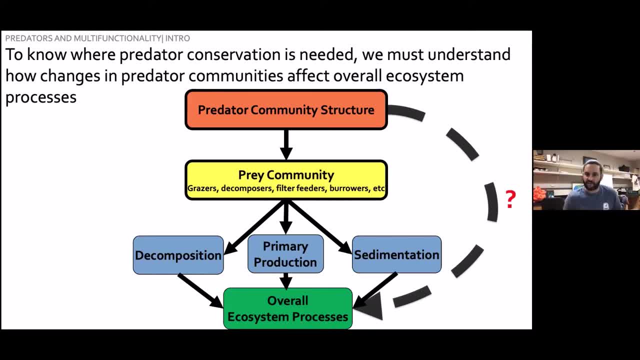 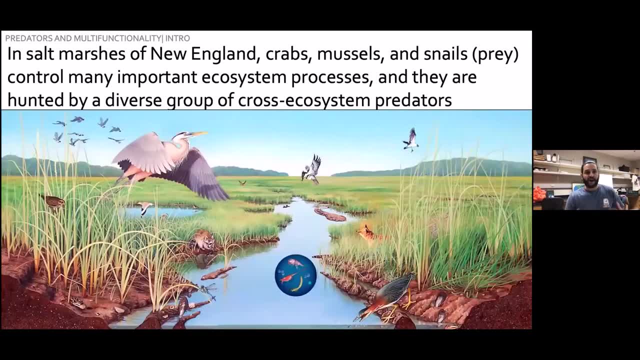 on overall ecosystem processes, because this is a difficult question to tackle and represents a whole new area of ecology. Luckily, salt marshes are an awesome place to ask questions about the role of predators in overall ecosystem processes. In New England, in particular, the salt marshes of 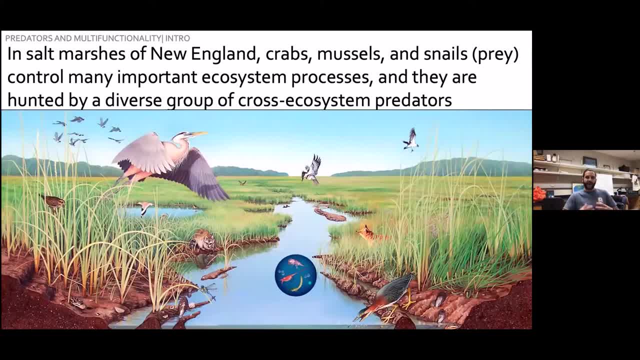 New England have all these resident invertebrates: crabs that are burrowing or herbivores, filter feeding mussels, snails that decompose dead tissue, that all control and help control many important ecosystem processes. These invertebrates are all hunted by a really cool 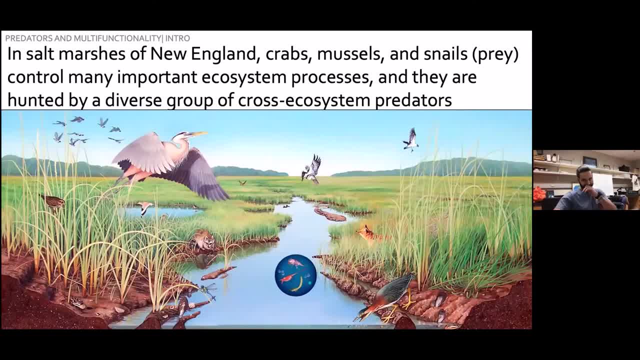 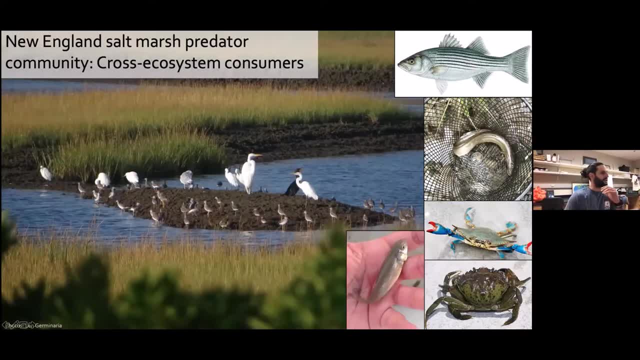 diverse, abundant group of cross-ecosystem predators. So as the tide goes out and low tide is exposed to the creek bank, birds come in and feed on the marsh edge- This picture is taken by Lenny- the edge of Folgers Marsh. 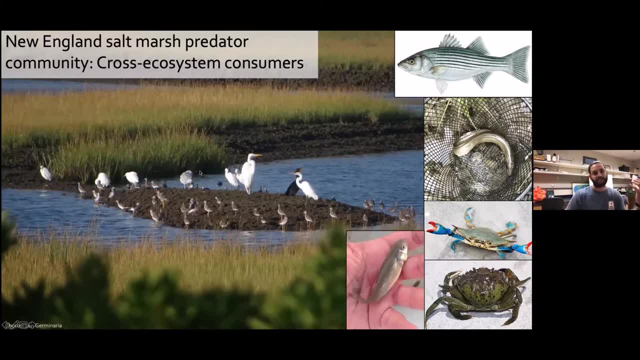 And then, when the tide comes up, from the marine side of the food web, species like striped bass, eels, blue crabs, green crabs, mummy chugs, come into the marsh and take advantage of all these resources too. And so this is the New England salt marsh predator community And the way that 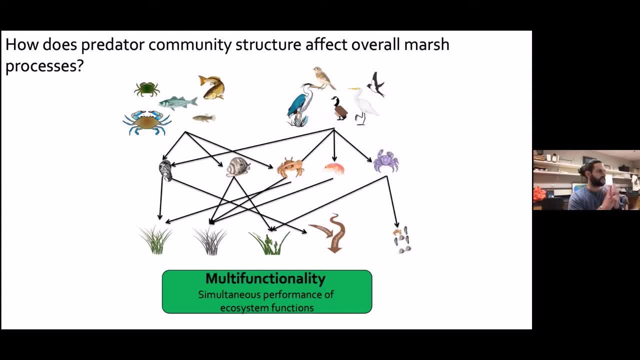 I've structured my research questions kind of go along with this picture right here. basically, where there's a marsh predator community, birds, fish. This marsh predator community has different guilds and from marsh to marsh they vary in abundance, in diversity, in the number of species These predators control. 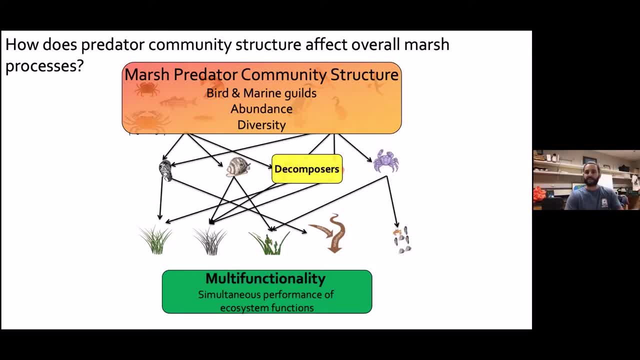 these predators feed on prey that are like decomposers, herbivores, burrowing crabs, filter feeders, which then, in turn, of course, affect the different ecosystem functions like primary productivity, decomposition rates, sedimentation rates, the way in which sediment 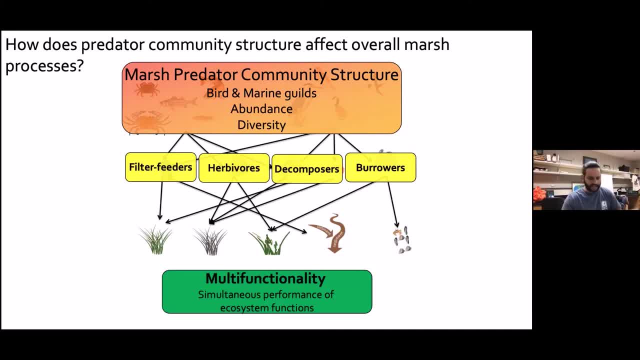 is deposited onto the marsh, And so we know a lot about these arrows right here, how predators affect their prey, how prey affects ecosystem functioning, And my research is, then that I'm going to talk about here. I used experiments and surveys to sort of understand this, this dotted arrow as well. 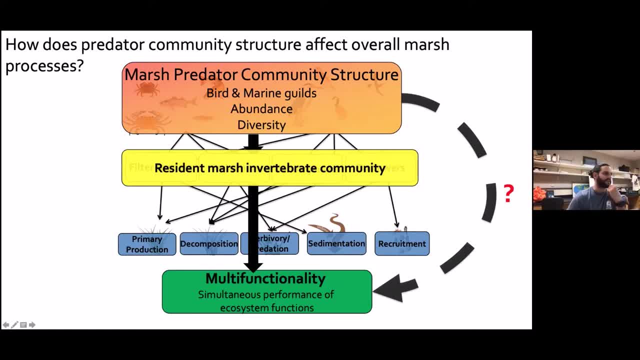 Really quickly. I just want to define one term that I'm going to use just a little bit, which is multi-functionality. This is the simultaneous performance of multiple ecosystem functions. So these different ecosystem functions here, basically what multi-functionality is. 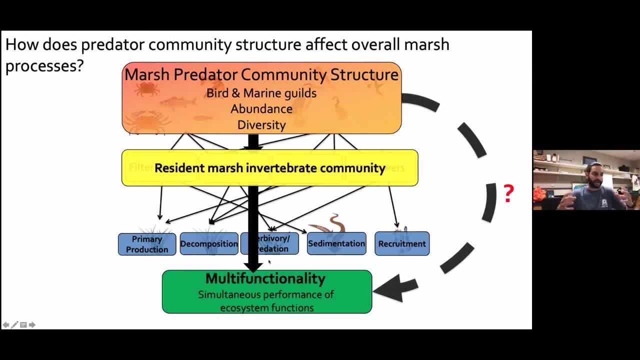 is just a way to summarize the overall combined rate of a bunch of different processes at once, So it helps us look at overall process. So to address this, how do predator community structure affect overall marsh processes? I have a two major reasons. The first one is that you know there's a lot of 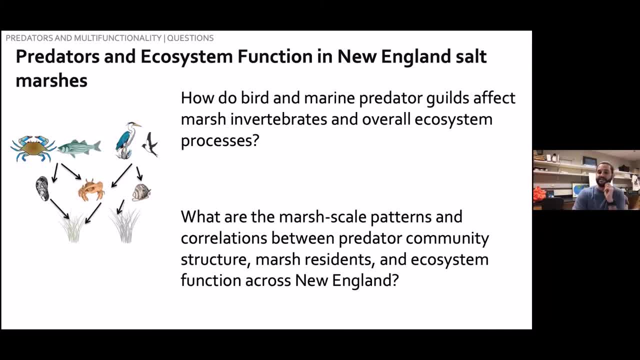 research questions that I mentioned. I used experiments and large-scale surveys to understand or to answer, excuse me. So first, how do bird and marine predator guilds affect marsh invertebrates and overall ecosystem processes? So to answer this question, I did a manipulative. 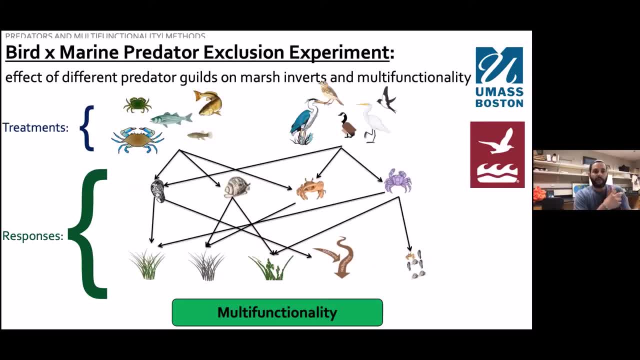 field experiment in Folgers Marsh where I manipulated the presence or absence of these predator guilds and I measured the rest of this diagram. I measured the community structure, so the resident invertebrates that live there and these ecosystem processes, How I manipulated these predators in Folgers Marsh along the creek banks, I had these two. 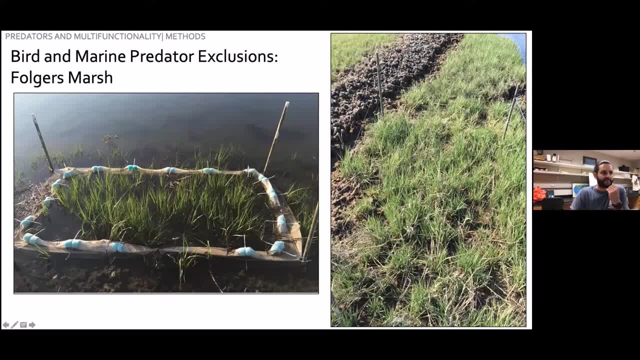 by two meter plots where I either excluded birds- that's what this picture is on the right. it's tough to see which is the point. this is a fishing line wrapped around PVC poles, and sometimes I use some flashing tape as well, so I can't really see what's going on, but I can see what's happening. 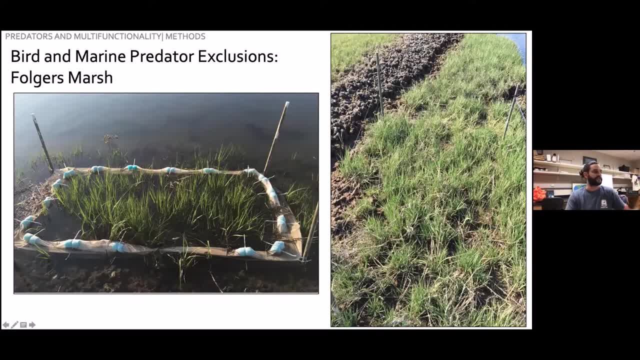 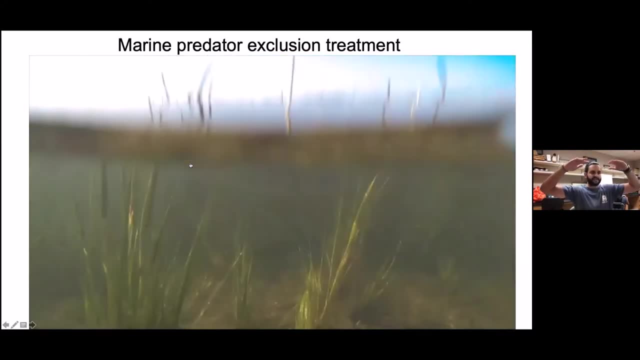 So I did a little bit of tape as well as a visual deterrent to exclude birds And then to exclude marine predators. I built this cage here, which is a floating net cage. I've got a little video that hopefully plays okay, where, as the tide comes in, the water raises the floats and no fish or 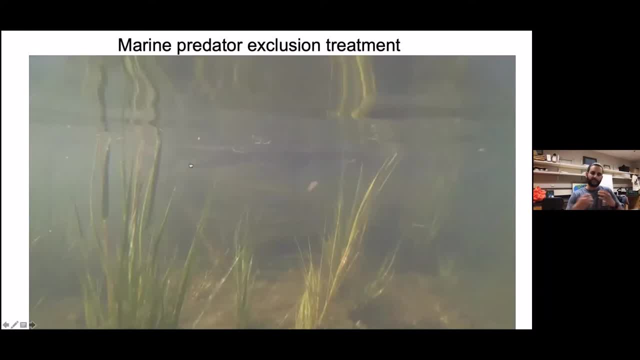 crabs or anything can swim into this. I have treatments where both are excluded and neither are excluded. So over the course of the growing season I've been working with a lot of bird and marine predators. I measured invertebrates and ecosystem functions. So what did we see? 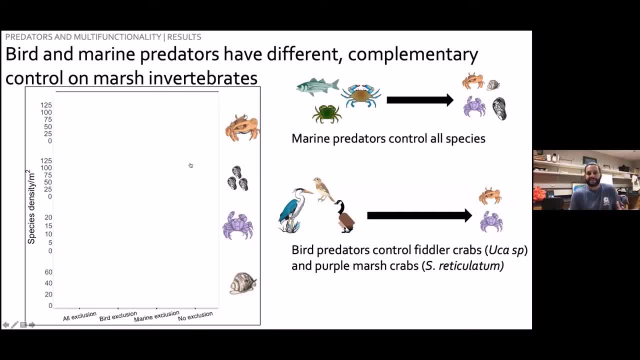 So at the end of the experiment I found that birds and marine predators have different effects on the marsh invertebrates. So I'm going to show the graph on the left, but it's a little bit complicated. It's much easier to just look at my pictures on the right. 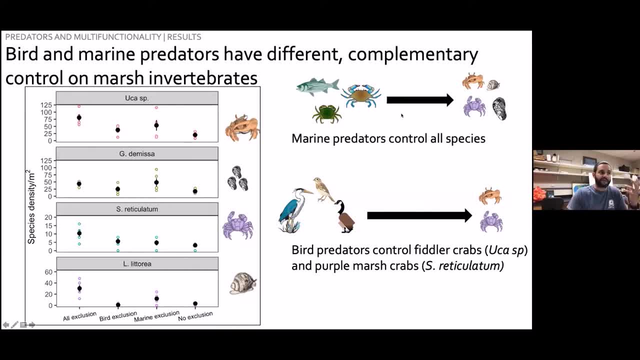 but what I found was that marine predators, so the crabs and the fish, control all the different prey species that I measured. But bird predators in fact only had an effect on crabs, on the burrowing fiddler crab and the herbivorous purple marsh crab, So importantly. 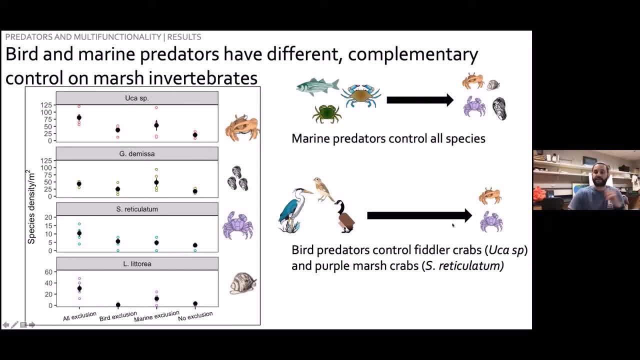 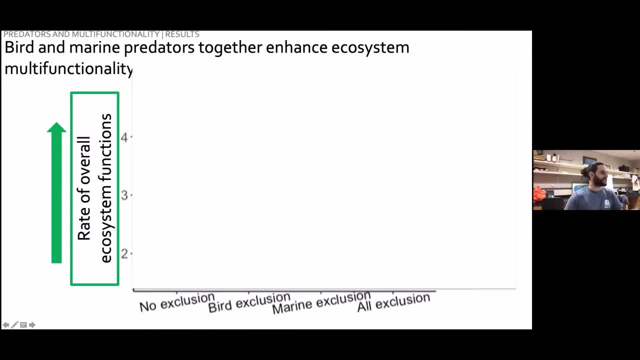 bird and marine predators do different things. Sometimes they complement each other and sometimes they don't. How does this translate, then, to ecosystem function? So here on this graph, this is the rate of overall ecosystem functioning, where higher numbers mean the more processes that are occurring at higher rates. And my different 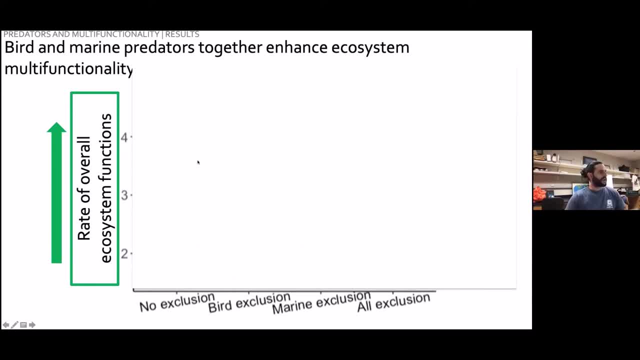 treatments down here, which you don't need to worry too much about. what I found was that the plots that had the highest amount of functioning were the plots where all predators were allowed in, And in fact, the lowest combined rate of ecosystem function occurred where no. 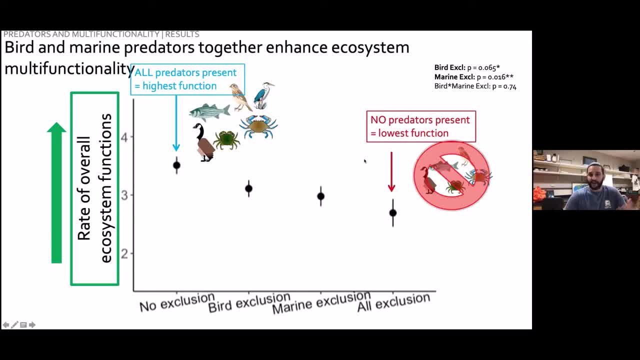 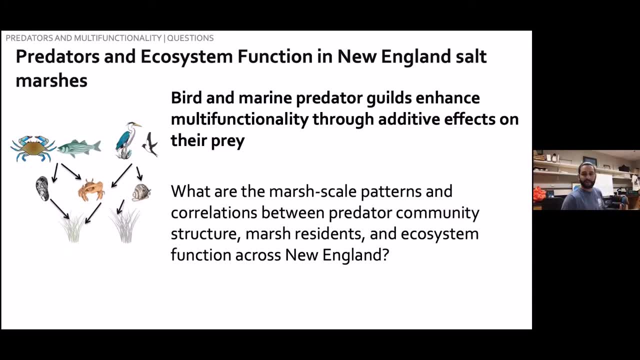 predators were present, So bird and marine predators together enhance ecosystem multifunctionality in my experiment through these additive effects on their prey. So this is a really interesting result And I think this told us a lot about what happens along the creek banks in plots. 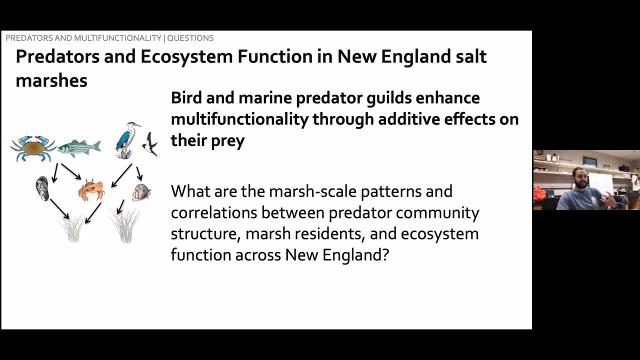 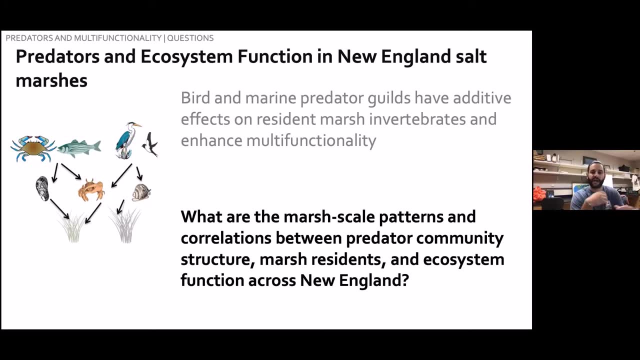 in a manipulative experiment. But I also wanted to understand, basically, how does this scale up to the whole marsh And how does this scale up to places that aren't Folgers Marsh as well? And so to get at that question number two, what are the marsh scale patterns and correlations? 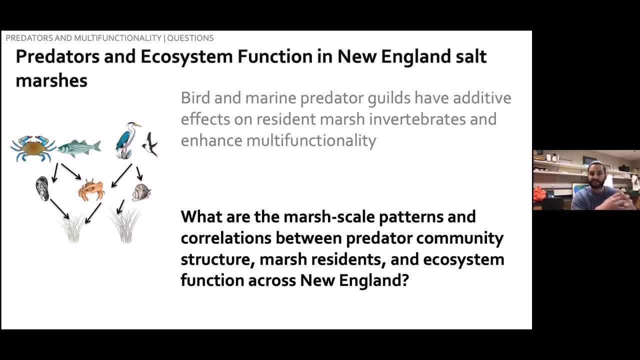 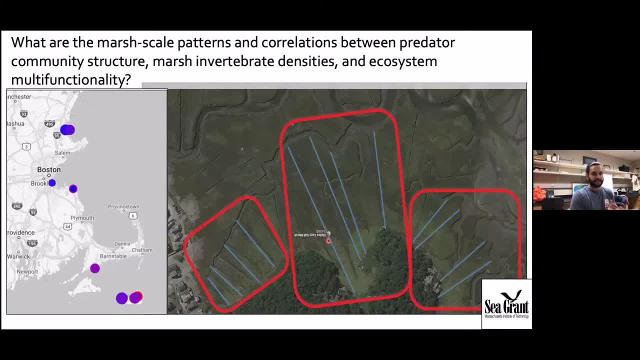 between predator communities, the marsh, invertebrates and ecosystem function Across New England or across Massachusetts. really, This was a MIT Sea Grant-funded project. I started right when I got up to Massachusetts and working with Jarrett And basically what we did. 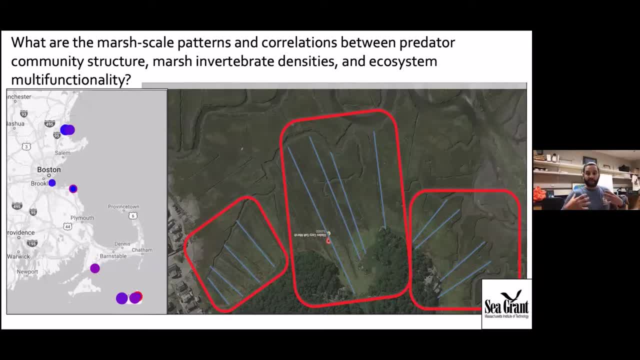 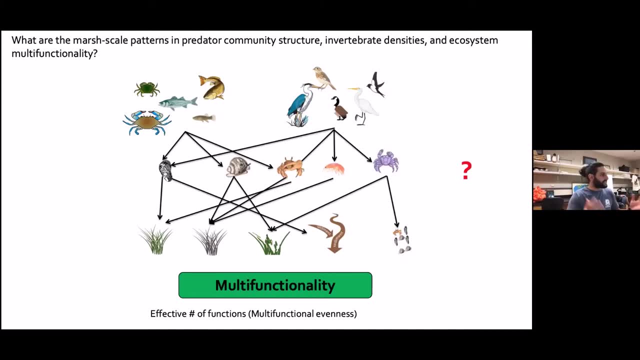 so these are our sites on the left. here is: we went to all these marshes and chunked them up into these three different zones And we went out there and quantified everything you're looking at here: all of the predators, all of the invertebrates and all these ecosystem functions. 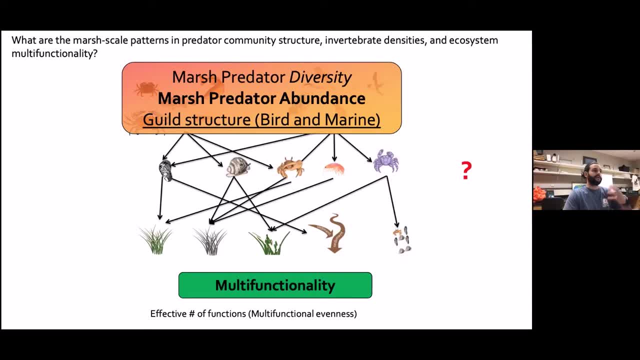 And then we looked at relationships between the predator community. So marsh predator diversity, how many different species, the abundance of all predators and then also within the guilds, bird and marine. We measured again marsh invertebrates and quantified all these different. 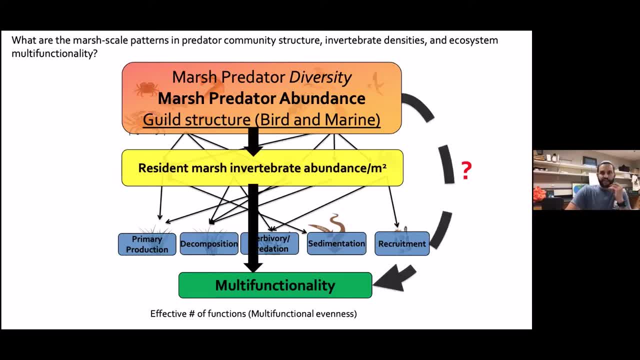 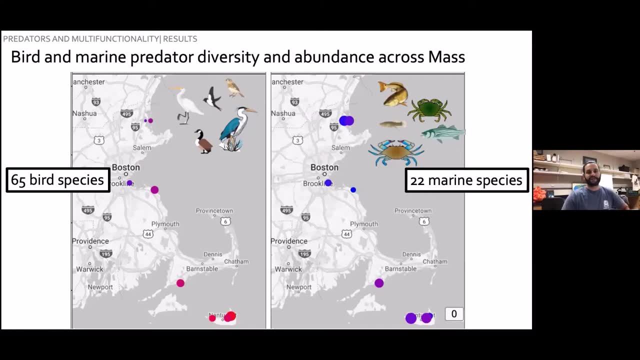 ecosystem functions, And so I'm going to walk through basically each of these black arrows and the direction of each of these, But really quickly. first, since this of this talk, I do want to point out the patterns in bird and marine predator diversity. 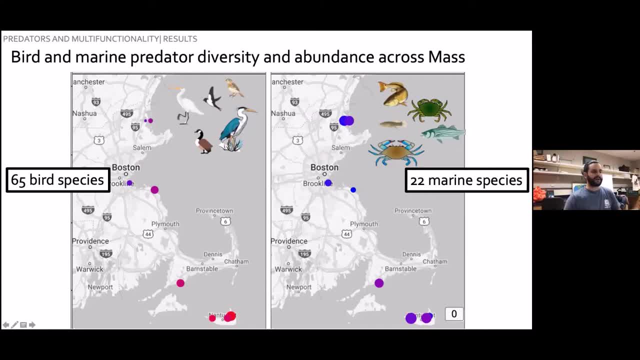 across Massachusetts. So on the left this is birds, On the right is marine species. Each of these circles is one of the sites. The size of the circle is abundance And how red it is is richness. We found 65 total bird species across our surveys, 22 total marine species. 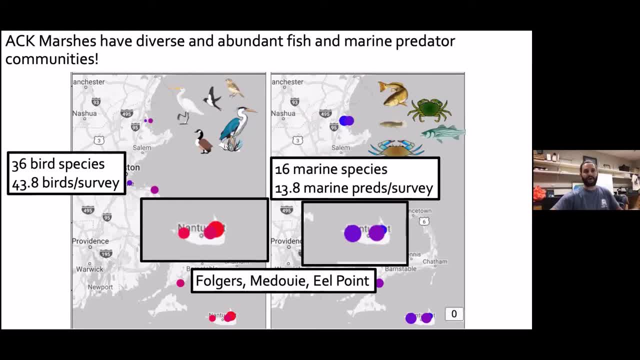 And I in particular wanted to point out how well performing the Nantucket marshes were. So the three marshes that we surveyed here were Folgers, Madawi and Eel Point, And basically Nantucket marshes in our surveys were the most diverse and most abundant. 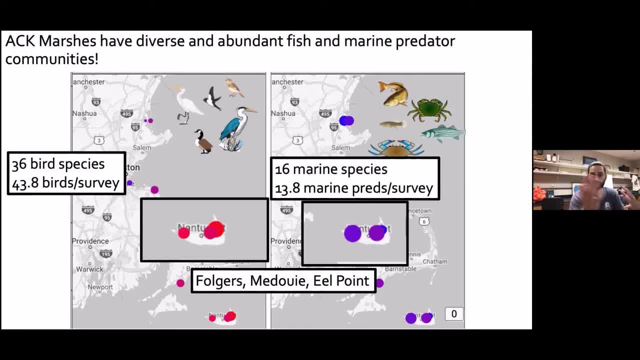 fish and marine predators throughout the places that we surveyed: 36 total bird species- I think that was in Madawi marsh, 16 total marine species in Folgers marsh. So this is actually why I decided to do the experiment where it was. But it was kind of cool that Nantucket had such good 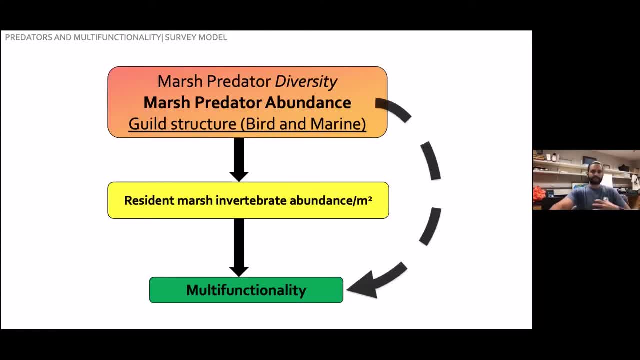 abundant, diverse fish and predator communities. So what does that mean? though, Not all marshes have all the birds and all of the fish right, And so to understand that variation, we're going to look at this diagram here. So first, the relationship between marsh invertebrates and multifunctionality. This 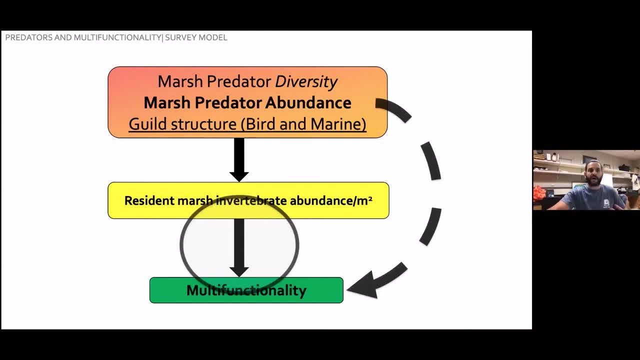 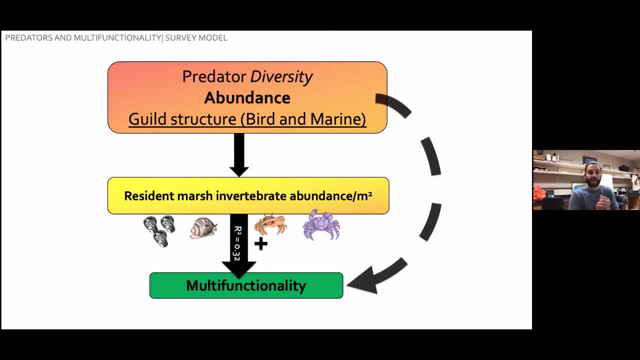 is actually something that's been teased out in experiments before Marsh. invertebrates have a positive effect on multifunctionality, And this was confirmed again in our surveys, where muscle density, snail density, fiddler crabs- they all increase the rate of multiple processes happening at once. So what about the effect of? 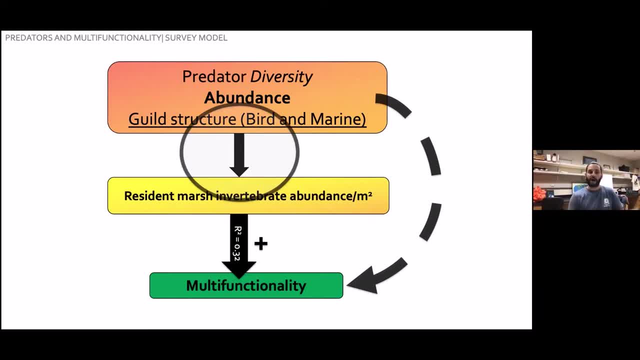 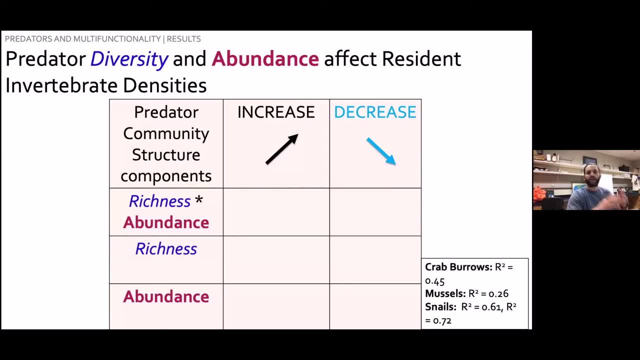 predator: community structure, diversity and abundance, bird and marine on the resident marsh, invertebrates. So, as you can guess, there's a lot of different predators and a lot of different invertebrates. So I'm not going to show a bunch of graphs, I'm just going to pop up this table here. 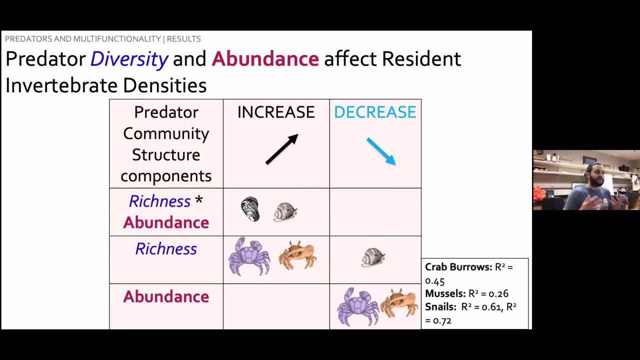 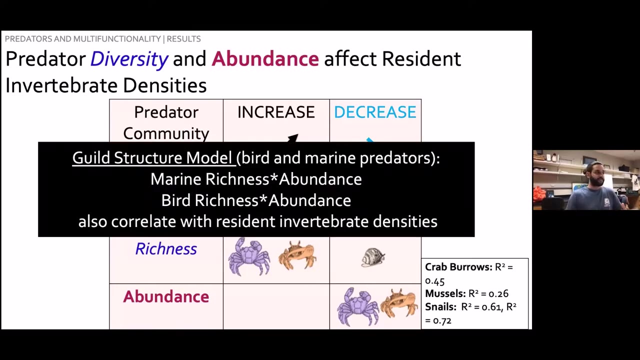 and show that predator diversity and abundance both affect invertebrates in different ways. Abundance generally decreases the predator abundance generally decreases invertebrate abundance. But basically there's complementary effects of both species- richness in predators and abundance. And when we look at birds and marine predators we see a similar pattern where there's an interaction. 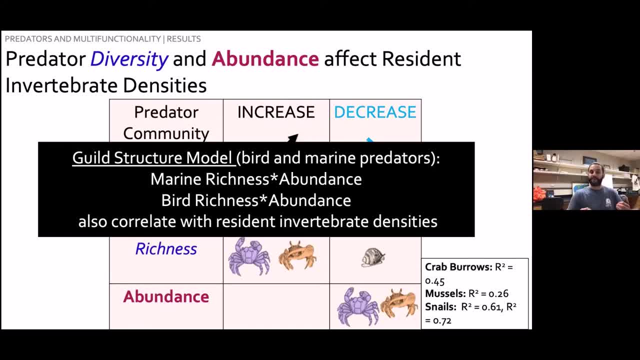 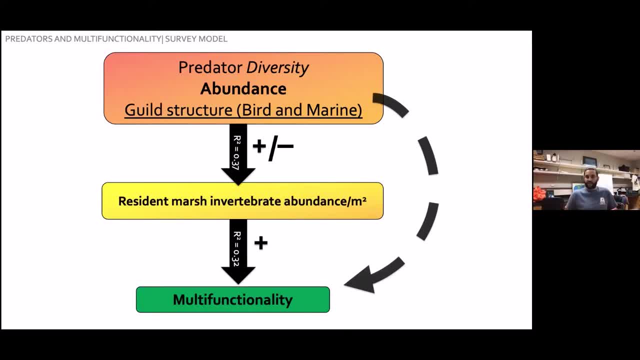 between richness and abundance, both within marine and bird predators, correlating with resident invertebrate density. So, again, similar to what we saw in the experiment, bird and marine predators and predator diversity and abundance do have different strong effects on their invertebrate prey. So now, what about this last connection here? 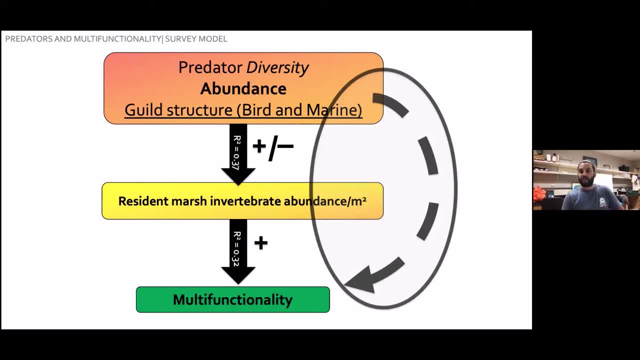 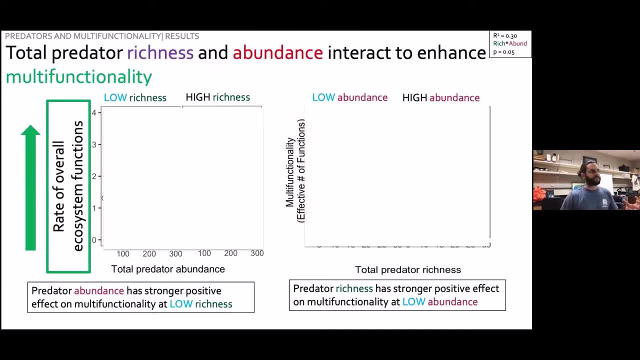 How does predator community structure affect multiple ecosystem functions? So I'm going to show a couple of different graphs here, but basically the main point is that total predator richness and abundance together interact to increase the rate of ecosystem function, And it's really cool because they kind of compensate for each other. So on the left here, 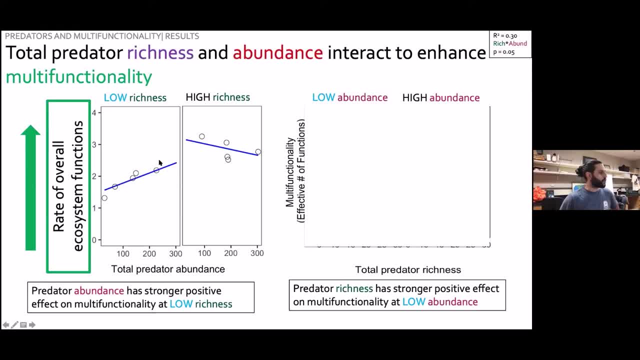 I have two plots. This is marshes that have low predator richness, and this is a marsh that had high predator richness, And so increasing predator abundance has a stronger positive effect on multifunctionality at low richness. And then the flip side of that is also true, which is really. 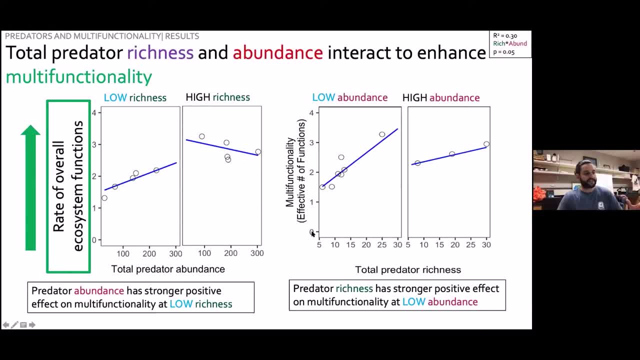 cool. That means that predator richness, increasing the number of species, has a stronger positive effect on multifunctionality at low abundances. So again there's this really interesting compensation between abundance and diversity, And it makes sense that the most abundant and diverse marshes would be the most multifunctional Within the guilds we found. 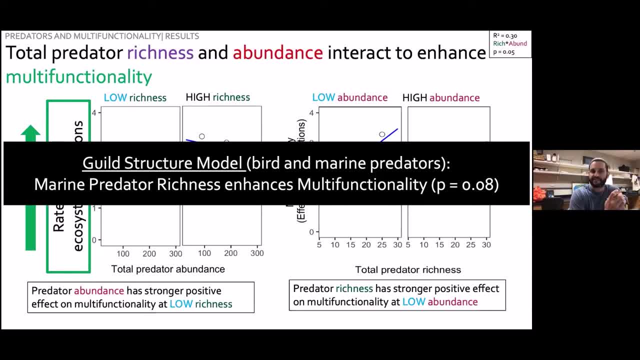 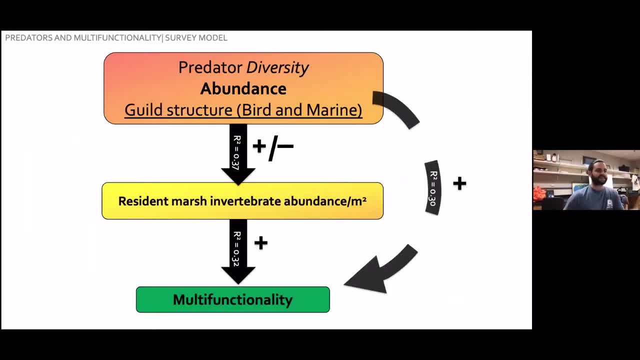 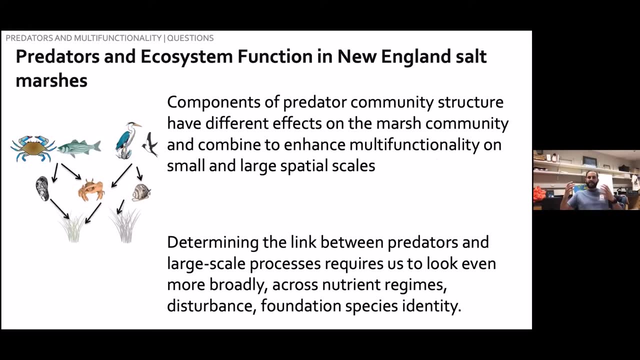 that not birds but actually marine predator richness did increase ecosystem functioning as well across all of our surveys. So this is what our sort of final diagram looks like here, with this indirect positive effect of predator communities on multifunctionality. This is a really neat finding because those different components of the predator community have 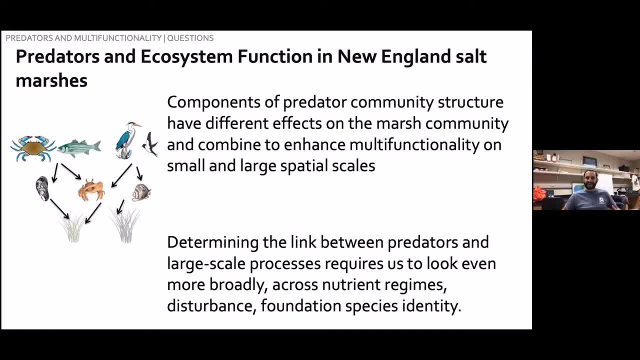 different effects on the marsh, on the marsh invertebrates, And that combines to increase multifunctionality, both on small experimental scales and on large whole marsh scales, And so what this means is to determine this link between predators and large-scale processes. we have to look more broadly across nutrient regimes under different 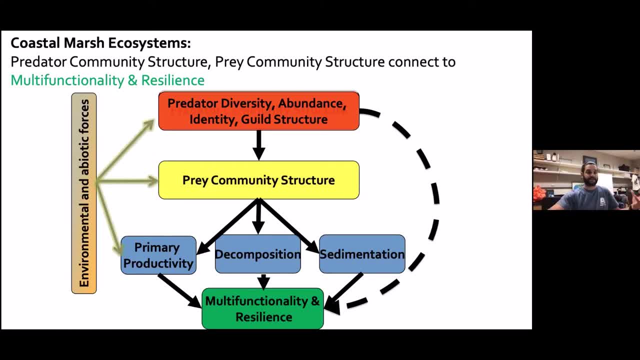 levels of climate change, And so the final sort of diagram looks something like this: where environmental and abiotic factors sort of affect everything. Predator diversity and abundance and identity are all important And multifunctionality is related to ecosystem resilience. where an ecosystem that's performing 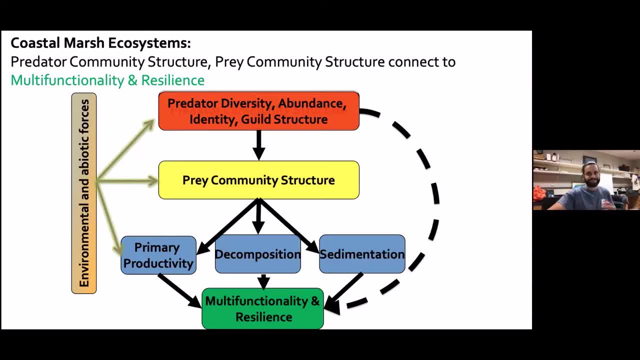 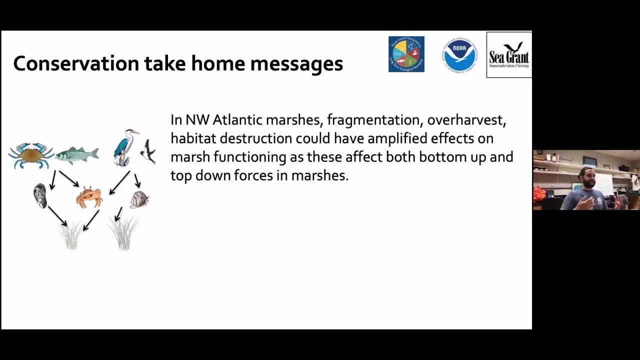 more functions at higher rates is going to be more resilient over time. So from a conservation standpoint, there's a couple of big take-homes that I just want to point out. One is that in Northwest Atlantic marshes, fragmentation, overharvest, habitat destruction are big threats. 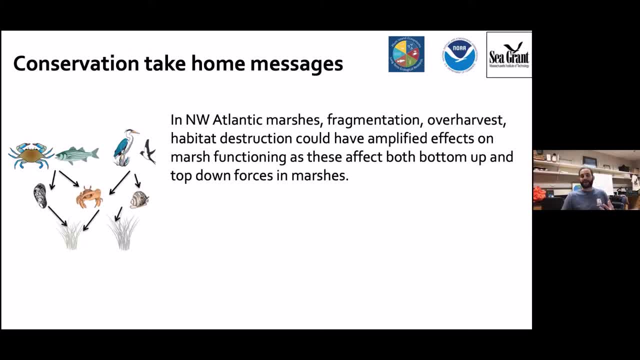 to marshes as a whole. These are also things that will affect predators, So that means that there's the potential of amplified effects, both from bottom-up standpoint and top-down forces in marshes if these things continue to go unchecked, And also when it comes to the conservation. 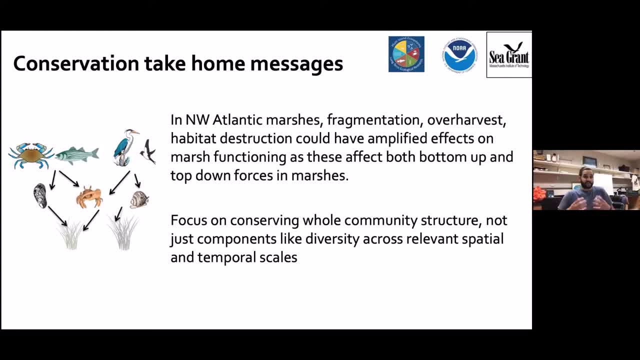 standpoint, especially with predators, we have to focus on conserving the whole community structure, not just its components like diversity, because that's what becomes really relevant across large spatial and long temporal scales. So with that, I'd like to thank a lot of different people. 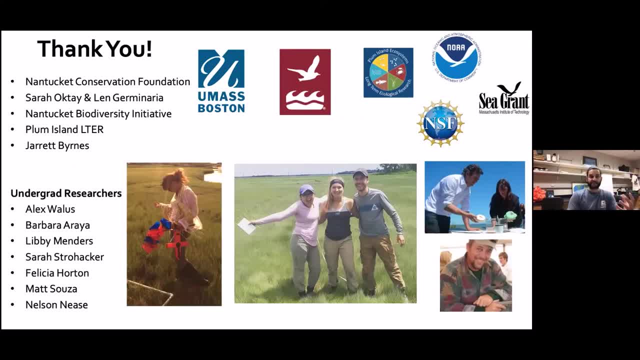 So a ton of this research was funded through the Nantucket Conservation Foundation. Obviously, a big chunk of it also took place on Nantucket as well, So big thanks to them and to the NBI as well, And to my advisor, Dr Burns. this was a project that we started right at the beginning of my 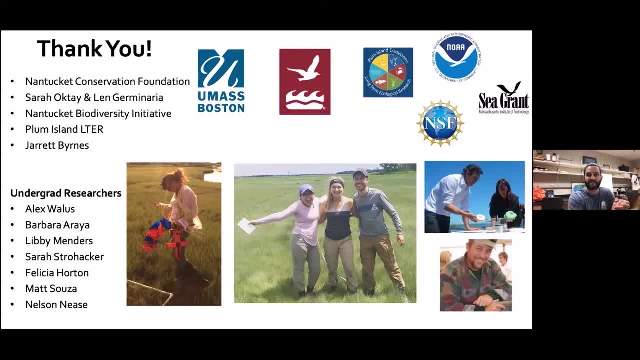 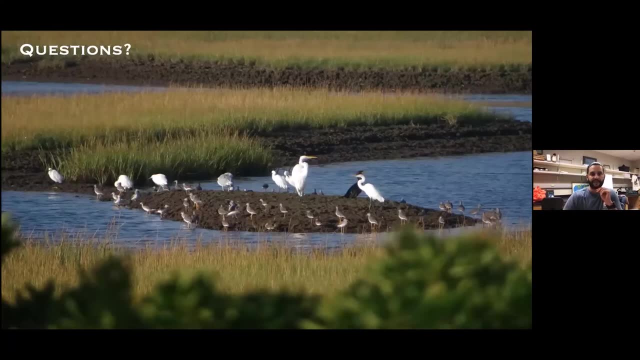 dissertation and carried all the way through and it's still going now, And so I'm really excited for the future of this work, Had a number of really good undergraduate researchers help me out throughout the course of this project And with that I'll turn it over to Leo to ask any questions. 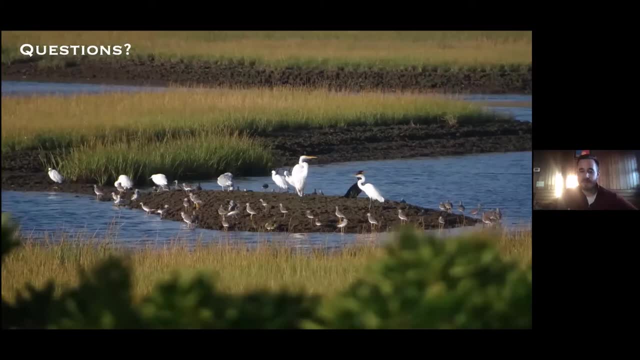 Awesome. Thank you, Mark. People are maybe being a little shy. We don't have any yet in the question and answer portion. Just so folks know, there's a chat feature and a Q&A feature and I don't believe that I can. Oh, look at that. Yeah, I can allow. 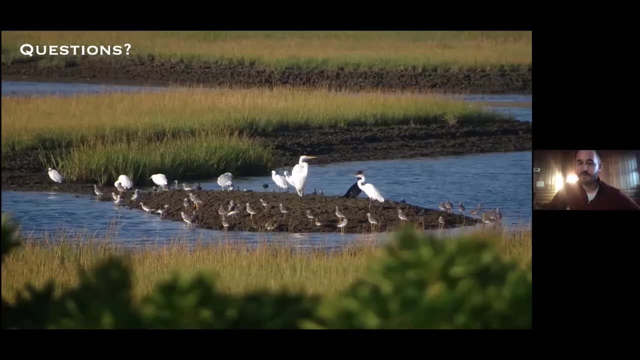 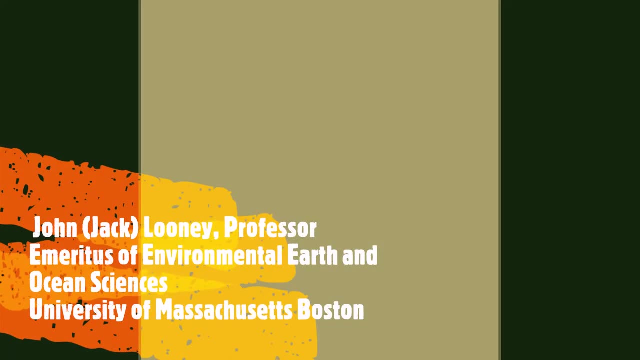 John to talk here, So I'm going to allow John to ask his question. I think that when I think of ecosystems, I think of a basic equation: A plus B equals E. You focused mainly on the biota, and yet you mentioned spatial and temporal issues. 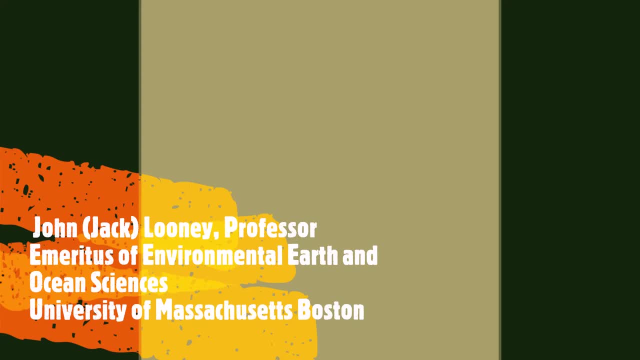 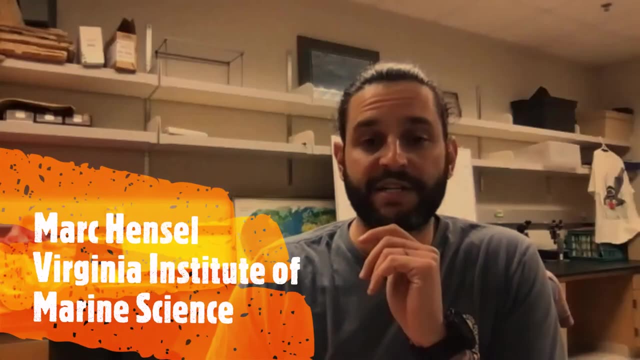 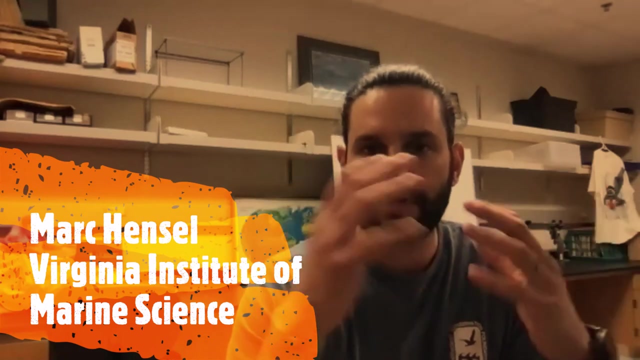 Did you do anything regarding the abiotic factors or did you just concentrate on the biotic factors? Great question, John. And really, if you scale up the diagram that I have of how I envision everything working at the end, that's where different abiotic and environmental changes. 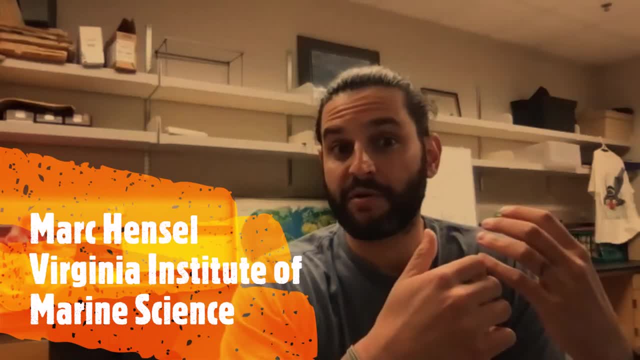 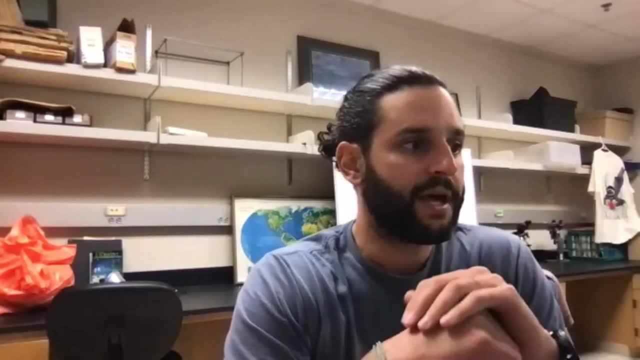 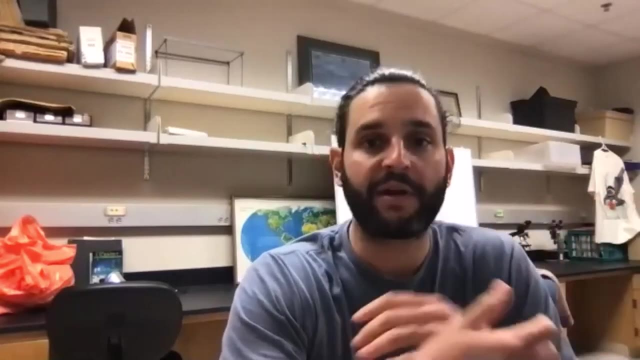 can potentially come into play. So I did a number of things to control for differences in abiotic forces and environmental forces, For example. even when it comes to the food web surveys itself, we try to do those in the same time of year to catch, so we're not getting migratory. 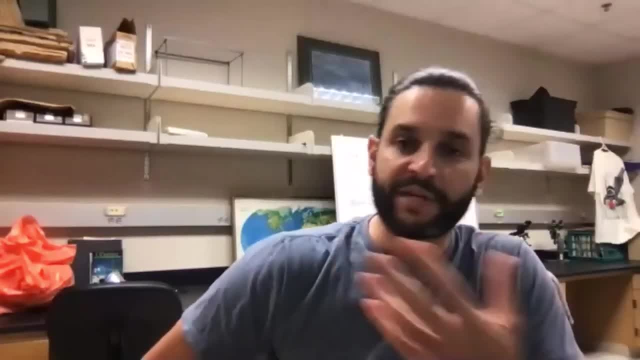 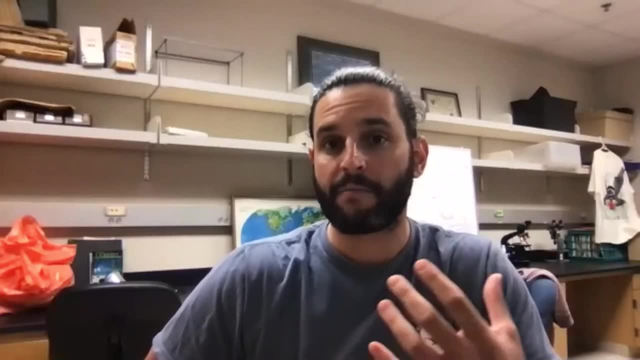 birds at different times of the year and stuff like that. And then we try to select marshes of similar size with similar creek size, which has a big effect on large-scale processes like sedimentation rates, that sort of thing. So we did do something to control that, But I don't know if 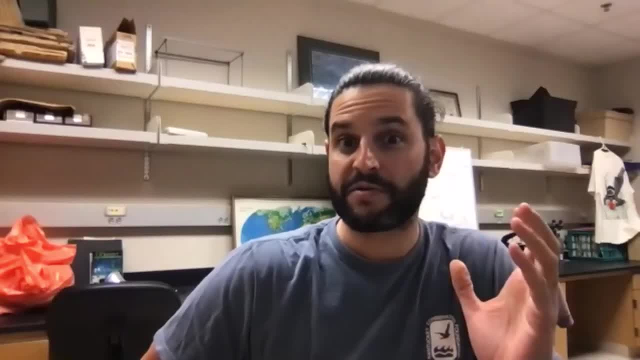 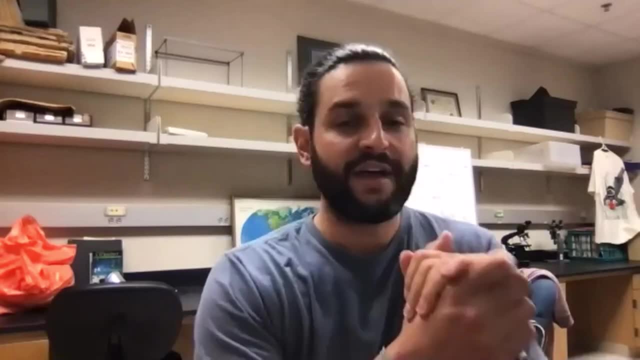 We did do as much as we can to make sure that those differences in abiotic forces are the same in a lot of different marshes. but as for, like you know, sort of explicitly working that into our models and stuff, that was not something we were able to do for this project. 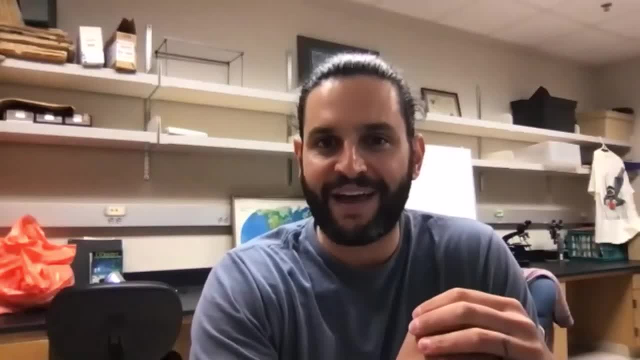 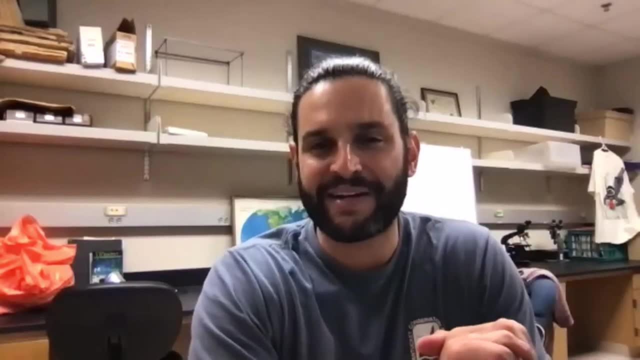 but I mean that's sort of an overarching goal in ecology in general- is to be able to basically handle it all. and you know it's not something we did with this project, but definitely something that's on our mind. So yeah, good question. Familiar with Plum Island and Belle Isle? 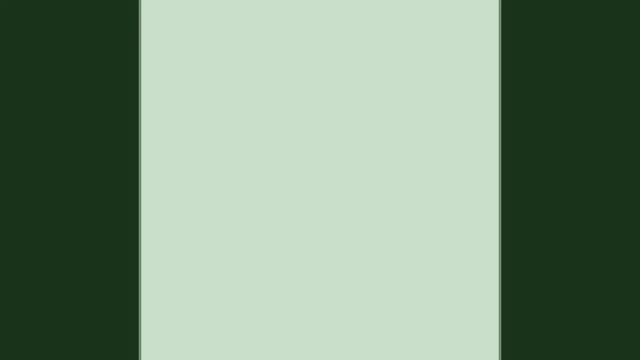 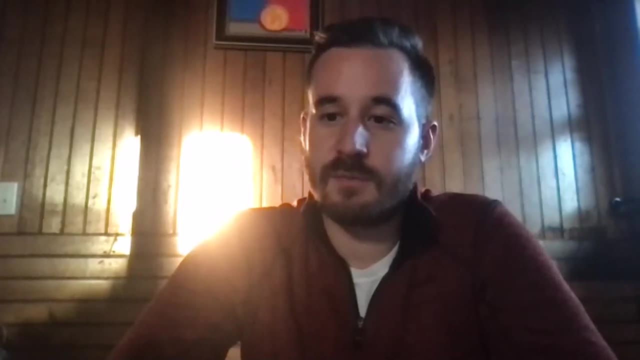 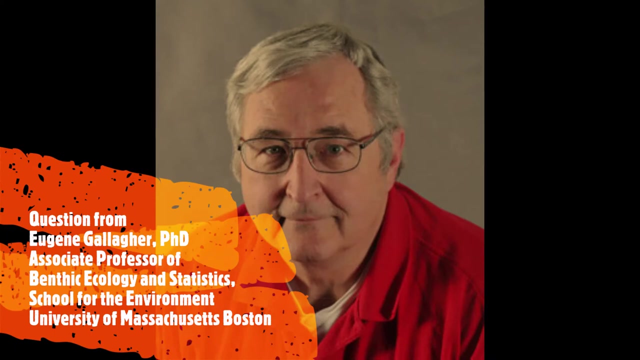 and also Folgers, and they are different, and that occasioned my question. Okay, we've got another question here in the chat, so I'll just read it out. The question here is: when Bernstein excluded blue crabs from Chesapeake Bay, what was the result of that? 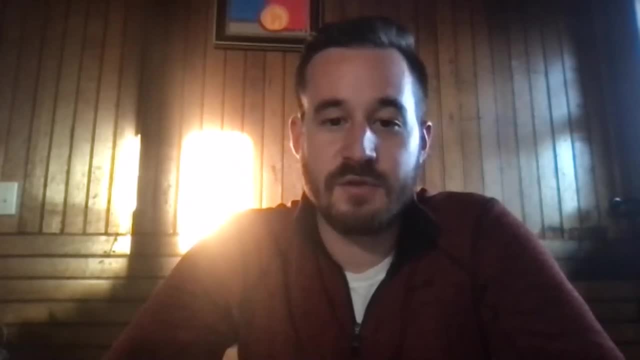 The question here is when Bernstein excluded blue crabs from Chesapeake Bay. The question here is: when Bernstein excluded blue crabs from Chesapeake Bay? benthos infaunal abundance increased dramatically and so too did benthic infaunal species richness. Do New England marsh? yeah, do New England marsh benthic? 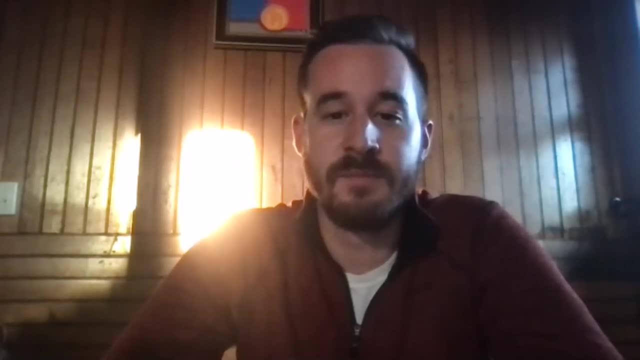 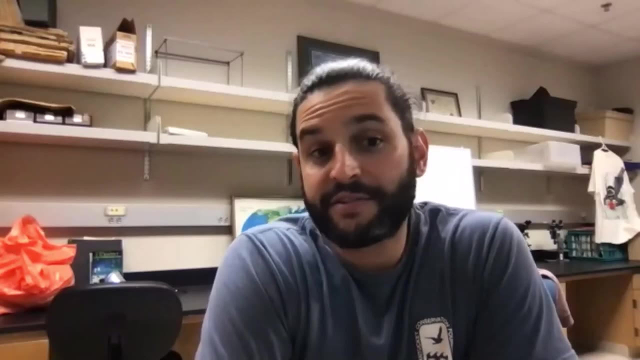 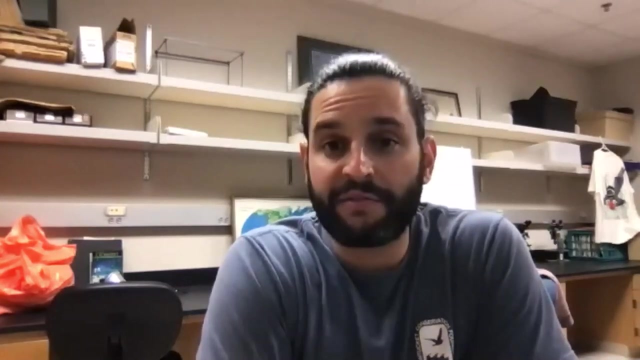 infauna behave similarly when crabs are excluded. That's from Eugene Gallagher. That's a really cool question, Eugene. The short answer is: we don't know. This is definitely something that is on the mind of researchers. It might even be on Michael's mind. 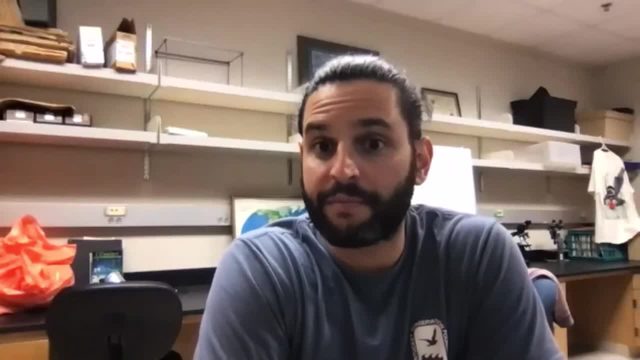 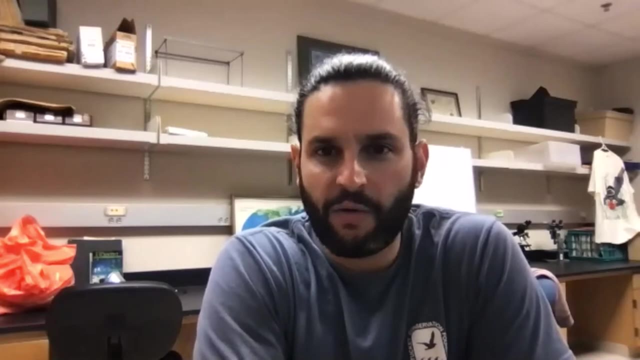 because as blue crabs move, you know, further up north, this is going to be something that that needs to be studied. So, you know, I'm not sure of, maybe, the current status on this, but when I was like doing this- the projects- Nantucket was one of the only sites that I went. 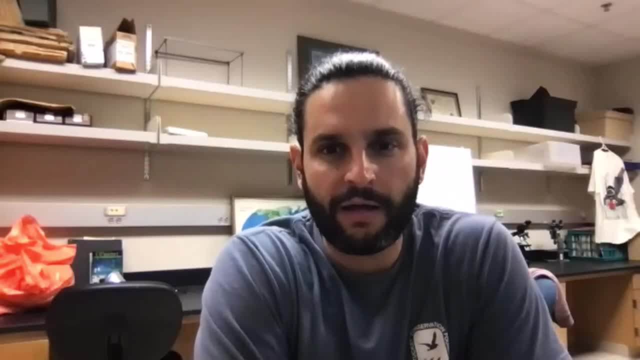 to that, even got blue crabs, I think maybe we got some on the Cape as well, but definitely not. I don't remember seeing very many north of the Cape. I think that maybe has changed over time and maybe Michael and I can talk about this in the 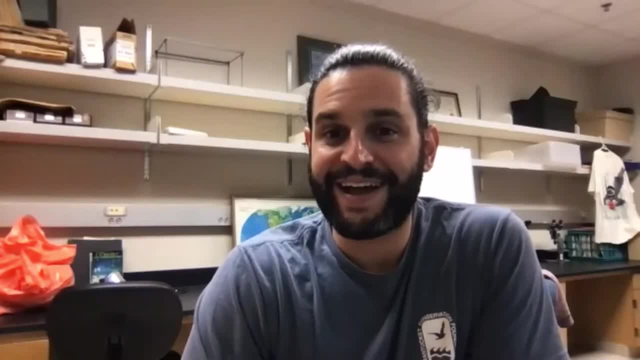 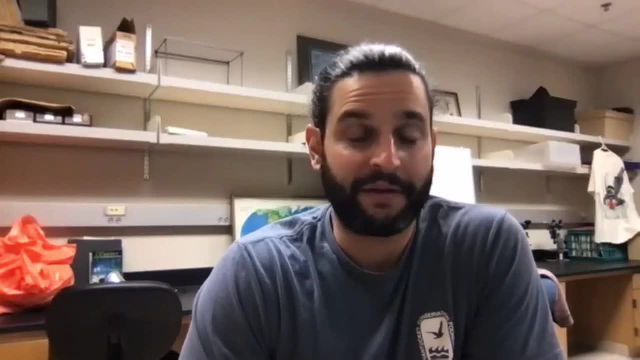 in the panel: potentially, but the direct answer is we don't know yet, but very, very likely. Yeah, blue crab impacts as because they're- I mean probably, you know they're extremely important, if not the most important predator as you go up the coast. That's gonna be something that's. 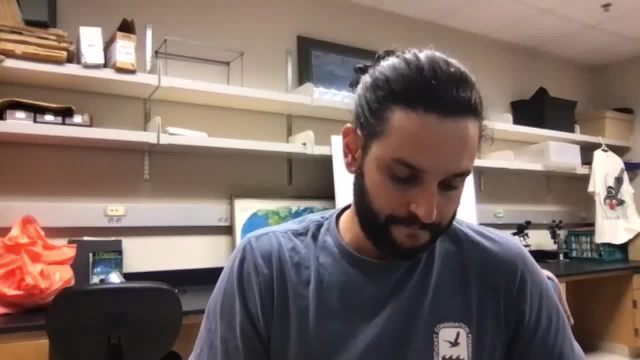 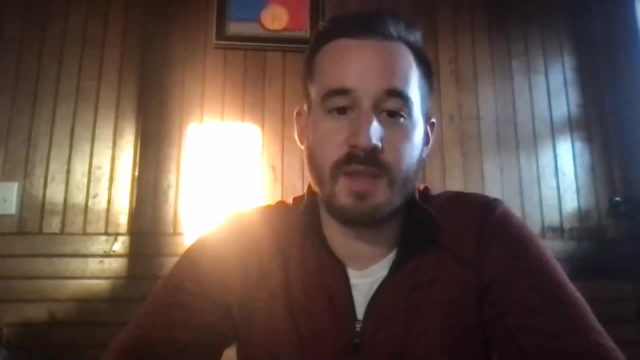 really interesting for the future of New England marshes. Awesome thanks, Mark. We'll just do one more question before we turn it over to Mike for a presentation. Just a reminder for folks. there will be time for more questions later. So Heather is asking: did you observe? 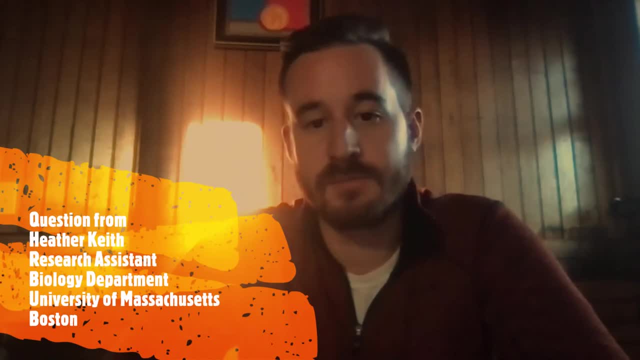 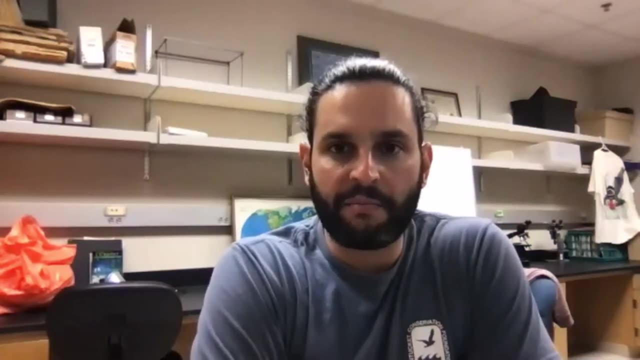 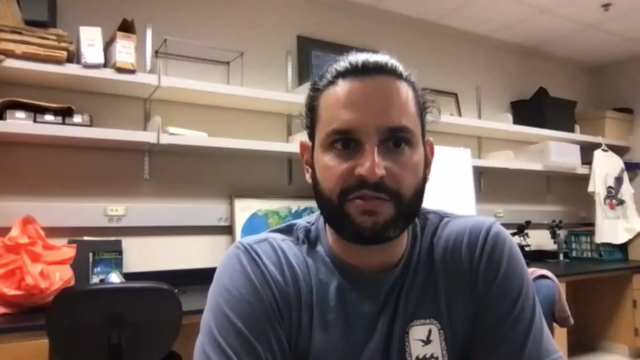 overpopulation of other species when you excluded predators? Good question, Heather. You know we didn't observe any like overpopulation. you know big, big booms really. but there were a couple of interesting findings sort of related to that. 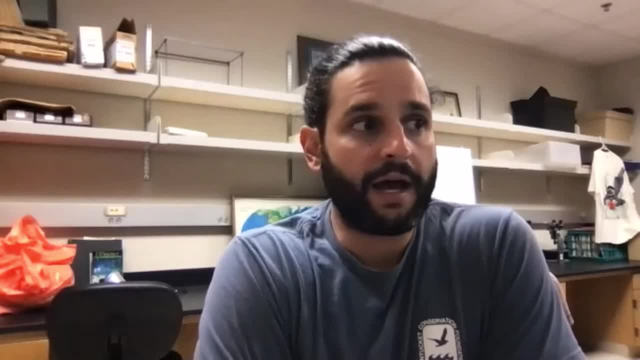 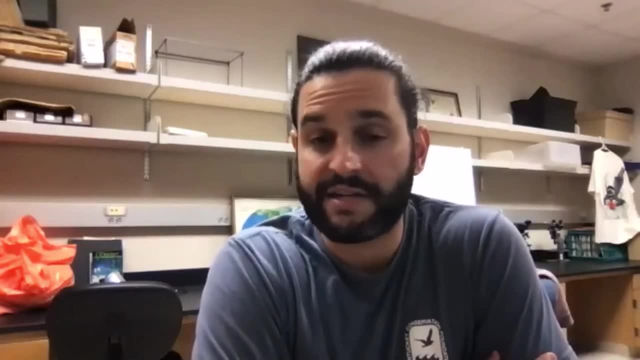 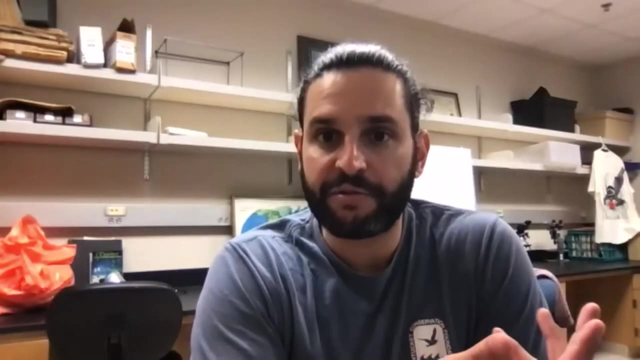 So in Folgers Marsh, in just sort of like as you as you walk along the marsh, no, no exclusions or nothing. you, at least when I was working there, you very rarely see any any. But as soon as I started to exclude marine predators, I noticed that these snails were recruiting into those plots. 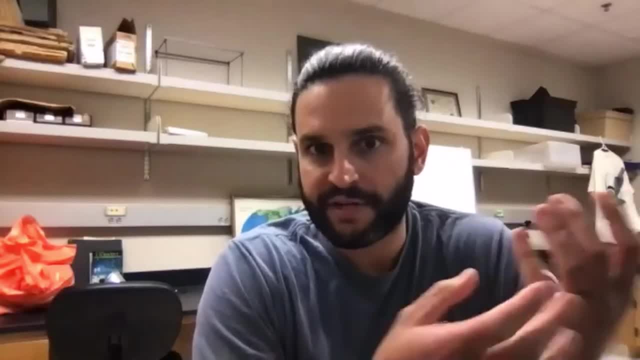 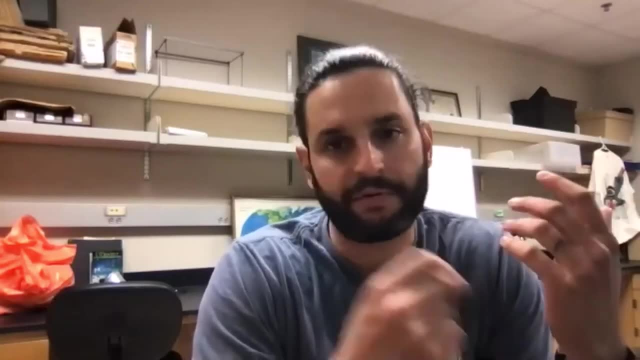 So this was a really interesting finding for me, because this meant that basically as soon as the snails were recruiting in these areas but they get eaten up like right away, either by little crabs or by mummy chugs who just take a mouthful of snail very easily. 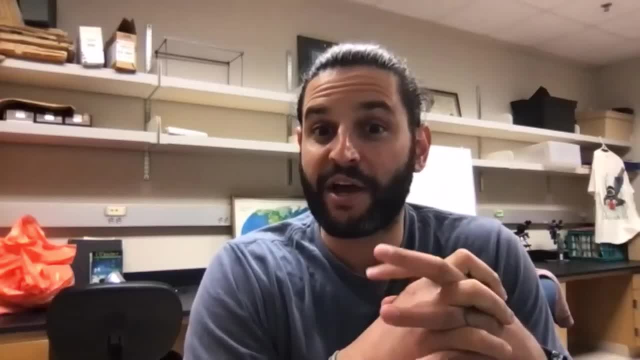 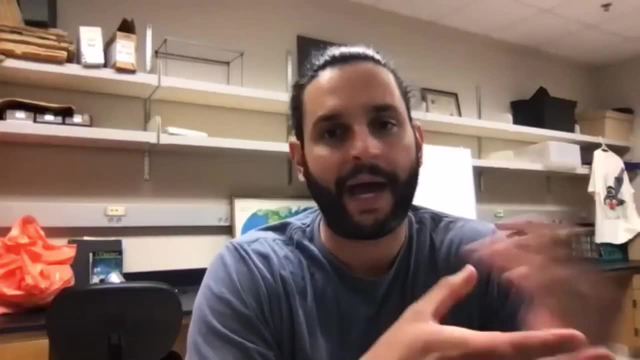 So you know, I think potentially, if things were to go like over time or multiple seasons, there potentially could be a buildup of of snails, maybe even of purple marsh crabs as well, But I didn't observe any of that in my experience. 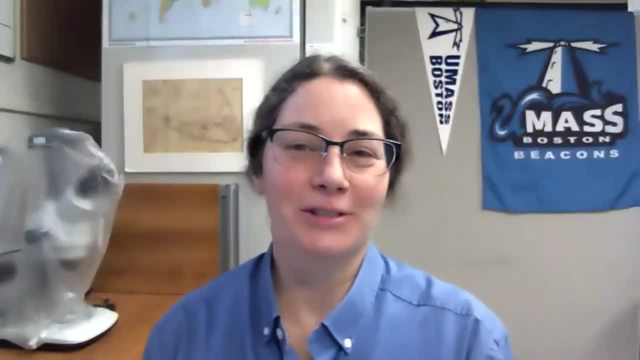 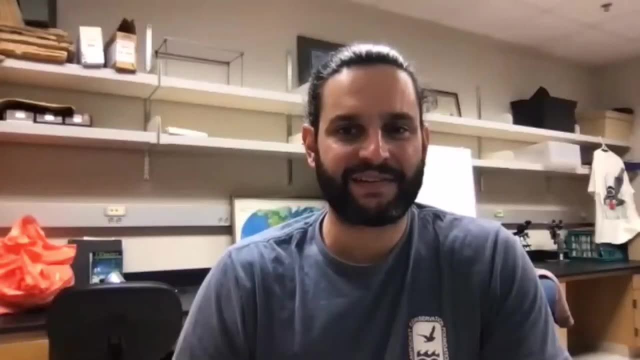 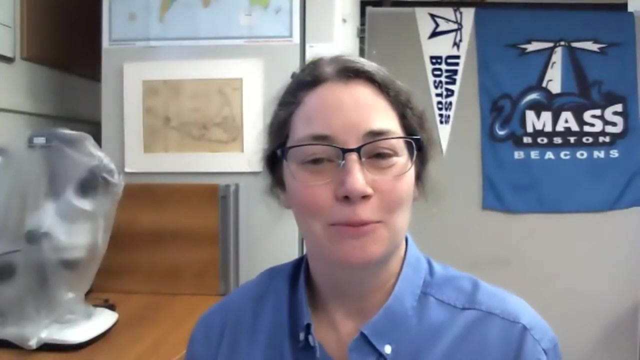 Thanks, Mark. This is so interesting. We could keep asking you questions, but we're going to pause that. So, for those of you who have more questions, write them down. But we're going to now hear from Michael Roy and it's my pleasure to introduce him. Normally we would be seeing Michael down here on Nantucket. 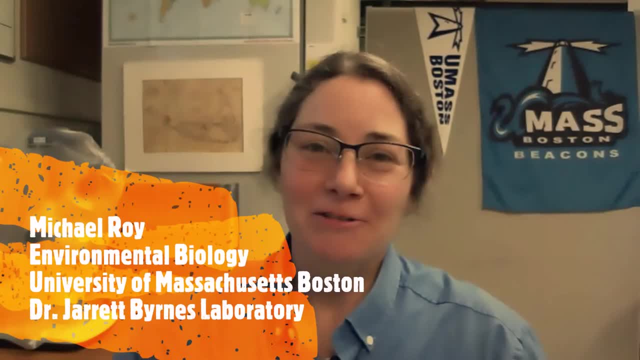 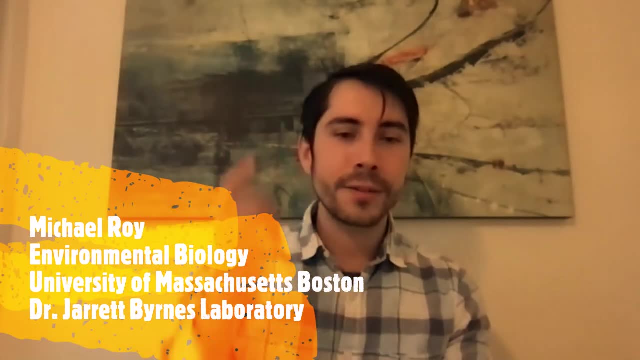 But tell us about your research. Thank you so much for that introduction, Yvonne, and excellent talk, Mark. I wanted to mention that on the blue crab front we actually- so I've done a fair amount of work in Plum Island. 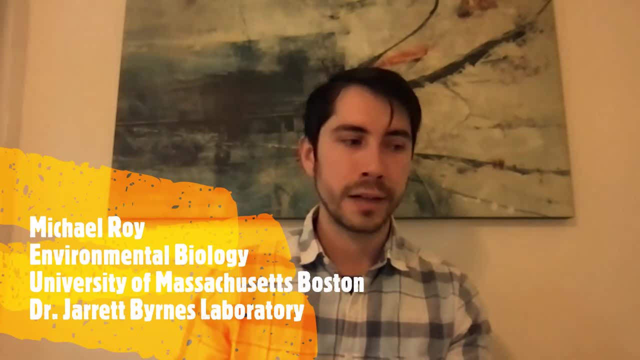 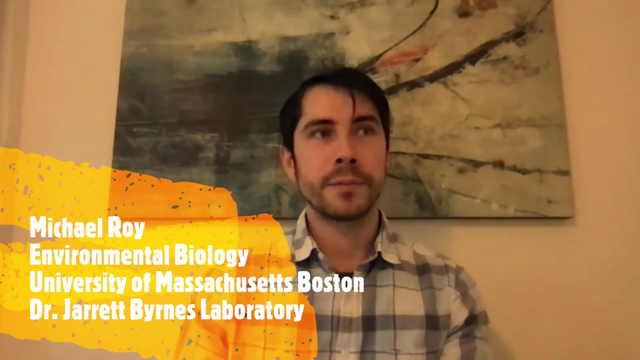 which I'm going to talk about a little bit today as well, But we saw five blue crabs. They were up in Plum Island this summer, which was which was really wild to see. So they're, they're coming up and it'll be interesting to see how, you know, their presence is really going to impact. you know food webs. you know up in, up in Pai. 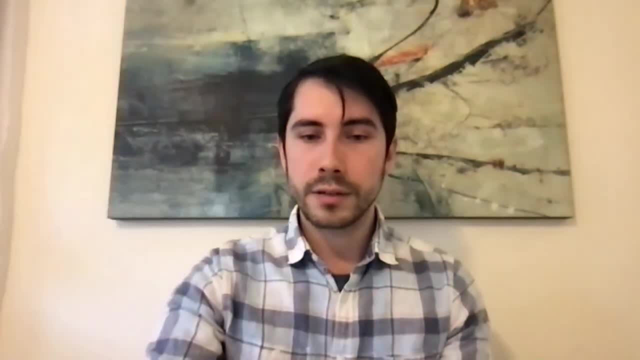 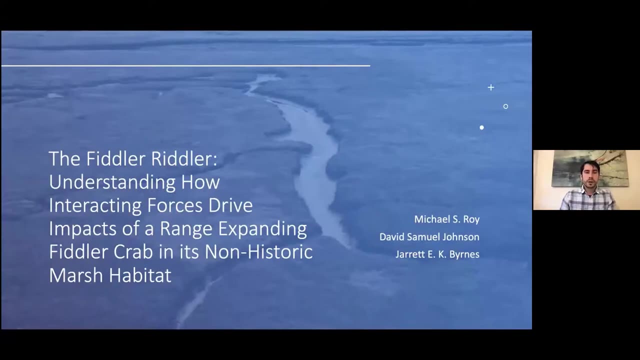 So All right. So I'm going to go ahead and start sharing the screen, All right? Thank you so much, everyone, for coming to our talks. I just want to start by highlighting my two collaborators, David Dr. David Samuel Johnson, who is also at the Virginia Institute of Marine Science. 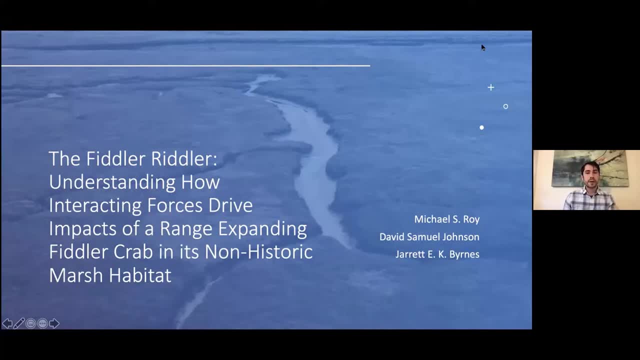 He started and pioneered a lot of the work that that I'm working on currently. He is the first person to find the fiddler crab that I'm going to be talking about in in Plum Island. And, of course, I want to talk about my adviser, Dr. 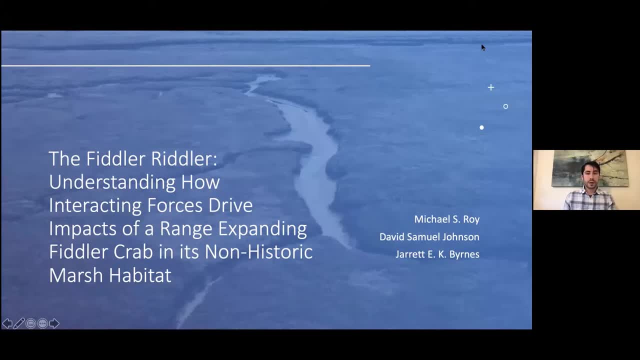 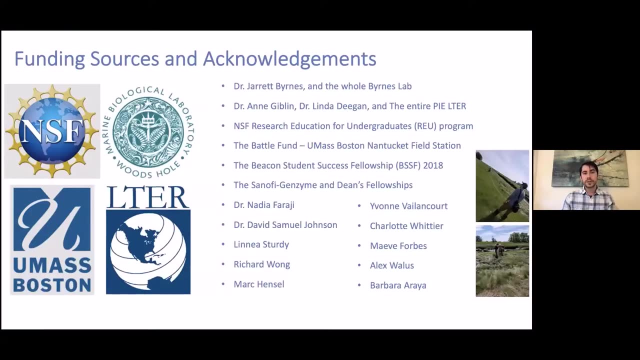 Jarrett Burns who's advising this. This project would not be possible, And I also want to Bring up, first and foremost, my funding sources and acknowledgments: a whole series of people that have really helped with this research, A number of undergraduates research funding through NSF, the Battle Fund at UMass Boston, UMass Boston itself and some internal grants at UMass Boston. 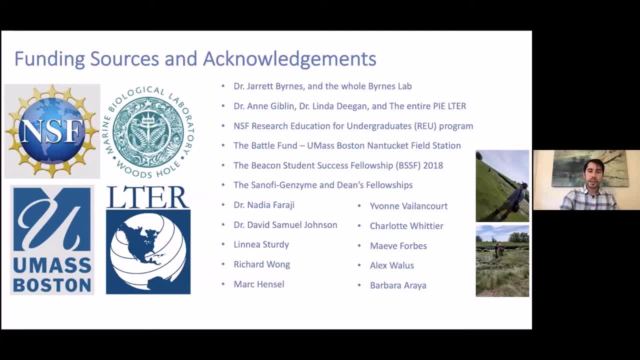 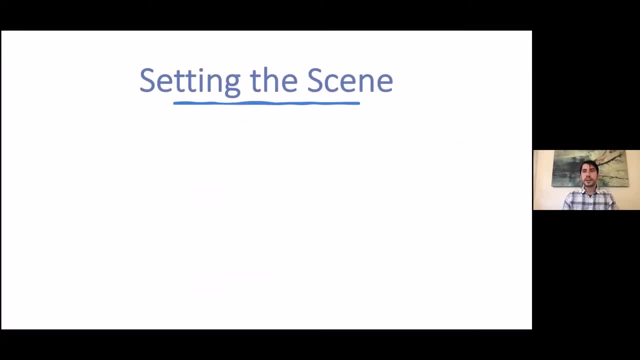 So with that, I'm going to get started on talking about really the work that I started in 2017.. And sort of have worked on throughout, throughout my dissertation, And it's really sort of an ecological story that I'm going to be talking about. with any ecological story, with any story. 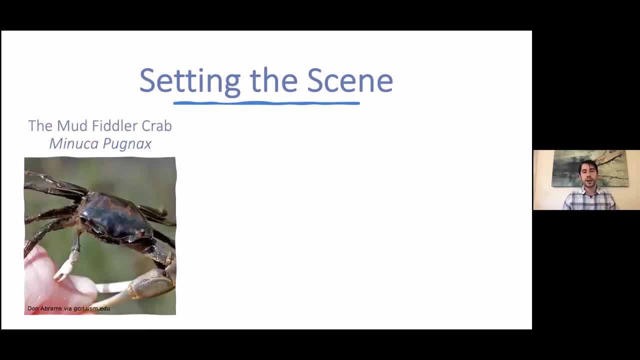 I want to set the scene, So first I'm going to talk about the star of the show, The fiddler crab, Manuka pugnax. This is a mud fiddler crab is a burrowing species of crab that is native to Nantucket. 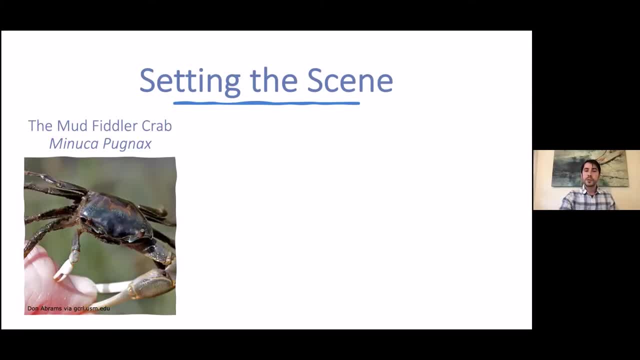 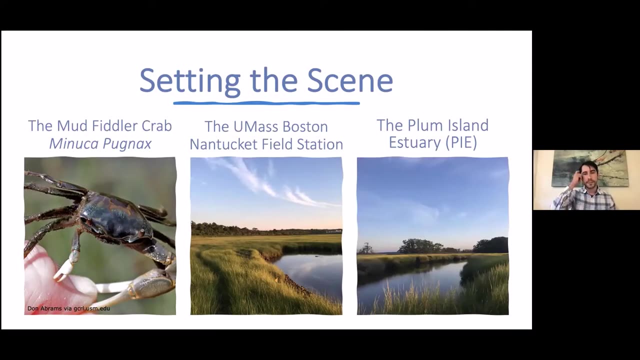 All the way down to Florida and is a really critical species. And the two places that, the two scenes, the two locations that I'm going to be talking about are the UMass Boston Nantucket Field Station, specifically Folgers Marsh at the UMass Boston Field Station, and the Plum Island estuary, specifically sites at the long term ecological research site there. 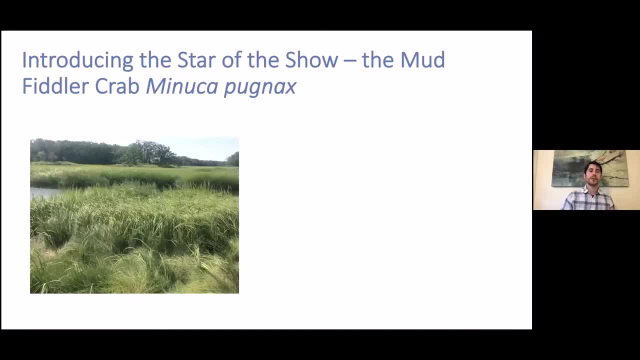 Okay, so let me introduce you to the star of the show, the mud fiddler crab Manuka pugnax. So the image on the left. you'll notice it's a very lush green spot. This is the low marsh of 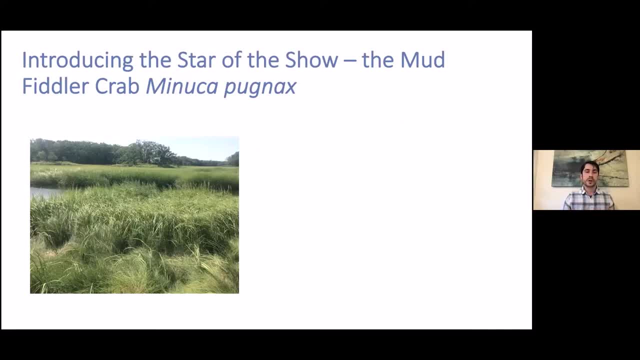 A typical salt marsh. this is where the tallest for China alternate flora grows. It's right next to creeks and part of the reason why it grows so tall is because it's the first grass that's going to encounter all of the nutrients that come in on every. tide, And so this is the spot where the fiddler crab, Manuka pugnax, lives. And where does it live? well, it burrows into the sediment- around this part- I know alternate flora, so it digs these deep holes, Roughly 15 to 20 feet deep. 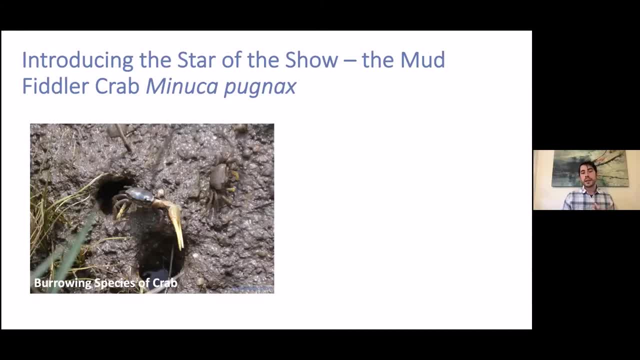 So it digs these deep holes roughly 15 to 20 feet deep. So it's a really dynamic species because it potentially has ramifications for interacting with soil microbial activity and water saturation. because it's basically Swiss cheese in the marsh, You'll notice here that the male fiddler crab is front and center. 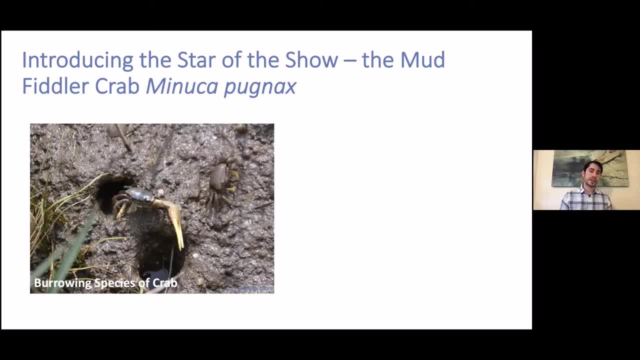 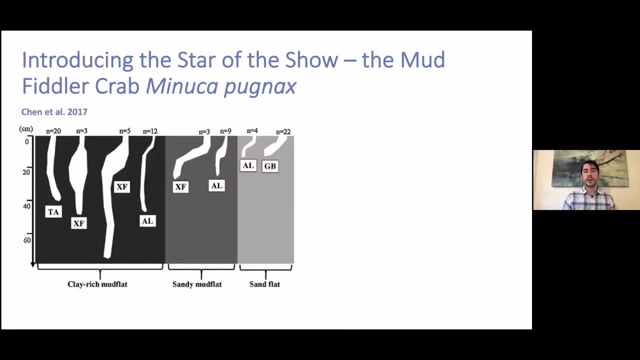 He is characterized by that large claw that looks like he's holding a violin, like a fiddle, and then the female, a female fiddler crab, is to the right of that in this image, And so, And so these burrows are really dependent on the kinds of sediment that they're burrowing into. 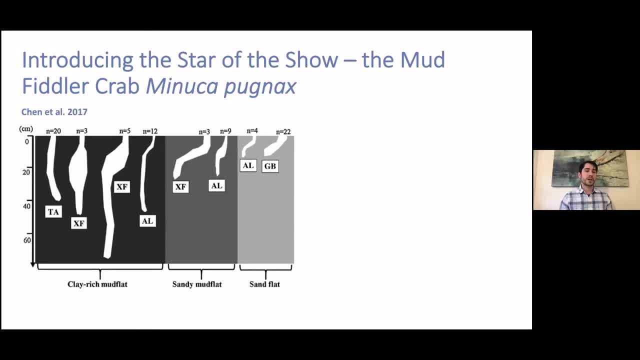 Not all salt marshes are created equal. Some salt marshes are going to be clay rich or so more peaty, some are going to be a little bit sort of a mix of the two, that are sandy, and some are going to be more of like sand flats, And this image from Chen et al highlights fiddler crab. 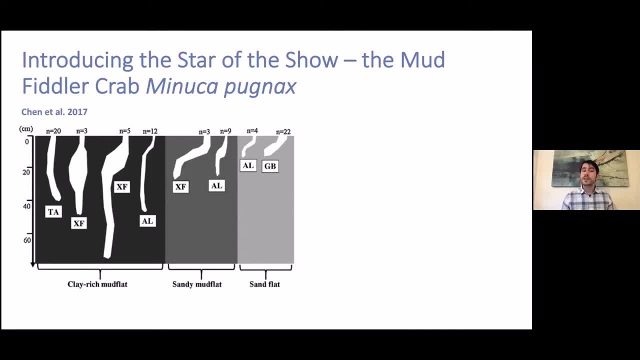 species that are not the mud fiddler crab, but they behave similarly in terms of their burrowing behavior, And so you'll notice that the clay rich mud flat fiddler crabs are able to burrow deeper, they're able to have wider burrows, and part of the reason for that is because 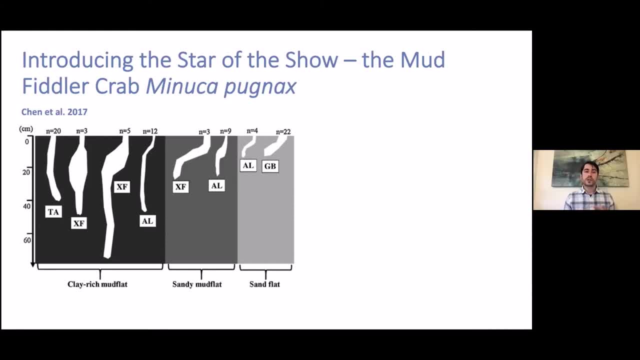 the clay rich mud flat has a little bit more structural integrity to maintain those burrows, and fiddler crabs don't necessarily have to spend as much energy maintaining those burrows once they're made. And then, as you'll notice that as you go towards sand flats, 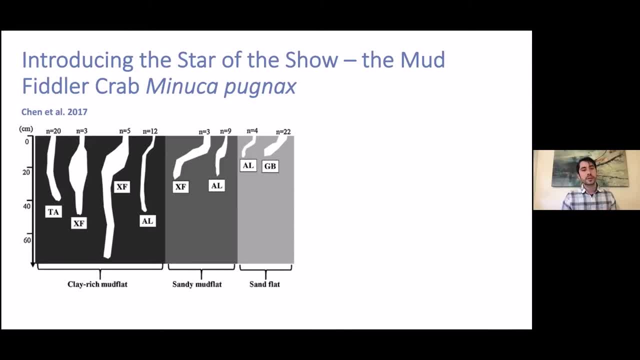 they're a little bit shallower and then not quite as wide, And so this is really important to take into consideration for the rest of the talk, as well as just thinking about how fiddler crabs interact with their environment, And what's really important to understand is that 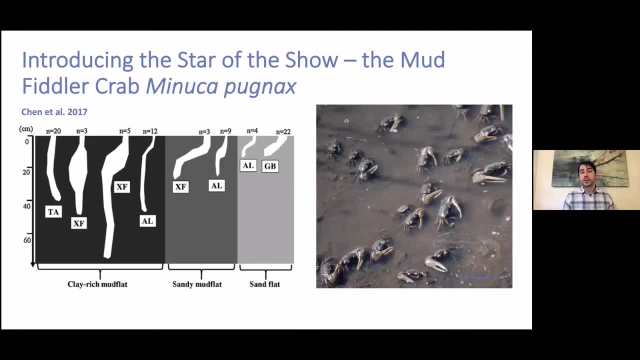 fiddler crab densities can get pretty high, so they're really creating a lot of burrows into the sediment. They can get up upwards of 150 individuals in some southern salt marshes in Nantucket between 80 and 100, and then even more, And so they are a really critical species for 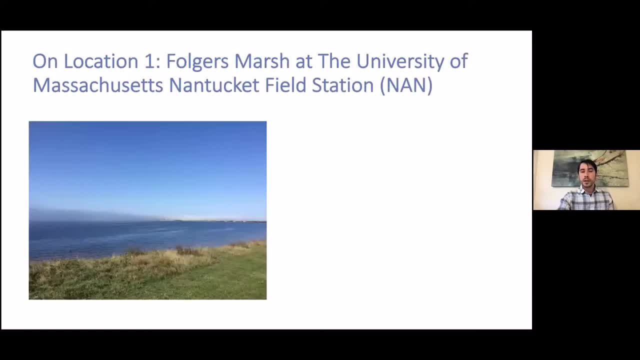 interacting with this environment. So let me talk about the Folgers Marsh and the University of Massachusetts Nantucket Field Station where this work was done. So, as Mark mentioned, it's an incredible place to do research. This is looking out over the bluff with the bunkhouse. 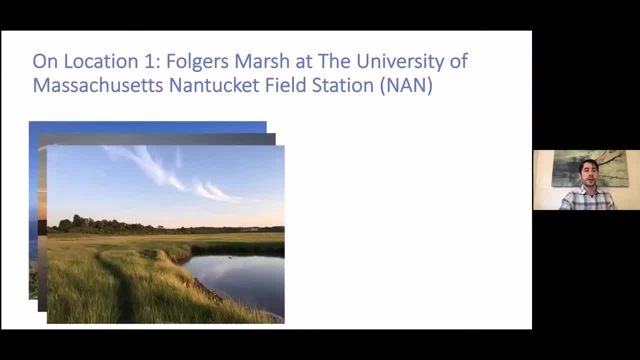 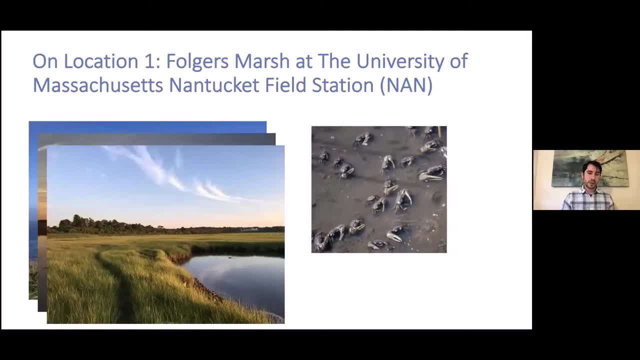 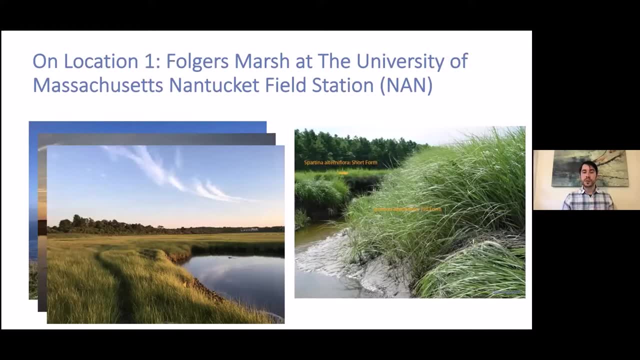 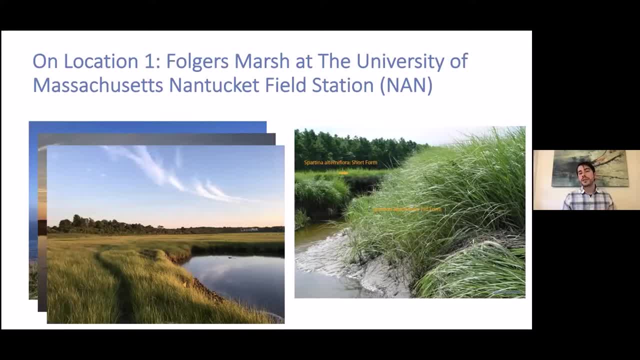 But in southern salt marshes- what I mean by that is salt marshes south of Cape Cod- they're predominantly dominated by this species of grass. North of Cape Cod, they're dominated by another species of grass, Spartina patens, which I'm going to talk about on the next slide. 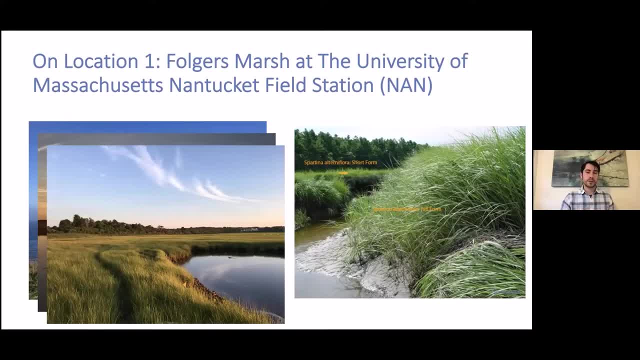 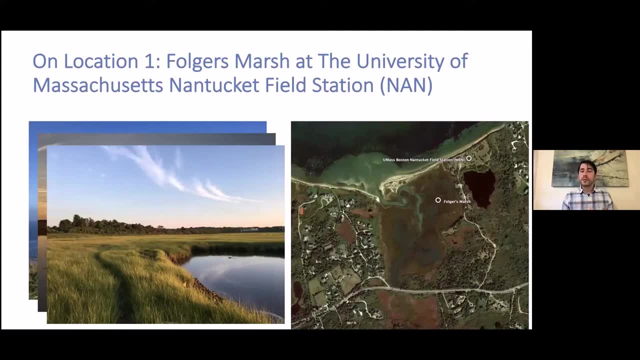 But it's just critical to keep that in mind in terms of differences between different sites. The last thing that I want to talk about for Folger's marsh is that there are a lot of oceanic inputs of sediment, So every tide sediment gets flushed into the marsh. 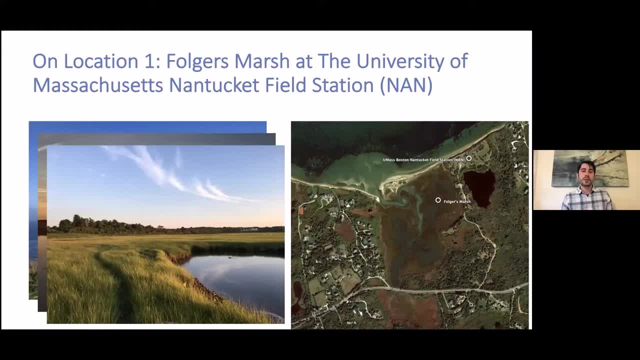 And that's, by and large, how the marsh builds up, both vertically as well as horizontally, And so it's really how the marsh grows or maintains itself over time. And because it's oceanic, there's a lot of silt, there's a lot of sand. 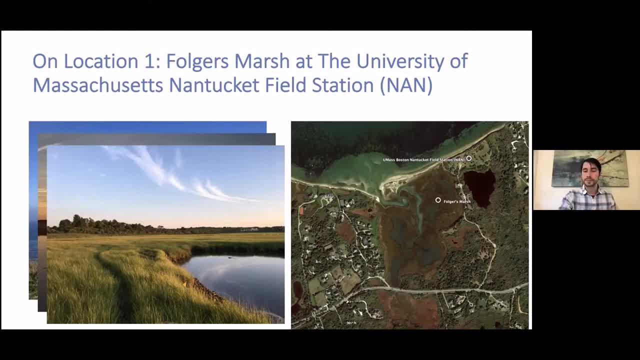 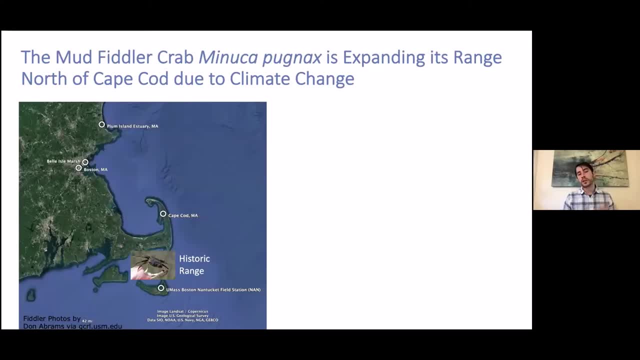 So it's a little bit more of a sandy and silty salt marsh. So this is where fiddler crabs live. That's their historic range. Fiddler crabs, as I mentioned, have a range all the way down to Florida. 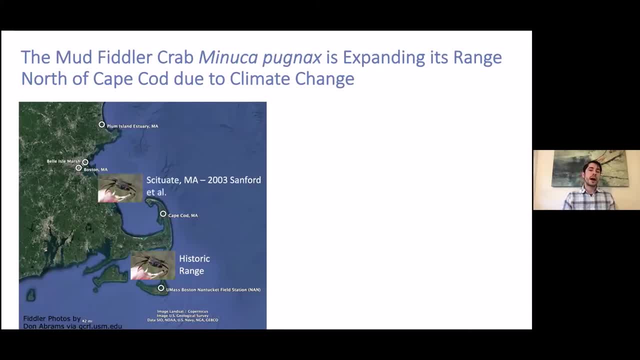 But what was really interesting is that in 2003,, Mark Sanford et al found individuals of mud fiddler crab for the first time ever in their life history in situate Massachusetts in 2003.. Then, as I mentioned, David Johnson and other colleagues at the PIE LTER, but primarily David, 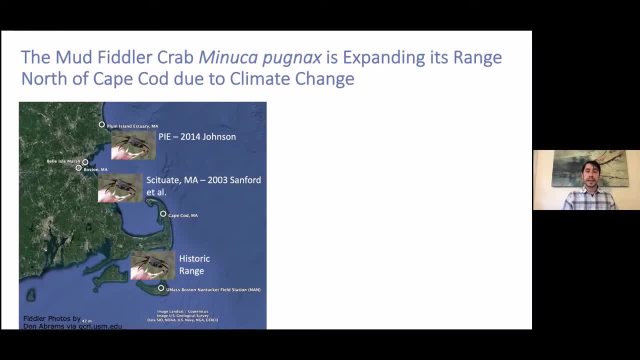 found individuals in 2014 up in PIE, And so this is the first ever occurrence in northern New England salt marshes. They're now found as far north as southern Maine, So their distribution is really expanding. So the question is: why is their distribution expanding? 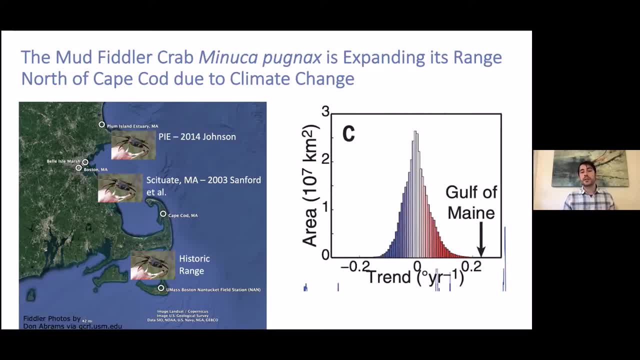 Well, a big piece of that is likely due to the fact that the Gulf of Maine is warming at a rate that's faster than 99% of the global ocean. So you can really see here that the Gulf of Maine is highlighted in sort of the red colors. 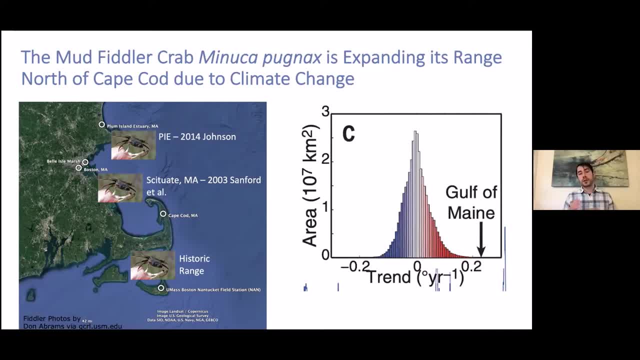 here, which is the more extreme habitats that are experiencing warming. Part of the reason for that is because, due to the oceanic offshore shelves, as well as other morphological features, the Gulf of Maine sort of acts as this large bathtub of water recirculates. It's still colder than It's going to be difficult to predict how fiddler crabs will interact- And they're new sort of expanded habitat- than potentially how they're interacting in Nantucket. So that leads me to my two research questions, which is: to what extent does this fiddler crab impact ecosystem functioning? And the three ecosystem functions that we looked at for this study were soil strength, primary production and decomposition in its historic range, which is Nantucket, versus its expanded range in Plum Island. And then the second question is: does the density of fiddler crabs influence any of these impacts that the fiddler crab has on these ecosystems? So to answer these questions, we set up a series of fiddler crab inclusion cages. And so we put in different densities of fiddler crabs, ranging from no crabs, which is demonstrated by the box, all the way to the left, which is 0. Then there is 20 crabs, which demonstrates ambient density. And this is crabs per school And this is crabs per quarter square meter, which is about ambient in Nantucket. So we replicated this four times in both locations, so 24 total cages per site. We ran this experiment from June to September in 2017 and 2018.. We measured a whole different suite of environmental indicators for these ecosystem functions. I'm not going to go through this laundry list, but what I do want to highlight is the map and the metric at the bottom, which is decomposition In order to measure decomposition. we took Spartina alterniflora, we dried it, we put it in these mesh bags and then we buried it 5 centimeters below the surface of the soil and 15 centimeters below the surface of the soil. And the reason for that is because we wanted to determine decomposition rates of these two different depths, because depth makes a big difference in terms of decomposition rates. And so, before going into sort of the how we took all of this environmental data and really tried to derive inference for how fiddler crabs were really, structuring these ecosystems, how they were really sort of driving ecosystem functioning. I want to go into actually what these cages looked like. So it was pretty straightforward. It was just four PVC pipes with mesh around them buried into the sediment to prevent crabs. 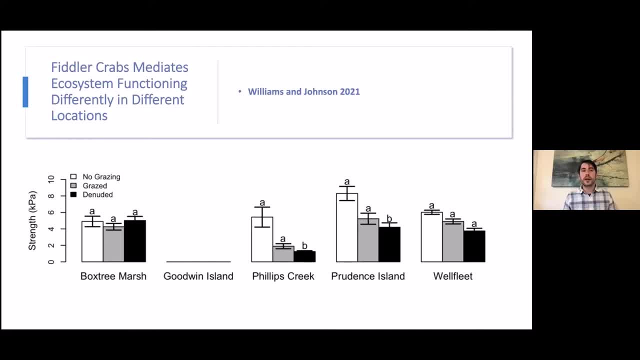 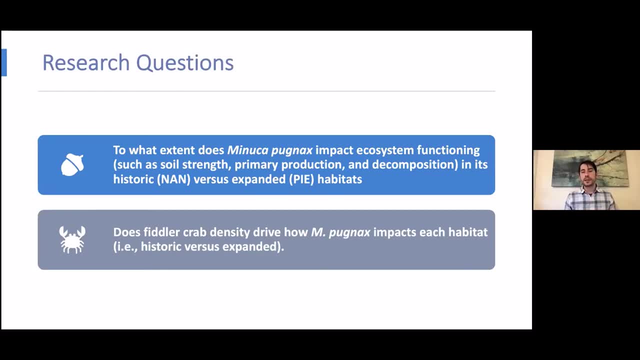 from burrowing underneath, And then we put steel flashing at the top to prevent crabs from either crawling out or for new crabs to crawl in to really control for that density. So, as I mentioned, we have all of these environmental indicators: soil strength, primary production, 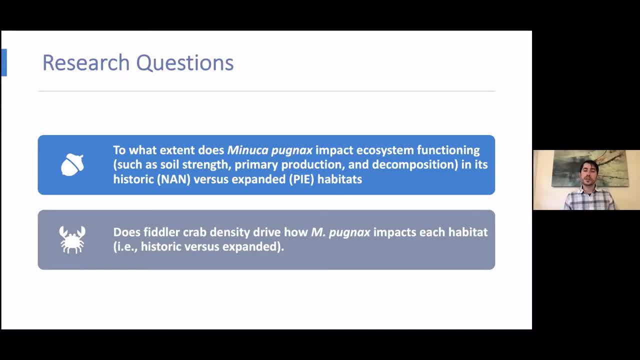 biomass of Spartina alterniflora, And so, given the fact that we have all of these different environmental indicators, we really wanted to tease apart what's really driving this system, And one methodology that is used quite often is using causal models and structural equation modeling. 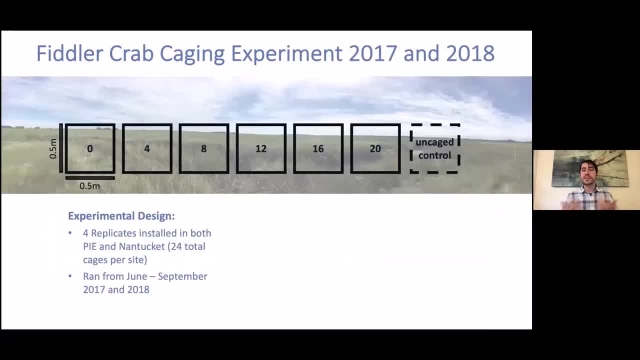 So I'm going to walk you through this. So we, every step of the way, there's an exercise in the Bay Area strategy for using lots of causal models, or ali- cerca analysis and qualitative analysis to really sort of understand how these species are interacting with this ecosystem. now 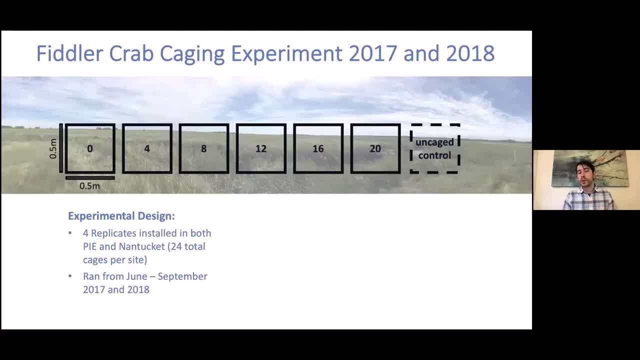 This framework works. So it's very straightforward: a change in c and then you can also have a causing a change in c as well. so really sort of qualitatively gets the researcher understanding about how their system is working, how they believe their system is working, and to test this quantitatively you can use what's- what's. 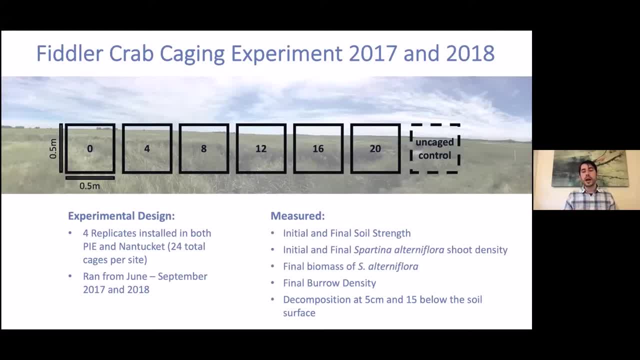 called structural equation modeling or sem. and structural equation modeling takes this causal model and it applies statistics to it to get statistical outputs to determine how likely this, uh, this um causal model represents the world, represents reality, and it gives you statistical outputs to determine, you know, if it is representing reality, what's actually driving. 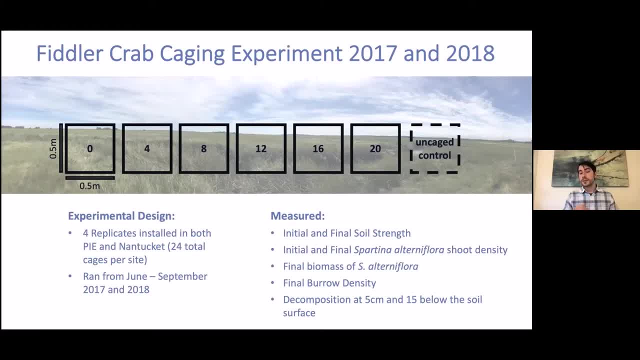 what variables are driving change? what is the causal relationship here? okay, so with that in the back of your mind, i'm going to jump into into my results, um. so, uh, the results i'm going to show you, um, are a mix between both the uh structural equation and the c, and you know the c equation, but i'm not going to get into the detail of all that. 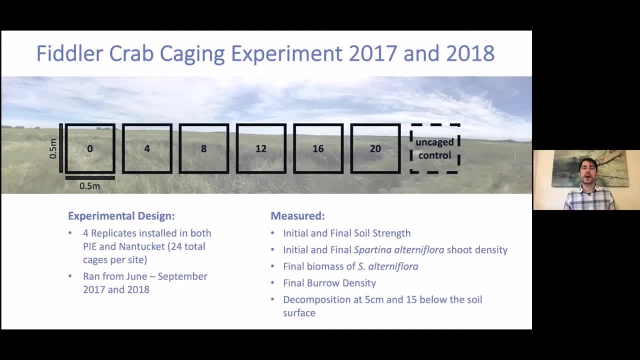 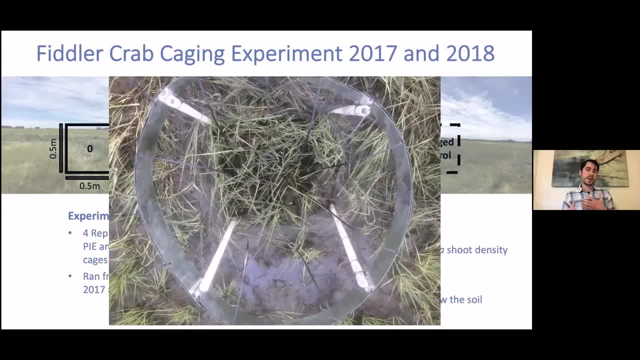 models that we, that we developed, as well as some heat maps that show some of the interactions that we, that we found, and so on the left, you'll see that we have crab density, which is just the number of crabs per plot and that we manipulated. those are the crabs that we put into each cage and we 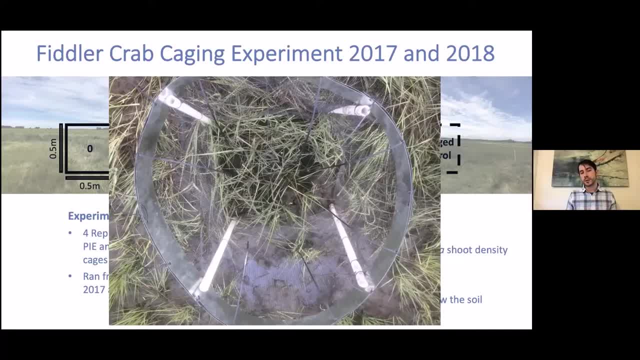 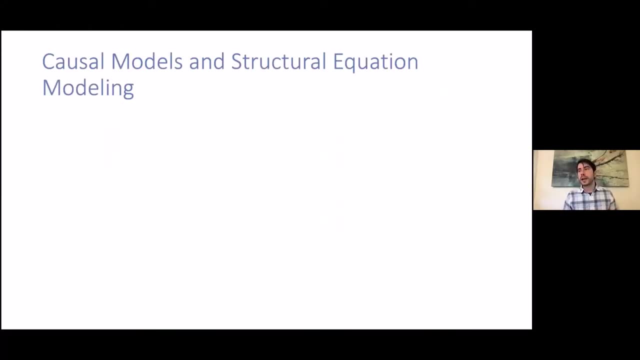 have initial soil strength, which is just the soil strength that we measured at the beginning of the experiment, without manipulating anything, and this was measured within each plot. and so then we wanted to determine: does crab density and or initial soil strength affect the number of burrows at the end of the experiment? and this is important because it's it is that burrow burrowing behavior. 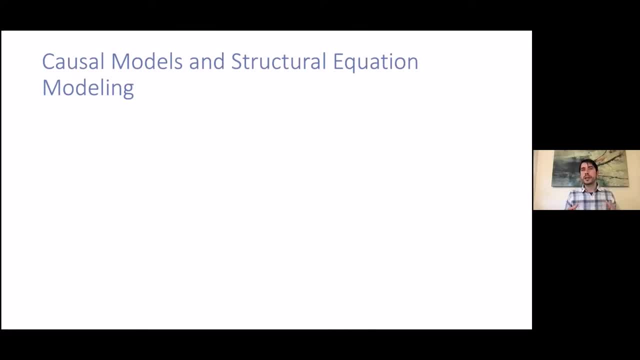 that's going to be driving whether or not the fiddler crab is going to be interacting with their with with the ecosystem in some way in either Plum Island or in Nantucket. and so what we found is that the gray, the thin gray arrows indicate a non-significant relationship, that crab density. 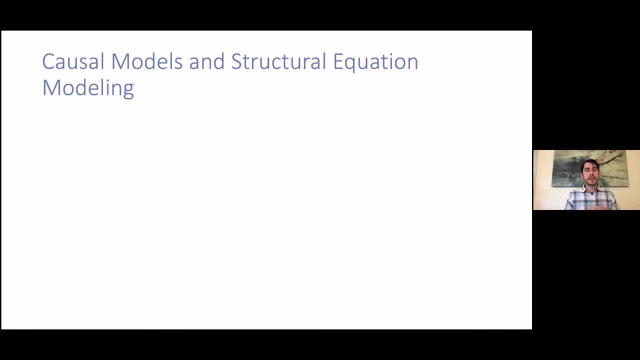 by itself, and initial soil strength by itself does not cause a change in burrow density. it doesn't matter how many crabs you have. burrows are irrespective of that, except when taking into consideration the interaction between the two. so as you so, essentially, as you increase the number of crabs, 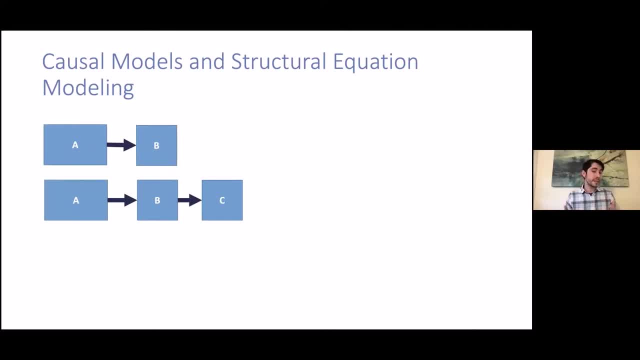 you also have to increase the amount of the, the strength of the soil, in order to increase the number of burrows, and so it goes back to that figure that I showed before, which is that that PD marsh is going to, you know, really be facilitating the ability for crabs to maintain these burrows. 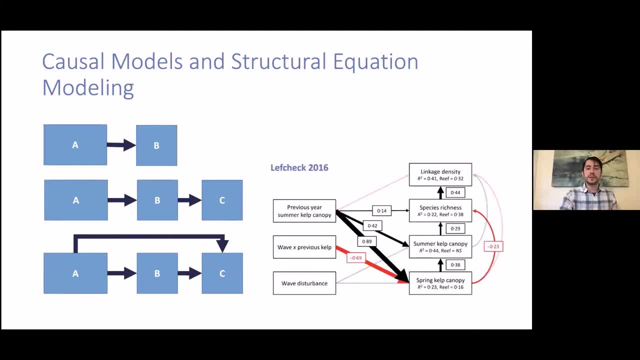 and to increase burrow density over time. so this is all well and good, but this doesn't really talk about the actual ecosystem serve or ecosystem function, which is soil strength. so does burrow density actually confer something about soil strength? and the answer is yes. so so the thick. 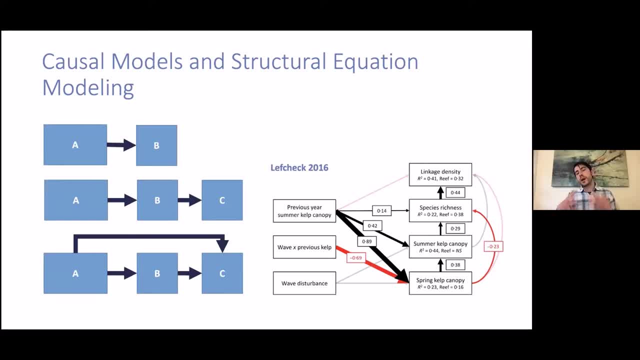 blue line indicates that there's a significant causal relationship between burrow density and final soil strength, such that the burrow density is going to be increasing over time and as you increase the number of burrows, you are decreasing the structural integrity of the soil. 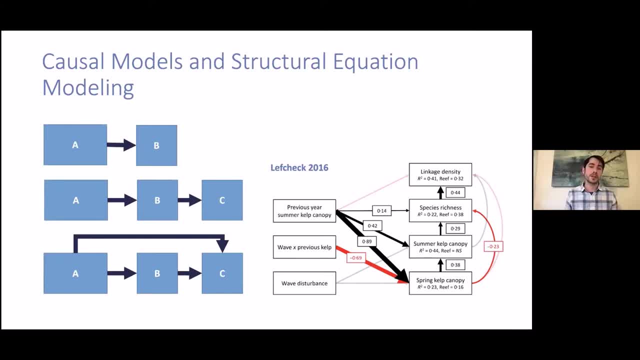 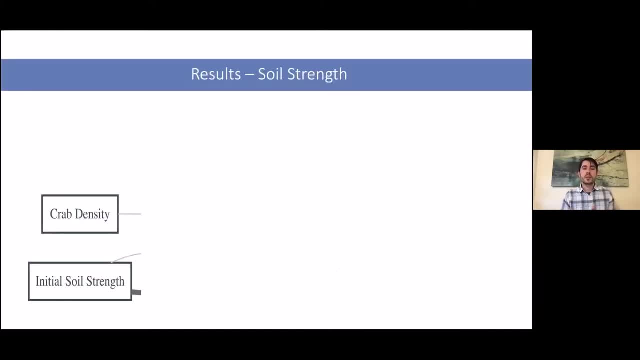 you're decreasing that compaction, which sort of from a first principles perspective doesn't isn't that big of a stretch, because when you think about all of that water saturating the sediment, you're sort of increasing the amount of water between sediment grains, So it sort of 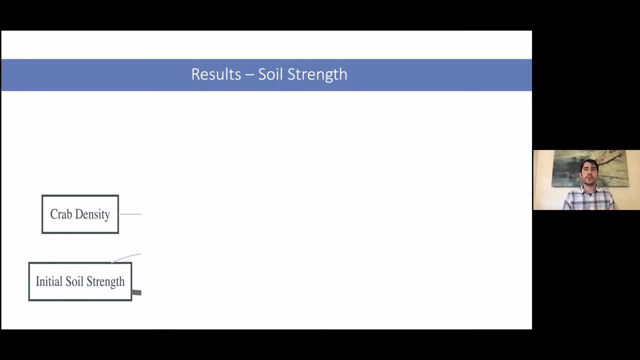 it makes sense that that might be the case. This final gray line just indicates that initial soil strength has a causal relationship with final soil strength, which is what we expected. So this crab density- soil strength interaction can be a little bit difficult to visualize. 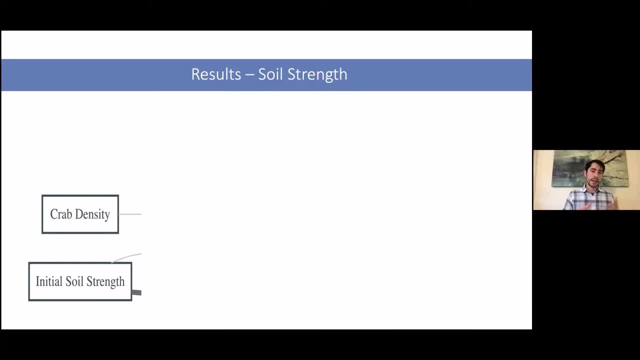 It was difficult for me to visualize at first, and so what we did was we plotted this in a heat map to really sort of try to understand how these three different variables are interacting with one another. So on the x-axis, down here, we have initial crab density, which is crabs per plot. 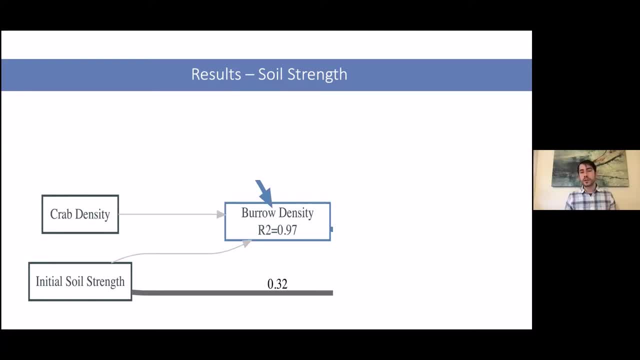 so again, that's just that metric of the crabs that we put into each cage. On the y-axis is this initial soil strength, which is again just that soil strength that we measured at the beginning of the experiment. and the different colors represent the number of burrows. So the redder 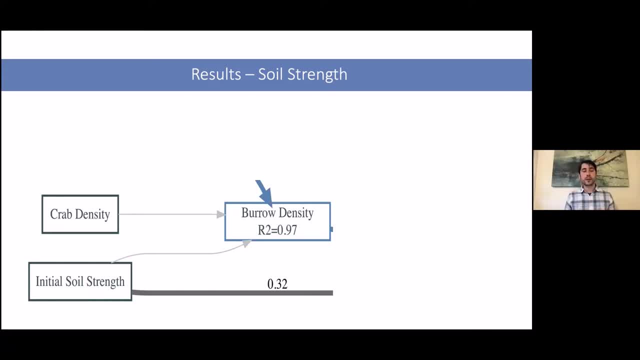 the color. the warmer the color the more burrows you have and the cooler the color the fewer burrows you have. This really highlights that in this upper right hand corner, as you increase the number of crabs and as you increase soil strength you have. 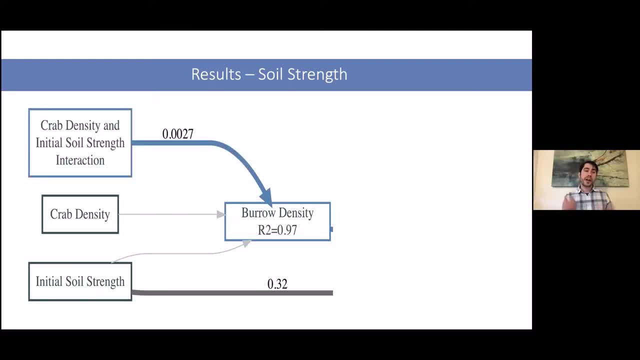 more burrows. This really highlights that interactive relationship and how fiddler crabs are really sort of, or how these environmental properties and population properties are really driving fiddler crab burrowing behavior. Okay, so what about the next ecosystem function, primary production. So I just want to mention that I threw sort of this model up. This is: 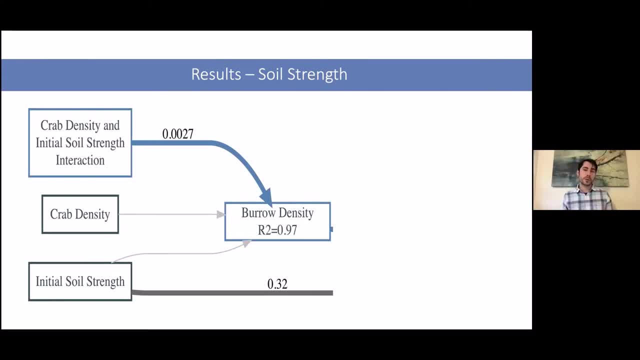 exactly the same model that I showed before. The thing that I want to highlight, though, is that what's really interesting is that fiddler crabs may be self-sustaining in terms of their their habitat. That as you increase the number of burrows, you're decreasing soil strength. 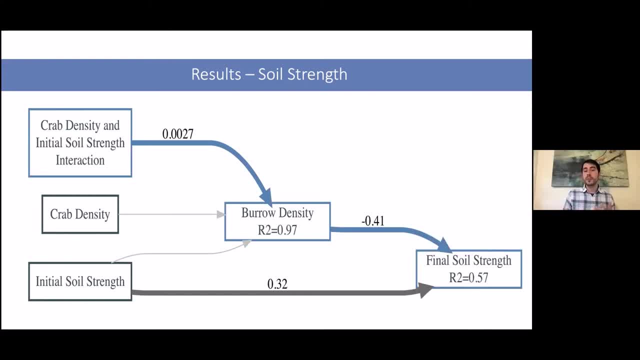 which is going to decrease the capacity for fiddler crabs to maintain their burrows. So it may actually be facilitating fiddler crabs and sustaining their own habitat. because there may be sort of this pulse where you have a really strong sediment, so a lot of burrows, but then 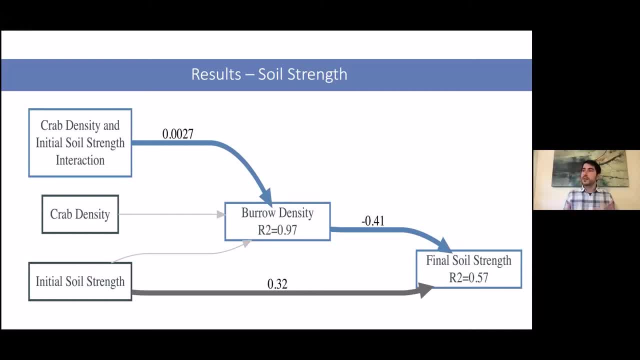 maybe the next year you're going to have a lot of burrows, and then maybe the next year you're going to have weaker sediment, and then so on and so forth. So I really sort of just want to highlight those dynamics before talking about primary production. So we measured primary 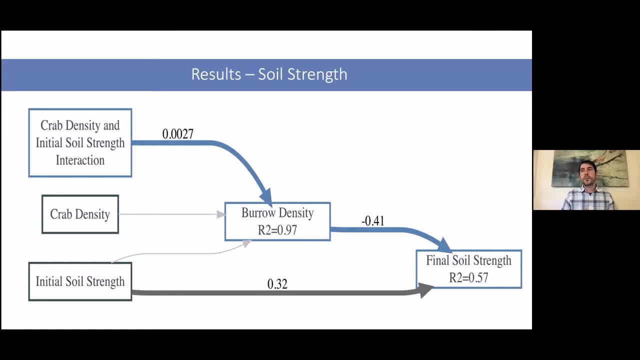 production, as both the amount of shoots in each plot as well as the biomass of the grass that we basically cut, dried and then weighed at the end of the experiment. So the Spartina biomass was not affected directly by any of the metrics from fiddler crab activity. 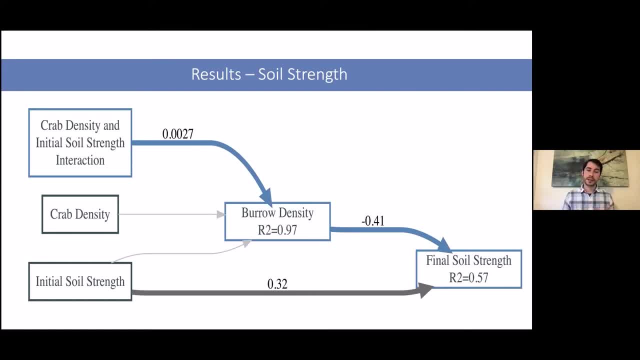 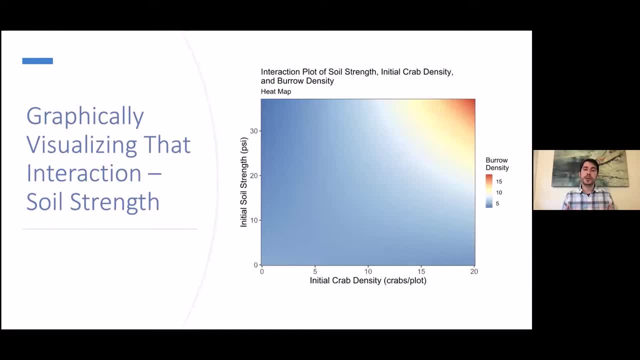 basically indicating, from this first approximation, that fiddler crabs do not affect the amount of Spartina alterniflora grass where they occur, Except again when talking about it from the perspective of an interaction. we found that there was an interaction between: 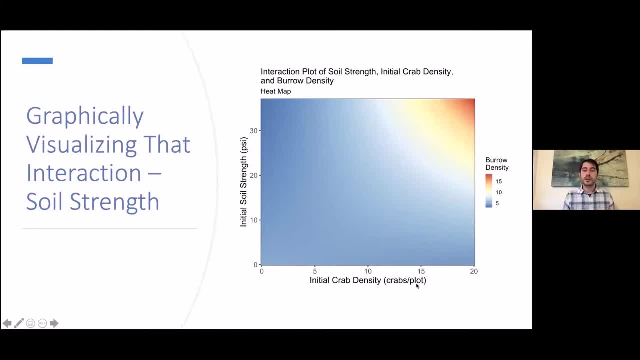 the soil strength when we collected this grass, as well as the shoot density when we collected this grass to weigh and dry. And so there is this indirect relationship where, if fiddler crabs are affecting soil strength, soil strength is not affected by the amount of grass that we collected. 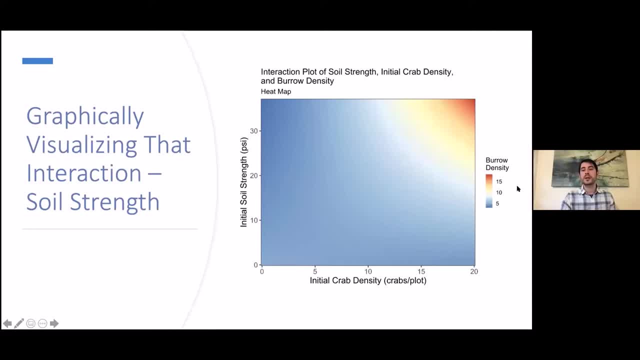 So soil strength will have an effect on Spartina biomass. So what does this interaction look like? Well, so there is another. we created another heat map that demonstrates this interaction. So in the x-axis is final shoot density, which is just shoots per quadrat, Final soil strength. 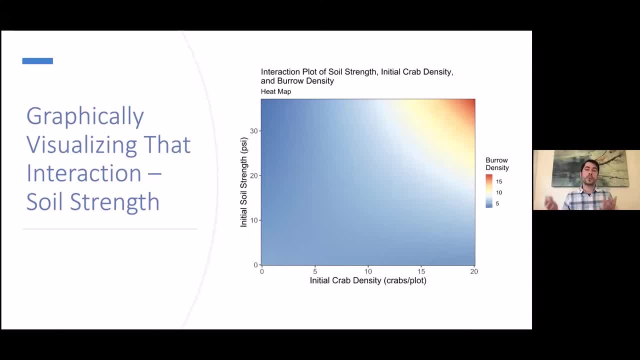 which is again measured in psi, And this time the warmer colors indicate more Spartina biomass and the cooler colors indicate less Spartina biomass. And what you'll notice here is that, on as you increase the amount of shoots and you decrease soil strength, you actually 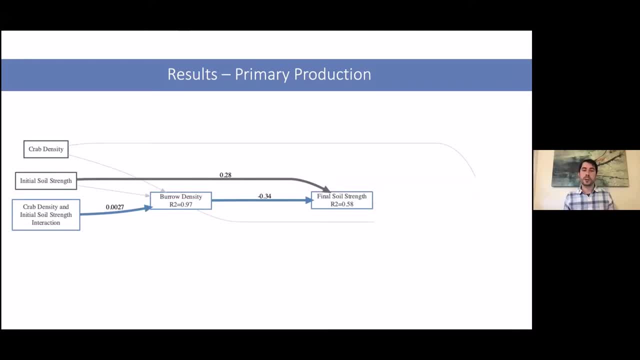 increase the amount of total biomass of the Spartina alterniflora, which basically indicates that Spartina likes to grow a lot of shoots but it doesn't like super, super tough sediment, And that's. you can imagine that being the case, because part of the reason, part of the way that 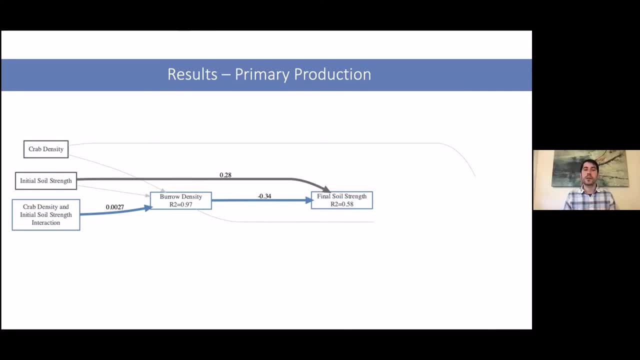 Spartina grows is creating rhizomes under the sediment and then shooting clones above through the sediment. And if it's really hard to grow, you know those, those rhizomes, it's going to be hard for the plant to grow shoots, And so in this instance, Fiddler crabs may be an indirect. 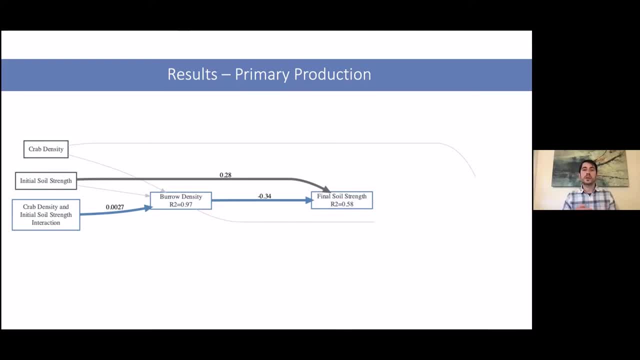 positive benefit to Spartina biomass via its weakening of the soil, at least at different timescales. Okay, So the final ecosystem function that we looked at was decomposition. And again, so this is more or less the same plot as before. I will highlight: 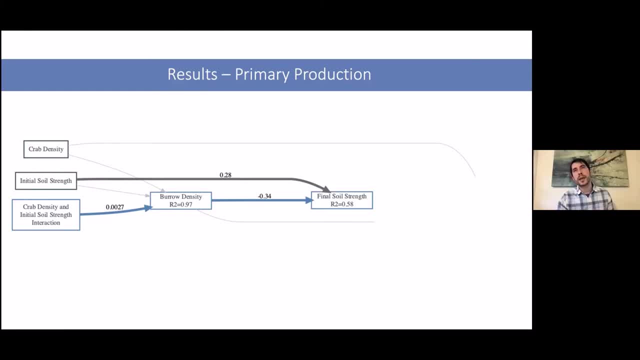 that this is only one year of of data. It was only in 2018.. We tried to collect this data in 2017.. The methodology that we used failed. We used tea bags. They disintegrated at the end of the. 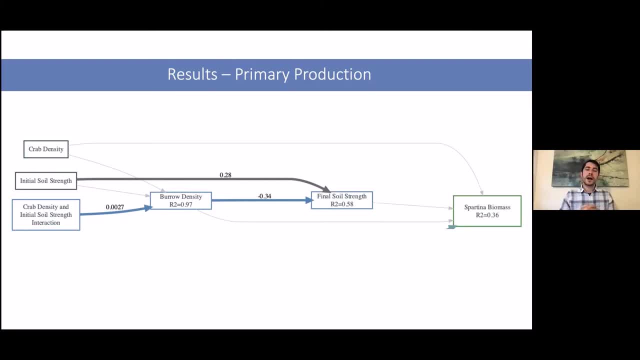 experiment. We used these litter bags instead these mesh bags, and that worked great, And so we do have data for this. So some of the causal relationships are going to be slightly skewed for the crab density, but we feel fairly confident in the relationships with decomposition, based on our 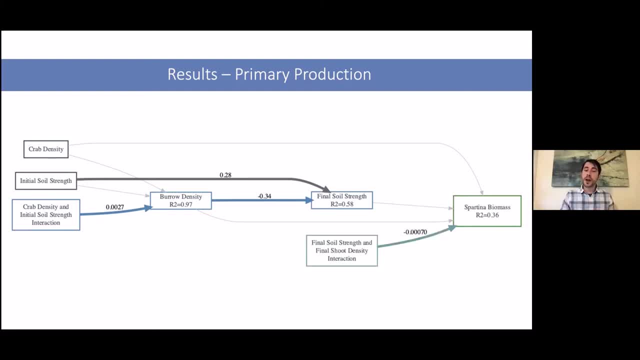 statistical outputs, And I can tell you that we have a lot of data for this, So we're going to talk about that at the end of the talk, if you'd like. And so what we have here is depth, initial soil strength and burrow density, And then we have this burrow density and depth interaction. 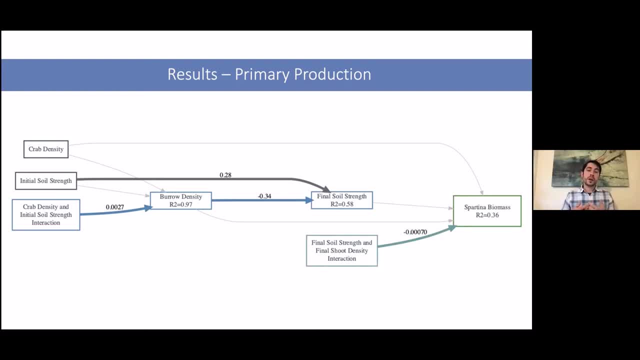 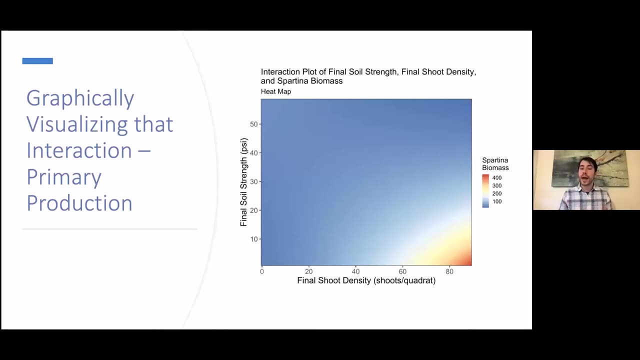 factor because we wanted to determine: does depth in the number of burrows have an effect on decomposition? And this final litter bag, mass, is that metric of decomposition And what this shows is that depth and burrow density by themselves do not affect the decomposition. 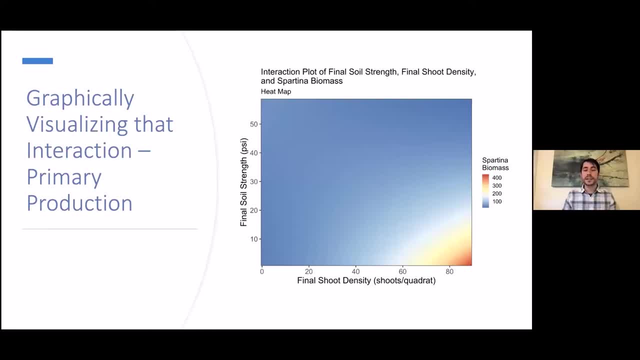 rate, But when burrow density and depth are combined, that is what's driving this final litter bag mass, this decomposition. And so again, I want to highlight this in a heat map to show this interaction. So on the x-axis we have burrow density, On the y-axis we have depth And the. 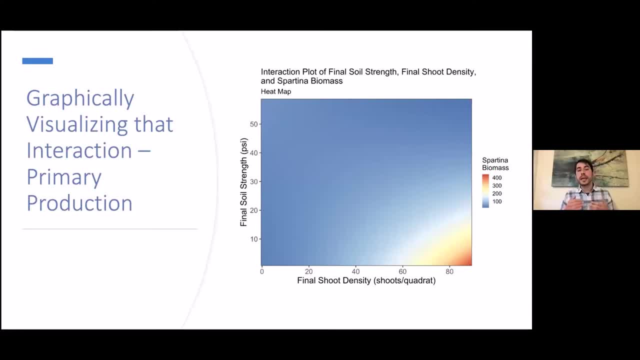 scale is inverted such that 5 is at the top and 15 is at the bottom, And we created it that way in order to sort of have it like you know: 5 is shallow and 15 is at the top, And so we have. 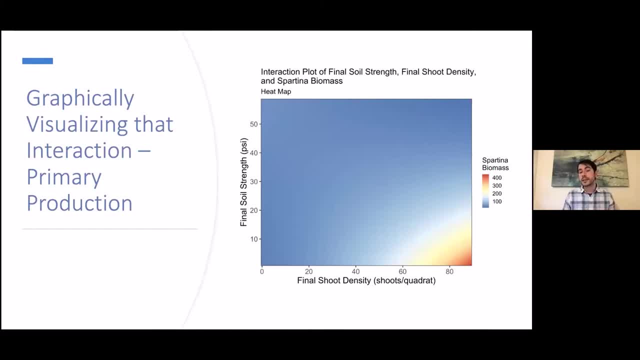 15 is shallow and 15 is deep, And so warm colors again are an increase in decomposition. So degree of decomposition just shows that As you get warmer in terms of color, that means you have more decomposition, And so what you see here is that the warmest colors are at the shallowest. 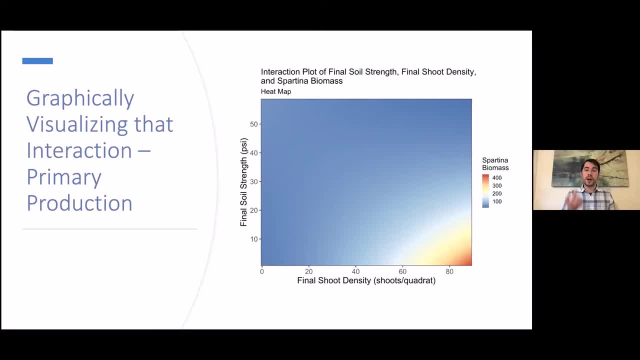 depths with the greatest number of fiddler crab burrows. So fiddler crabs are facilitating decomposition, but only at the shallowest depths. So that's a lot of information to unpack, And so I really sort of want to highlight this in a heat map to show this interaction. And so we have. 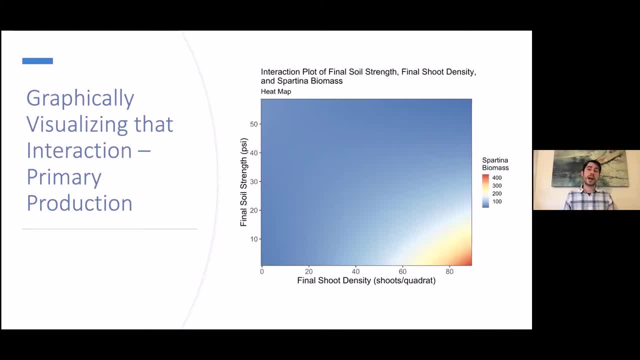 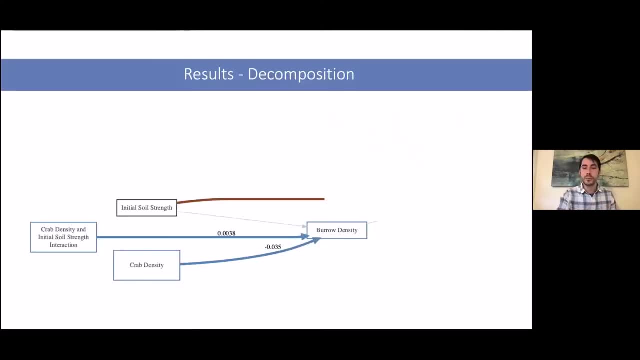 to talk about, you know, the bigger picture of how fiddler crabs are influencing these ecosystems. Before going into this, I did want to mention that I didn't show any plots in terms of differences between Plum Island and Nantucket, Because, while there were site-level differences, the two sites 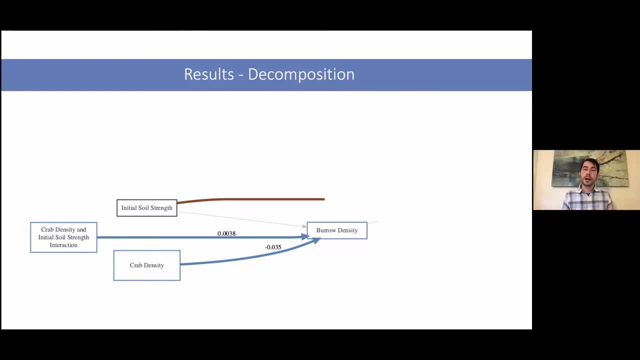 are unmistakably different. the patterns of change that we saw for these path diagrams, these structural equation models, were exactly the same. So the relationships were the same, even though maybe the degree to which that they occurred were different between different sites, which was a really 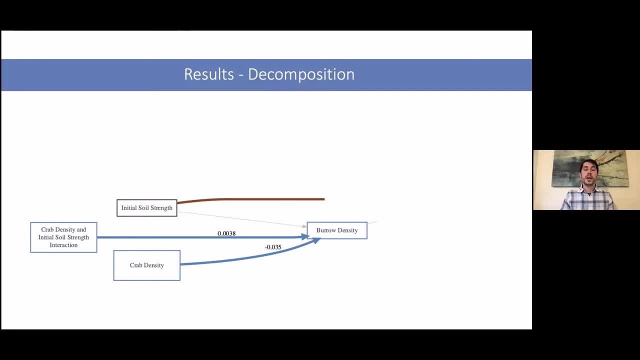 interesting finding, given the fact that the ecosystems are different. So we have crab density and initial soil strength and we know that the combination of the two affects burrow density. Now that we have that understanding, we know that burrow density influences soil strength. 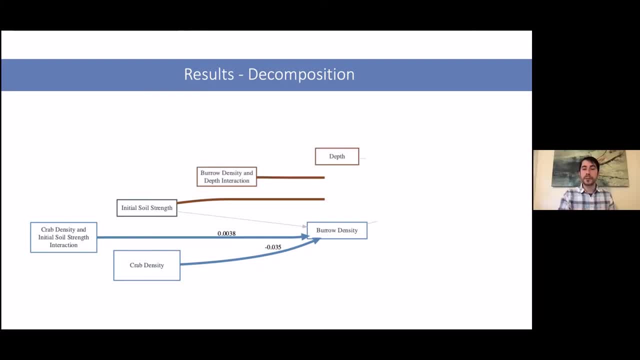 which is really what's driving the rest of the system. Soil strength affects primary production, Burrow density affects decomposition, which is really influenced by soil depth, And all of these different indicators combined affects marsh area, You know either, through increases in bioturbation. 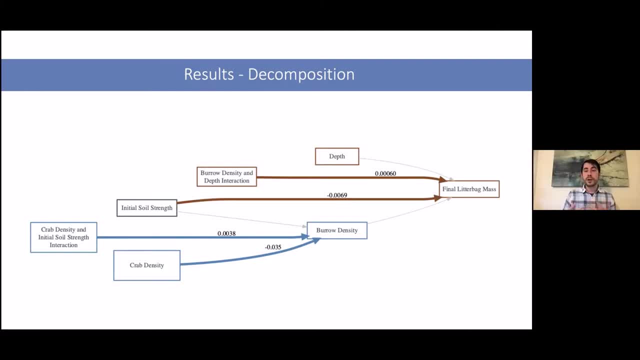 by fiddler crabs increases changes in soil strength, just changes in primary production, potentially facilitating that, And so understanding how this crab influences marsh area is really important, given the fact that we have critical environmental change and we have a lot of soil. 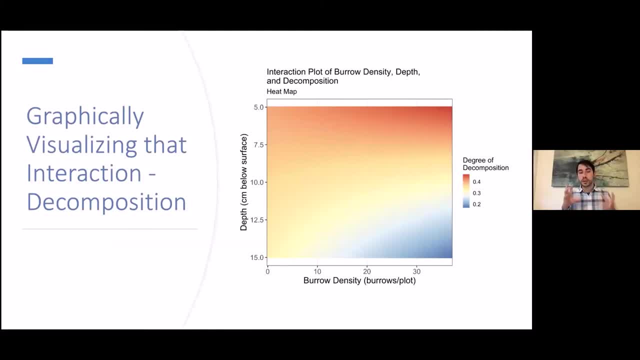 density change occurring in both Plum Island and Nantucket via climate change. And so here's that large map again of the Plum Island estuary. And so here's Plum Island and here's the city of Newburyport, and this city is right to the west of a huge barrier island. 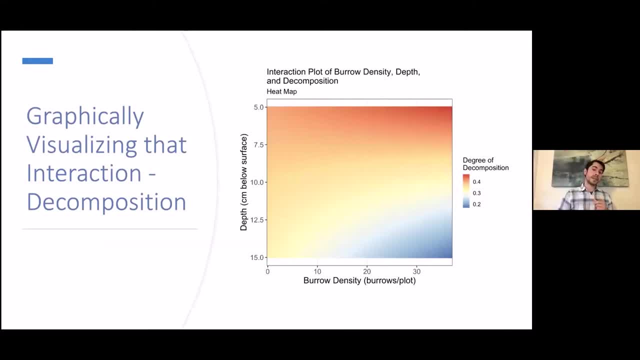 which is going to provide critical ecosystem services like buffer against stormwater, and then even aesthetic ecosystem services like birding or hunting or clamming, even just going, going out to the marsh and enjoying the peaceful outdoors. Meanwhile, Nantucket has very similar. 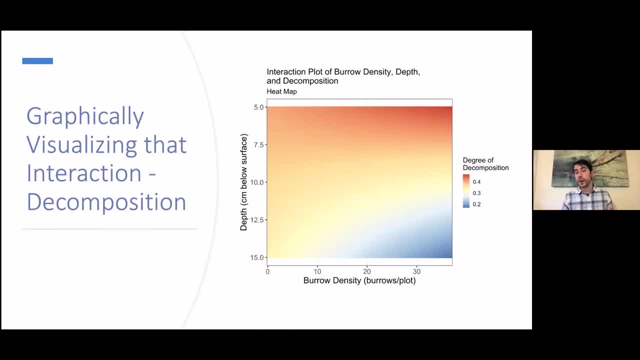 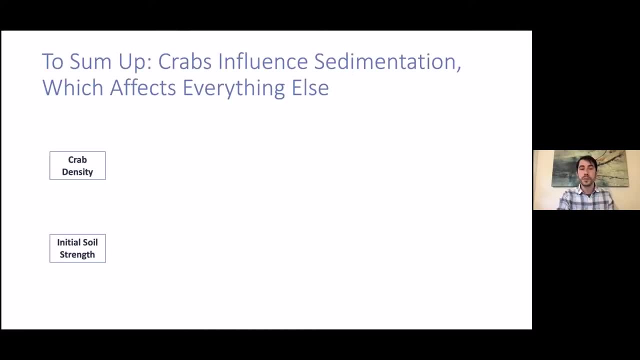 ecosystem functions and roles that the marsh plays. So here's, you know, a large map of Nantucket. We have Folgers Marsh, which is right up against the UMass Boston Nantucket Field Station, as well as a series of residential homes that use this ecosystem both for enjoyment, for 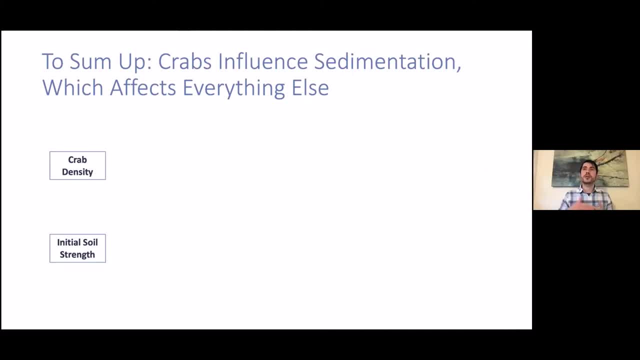 you know, looking out at this beautiful resource And this marsh is going to buffer some of the effects of flooding, as well as marshes, as well as storms, So these particular habitats are going to potentially be influenced by species like this fiddler crab. 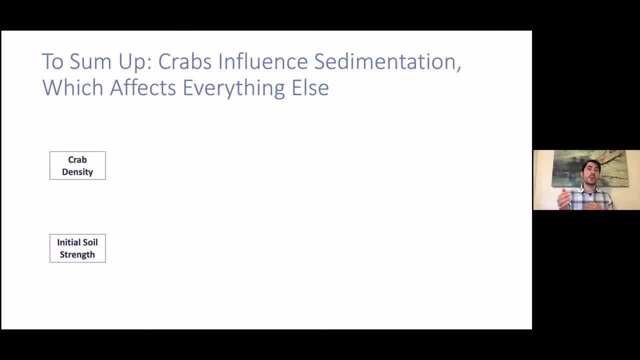 which will be important moving forward. So with that, thank you so much for listening to my talk and I'll take any questions. Awesome, Thank you, Michael. We do have one question in the chat already. The question is: how did you survey for a range of soil strengths and what was the variation in soil strength? 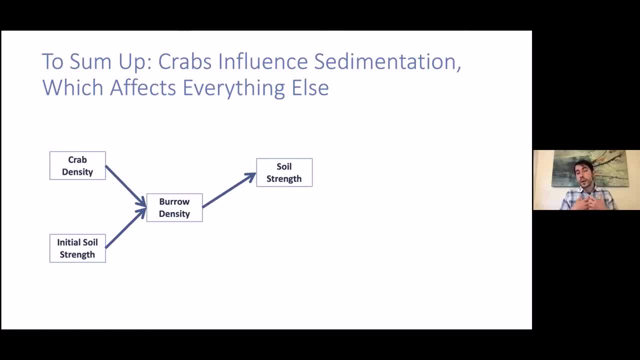 That's a great question. So essentially we knew that from previous research that marshes north of Cape Cod were stronger relative, more compact relative to marshes south of Cape Cod. So we knew that from a first approximation. But I was already doing work in. 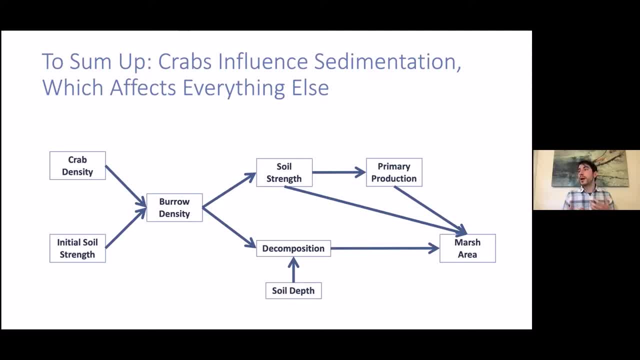 uh, Plum Island, I was doing work in Nantucket And so it seemed, because they had the different, different locations, that you know the biggest extremes really in Massachusetts. You can't get any further north in Massachusetts, any further south in Massachusetts than Nantucket and Plum. 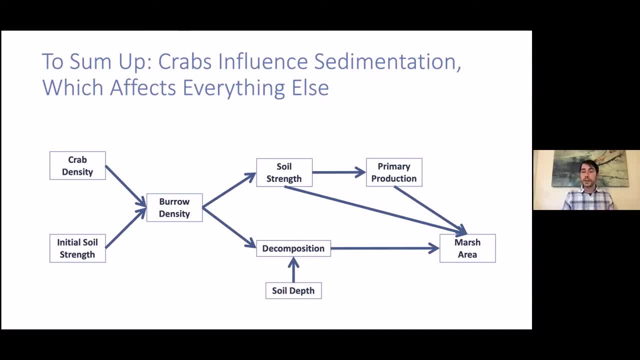 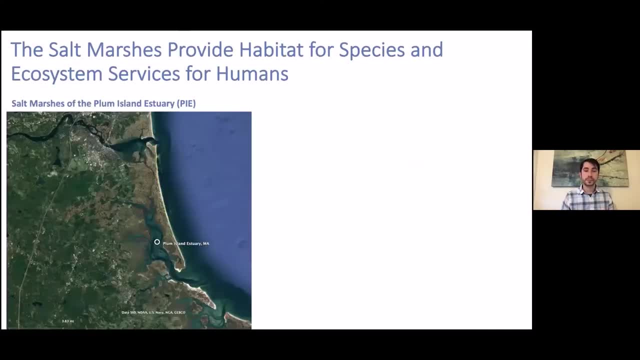 Island, that we saw that this was sort of, you know, a really great range of habitats to explore from. And then, in terms of answering your second question, there are significant differences between the two locations in terms of sediment compaction, And so you know, I think that's a. 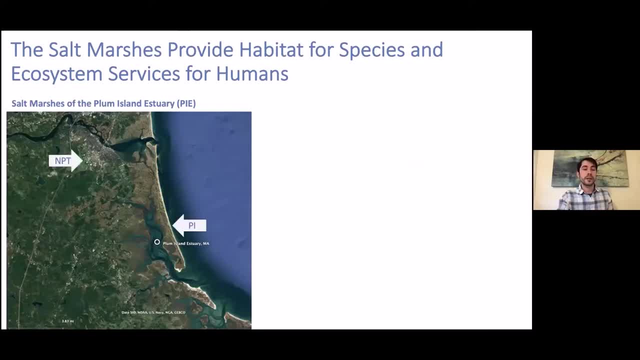 great question. So in Plum Island the sediment compaction on average is about 25 psi. It can get as high as about 60 or 70 in some locations, And in Nantucket it's about around 10.. So it's. 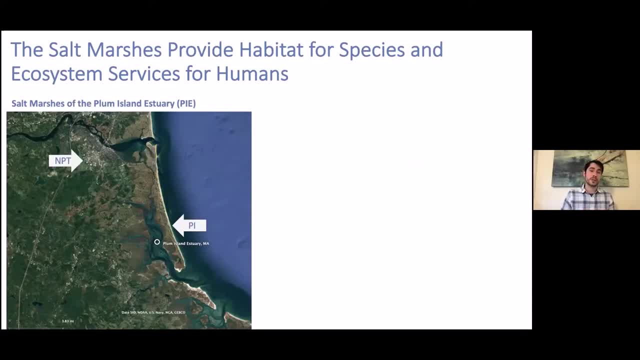 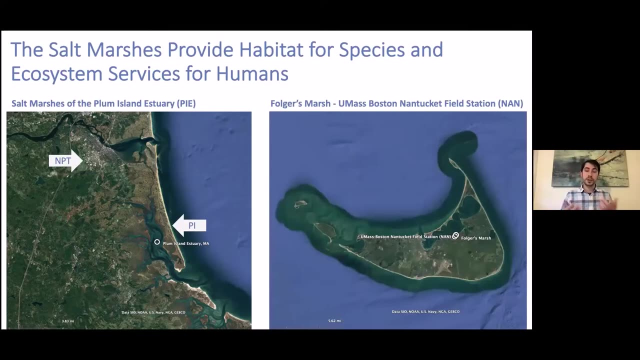 about 15 psi lower in Nantucket And that is about- I think my scaling is back- control and some of the measurements that we took for our cages. It wasn't perfect, There were some differences, but by and large our cages seem to be fairly. 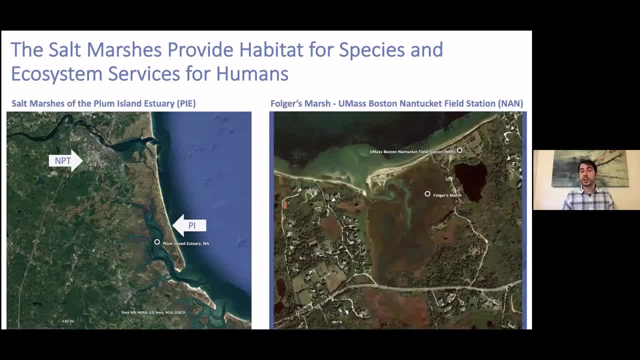 representative of the community, of the system, But that is, you know, a big, that is a big impact And to try to understand mechanism, it definitely will take, you know, creating larger cages, continuing to hammer home some of these questions and, you know, continuing to experiment. 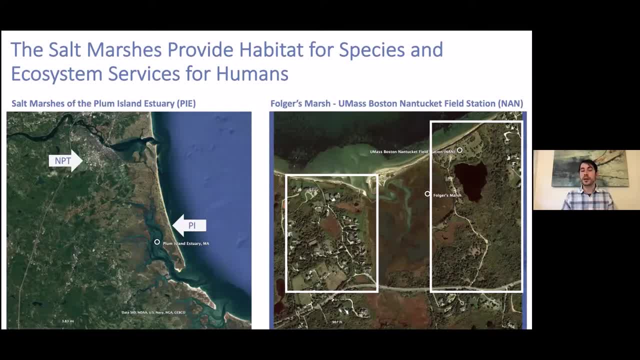 in that way, Great, Thank you. I guess at this point we can open it up to questions for either of our speakers. I see that Richard has had his hand up And like for my work. you know there's differences in the predator community throughout the course. 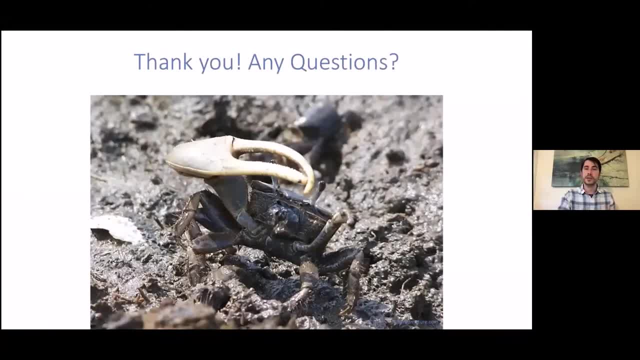 of the year. you know, both on the marine and on the bird side of things. And same thing with the resident marsh inverts, right, They recruit at different times, that sort of thing. So you know, the short answer is: you know, like the month-to-month temporal dynamics of 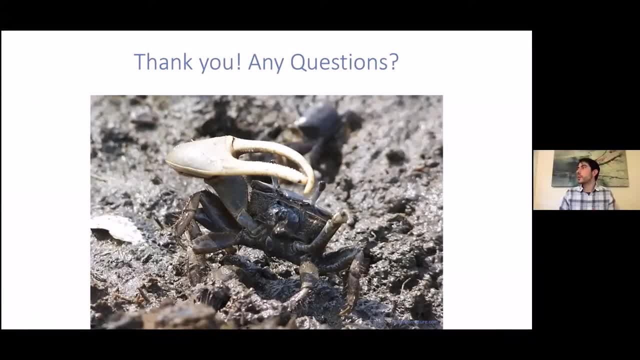 you know how the marsh food web changes and what that means for ecosystem functioning is really unknown. I think that there's definitely sort of excluding the animal side of things. You know, I think that there's. you know, we have a pretty good understanding of like, how things like. 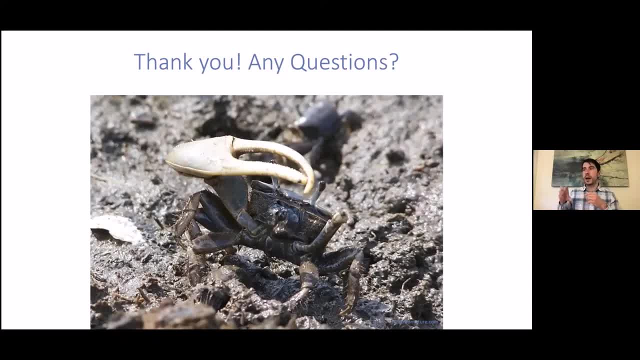 productivity and decomposition change throughout the year. right, More grass growth in the warmer months and decomposition generally occurs in the cooler months towards the end of the growing season. So you know, that's sort of the thing, But you know. as for like some of the other important 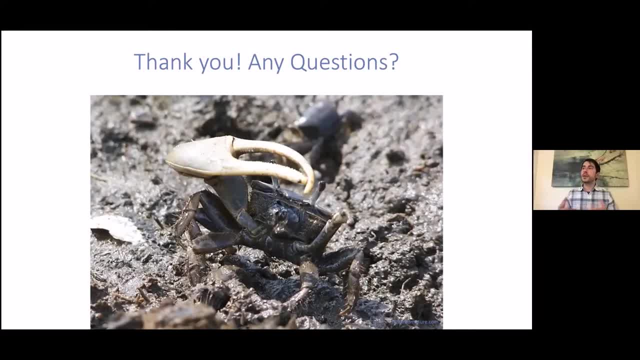 ecosystem functions. you know, I'm not really sure, I don't know if sedimentation rates vary throughout the course of the year or some of the other ecosystem functions, But you know the marsh is like is totally the place where these sorts of questions can be answered, I mean. 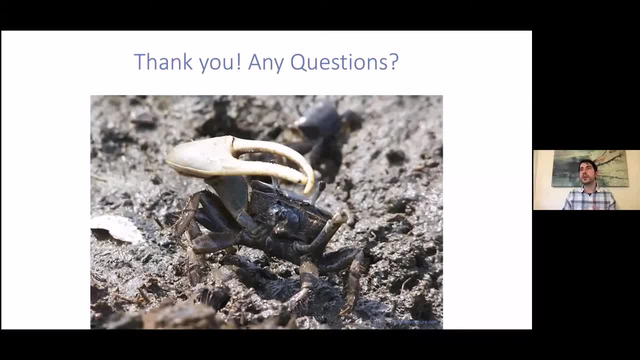 you know, really you're well, you know, those of you in New England know I mean, you know you're limited by like you know, basically like how much, how cold it is out there to get out and do your sampling. 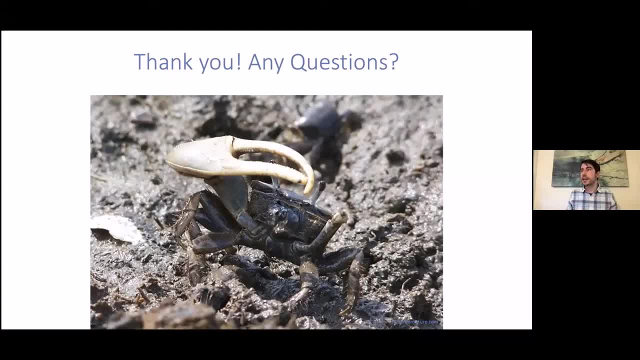 You know. so you know these are definitely questions that can be answered in the marsh. for sure It's not like having to go and scuba dive in 30 degree water or something like that. You know you can go out there and sort of measure ecosystem functions at different times of the year. But you know. as for like, how exactly that varies throughout the year, we it's an open question. So do we see a postdoc application funding application for spending time down on the island in January and February? I think it could be worse. Yeah, definitely If there's. if there's the funding out there, I say I say why not? So we've got another question for Michael. How did you measure marsh area? This person wants to hear more about your assessment of crab effects on on on marsh area specifically. That's a that's a great question. So in sort of my conceptual diagram, what I meant by marsh area is is more to more to the point of if filler crabs are going to have sort of localized effects on marsh structure that that potentially could scale up to the entire marsh. And so what I mean by marsh area is just sort of the, the amount of area that encompasses salt marshes specifically, So the amount of area of low marsh versus high marsh, and then total marsh as well. I mean, in fact, this is a question that I'm I've been asking for another chapter of my dissertation, which is: if you do have these localized changes in in um filler crab effects on ecosystem functioning, how will that affect sort of like the totality of of the marsh? And so that question is that I'm I've been posing that. towards Plum Island. Thankfully, because there's the Plum Island LTR, there is a large data set of actually going out and measuring the spatial area, the spatial extent of the salt marsh of Plum Island And so understanding exactly how, more or less, how much low marsh area there is and how much high marsh area there is. 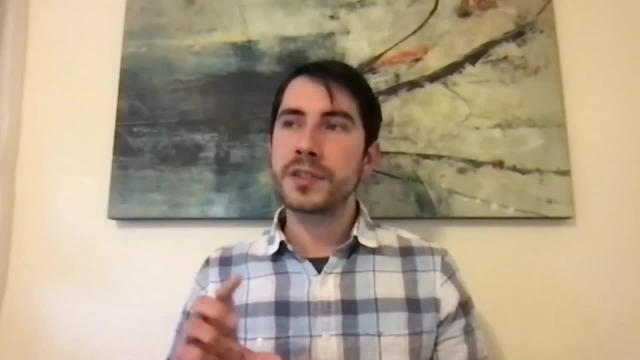 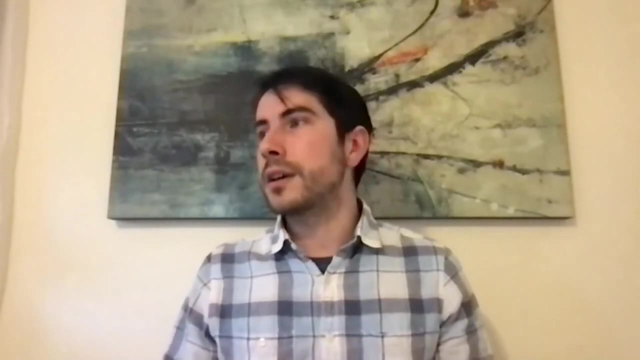 There have been folks that have been doing this using satellites, using transects, using on the ground, field, field work to try to understand, you know and extrapolate from there, And then taking that and trying to use a system dynamics model to understand how the relationships between the local and sort of the larger scale to sort of not just change, decomposition but nutrient reuptake, as sort of like seeding for the next season, um which I wonder if anybody's looked at that, I don't know. Speaking of postdocs, No, I mean, I think that this is a um. yeah, I mean, I think this is an important thing. That's why I thought this question about seasonality was was so interesting, because I mean, it's, you know, it's really. it's really striking in in New England marshes, where there is such a big um, change throughout the well, throughout throughout the season, for sure, But, like you know, if you compare the dead of winter and, uh, um, you know, peak, peak productivity in the summer, whereas in, in in Southeastern marshes, like where I am right now, it's, uh, most of that. like you know, that brown stuff sort of stays standing throughout the throughout the year, uh, or throughout throughout the winter, Um, uh. so, yeah, you know, I, I you'd think, like you know, sort of late, late season, like decomposing is, is uh, uh in New England. marsh is probably really, really important for how things kick off, uh, in the early spring. Um, and I, I, yeah, I'm not sure, I'm not sure if that, um, those sort of the names have been investigated. but Yeah, I wonder also if, like, if they have like a cyclical pattern where, like, early season they eat decomposed alternate flora, then they switched to diatoms, then late season they eat alternate flora, decaying eat alternate flora, because maybe there's not as many diatoms. in, you know, the early season because it hasn't gotten quite warm enough, And you know, or then again in early season there's sort of like that pulse of nutrients. you know that, you know, uh may foster a huge bloom of diatoms early season. So that might be it as well. 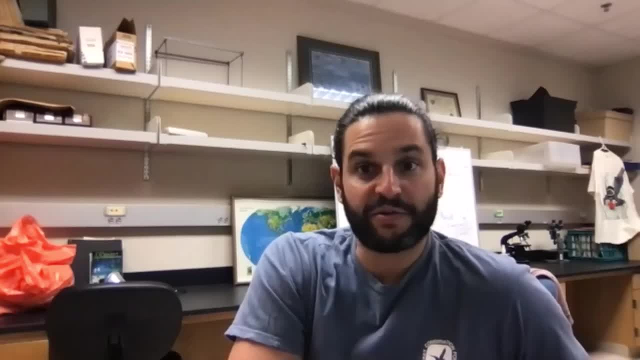 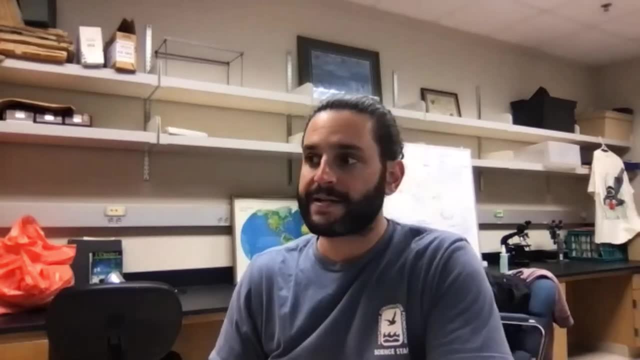 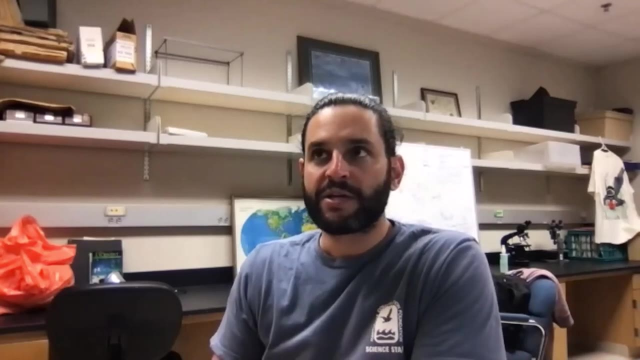 So yeah, I think that uh snails, uh um, I don't know about the literary and literary, but I know that literary, uh the big snail down here- definitely switches um from eating eating diatoms on the sediment to uh decomposing standing dead tissue to sometimes even eating live. 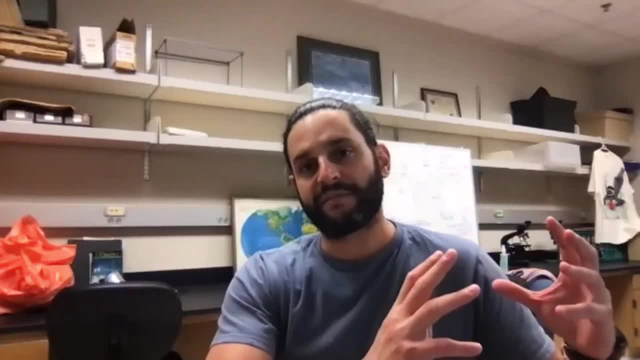 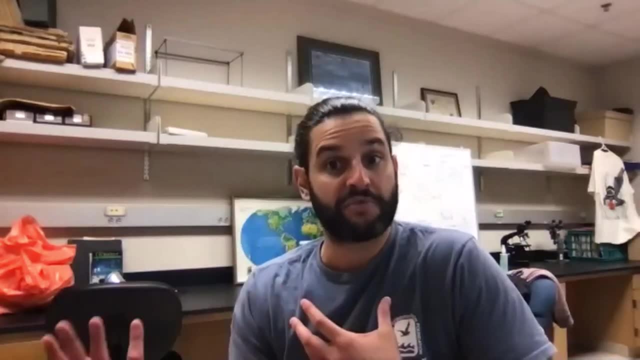 tissue throughout the year. So, yeah, I don't know if it's like a seasonal thing that happens all the time or if it's a year to year. Um, you know, I don't know if it's a seasonal thing that you know, big, big uh, uh, spring bloom. So everybody goes for the uh, for the benthic uh. 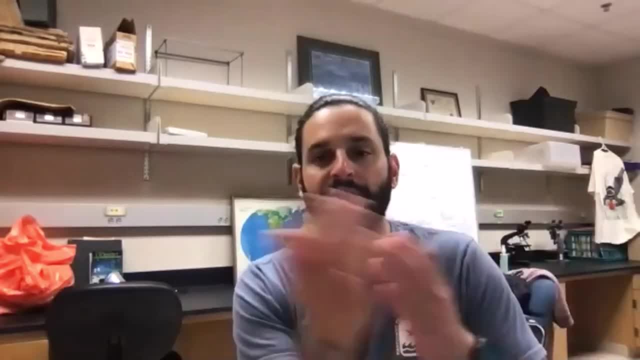 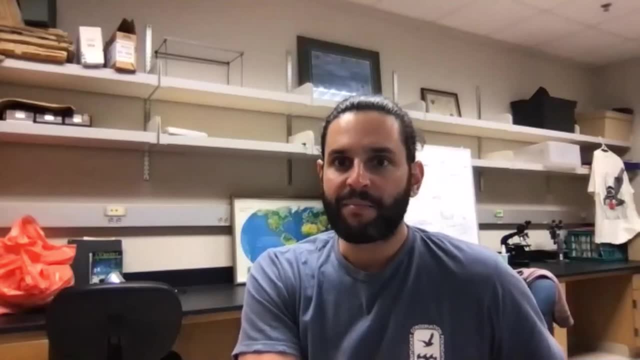 algae or what. but um, yeah, those sort of dynamics are untapped and really interesting because they can control a lot of uh of marsh processes. I agree, Yeah, So in your experience with um- I know you don't, you did a lot of work with sasarma, So did they- are they primarily just consuming on alternate flora or what are? do they change their diet as well at all? Or do you know? Um, yeah, I'm not sure, The purple marsh crab, sasarma ticulatum? um, I am, I'm not sure if it changes its diet throughout the year. um, as well, Actually. 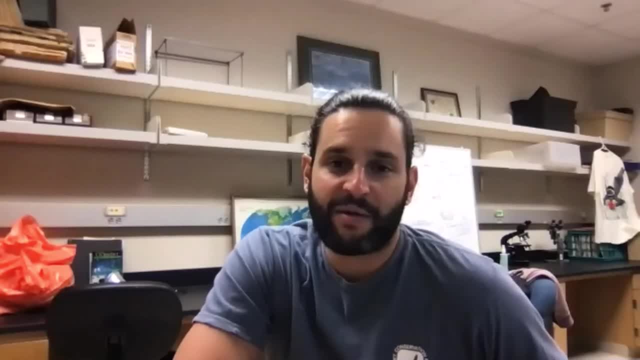 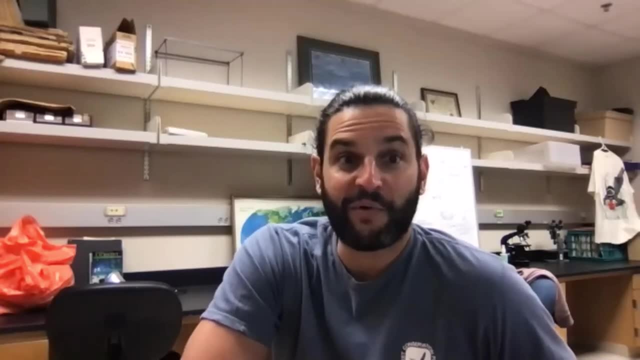 uh, a friend of mine uh here. uh, who's in David Johnson's lab? uh, Serena Whittingham is uh studying a similar thing. Um, she's uh looking at some of these dynamics here in Virginia marshes. 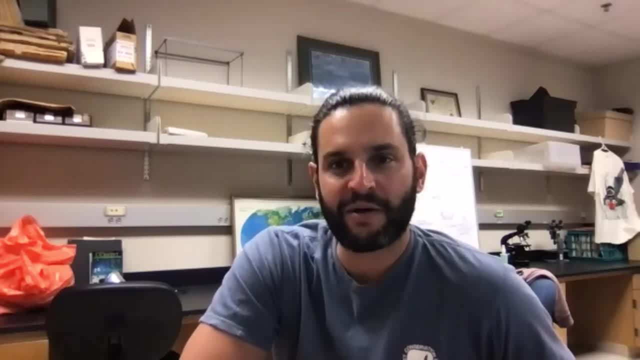 but um, yeah, it's another untapped uh uh question. Yeah, Serena, Serena's great. Yeah, I met her up when she came up with uh David up to uh to pie, So that's cool, It's very cool. 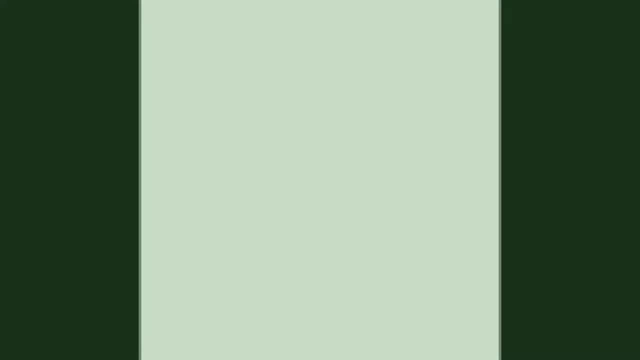 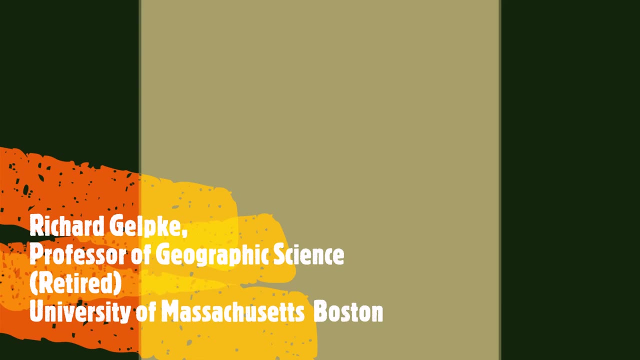 Um, so I had written down one of the uh questions that we kind of kicked down the road. um, for the panel, uh, panel questions. So I'm going to go ahead and address that And then maybe, Yvonne, you can ask some other panel questions after that if we, if we still have time. 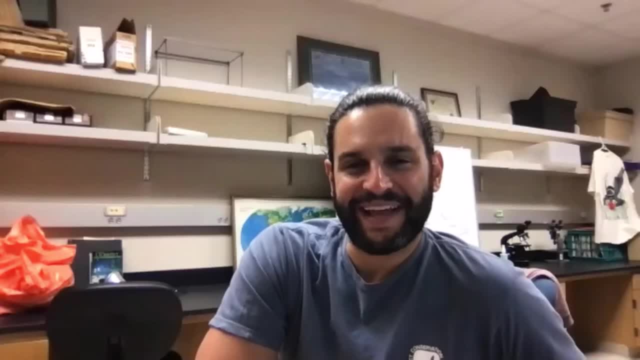 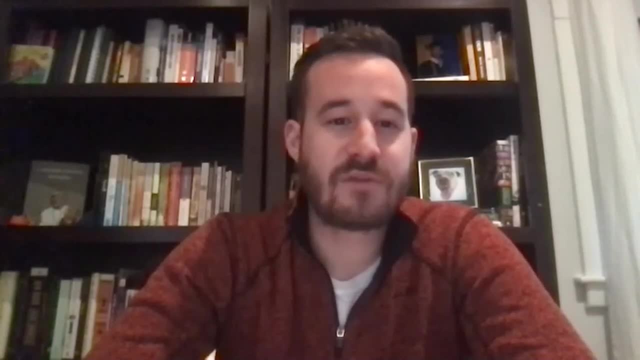 But, um, so, yeah, I uh a really cool question, um, you know, came up about, uh, about the blue crab. Um, you know, this is uh, uh, the blue crab's a, you know, an iconic coastal, you know. 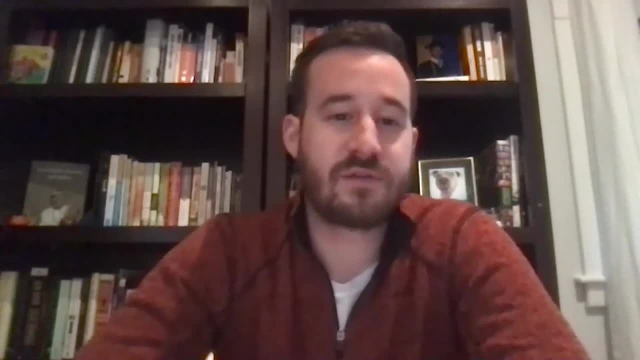 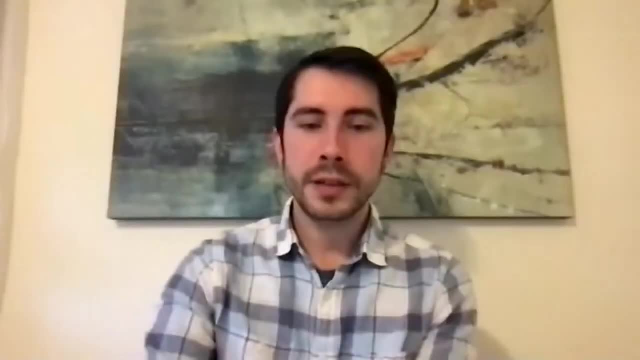 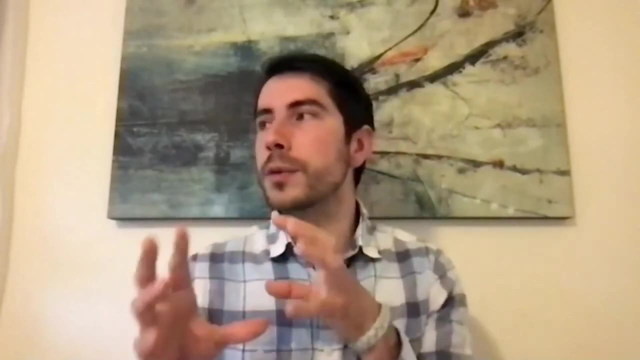 the uh, it seems like there's going to be, uh, you know, a similar story with with the blue crab right, Michael. So, like the- uh, you know, sightings are very much like that, like that cool map that you have with the dates of feather crab going up. you know it's similar stuff with. 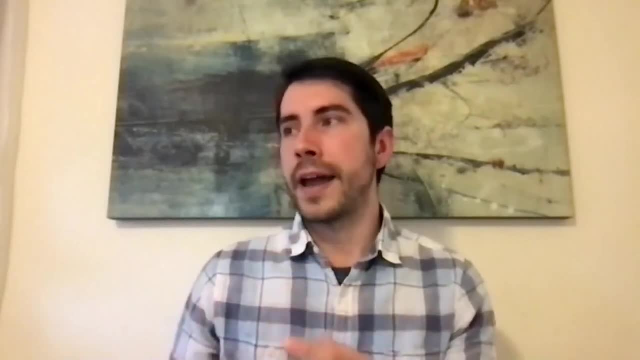 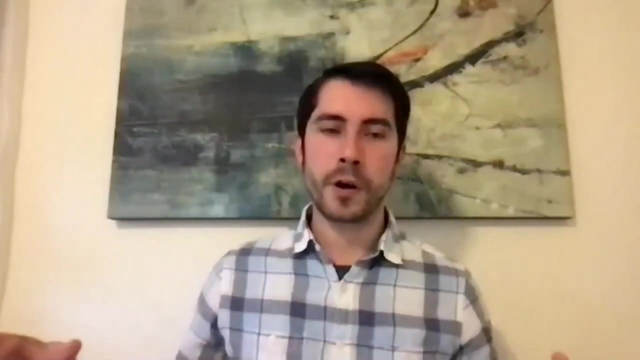 blue crabs. right, Yeah, I mean, um, that's that, that seems to be the case. I mean, um, there were before. I mean it was slightly different from from fiddlers, because there'd be patchy instances that they would sort of show up, then they'd be gone for like. 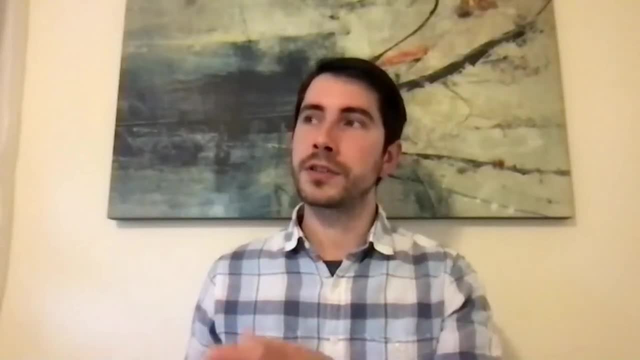 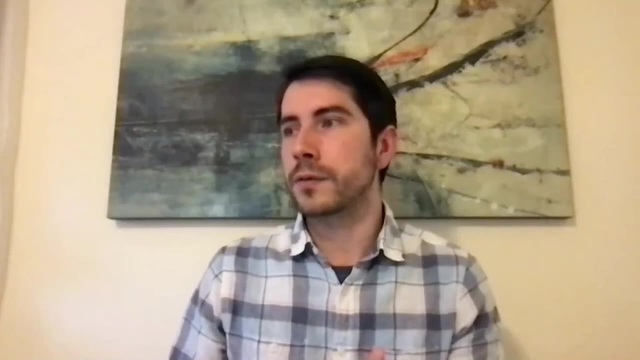 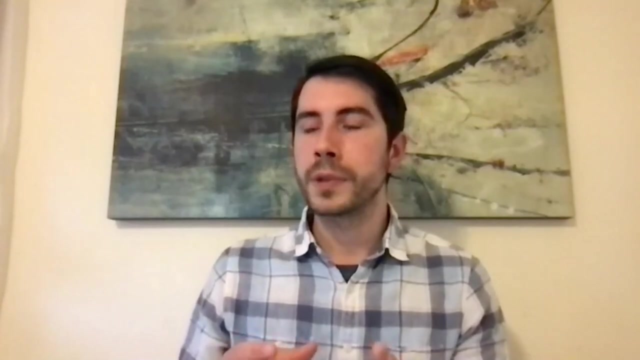 10 years and they'd come back with blue crabs. Yeah, From my understanding. But um, but lately, like the past, like three or four years, it's been more regular. It's been like on one year off one year on one year, And then I think even last year one was found, And then now this year, 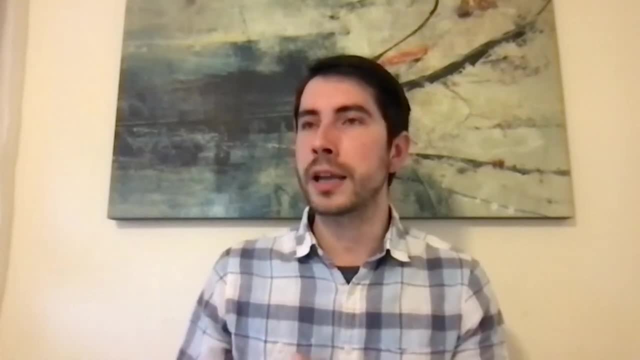 there have been five, So it's it's increasing in frequency, So it seems it seems to be tracking that more, more regularly And so you know this is a, this is a um, um, a really interesting. 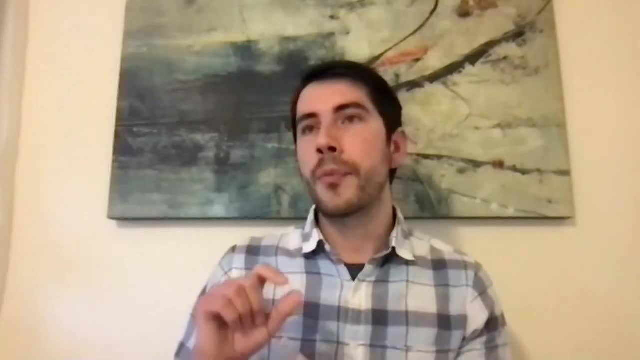 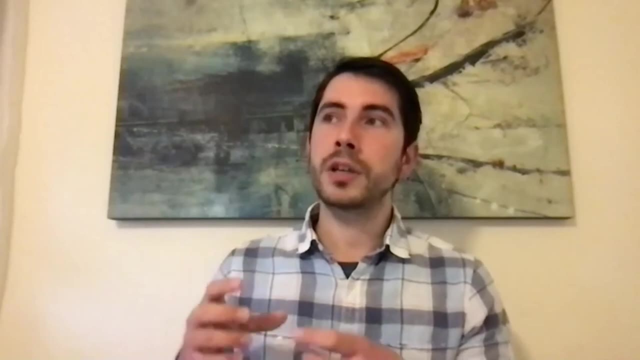 tie-in between both Michael and I's uh research, because you know blue crabs, basically wherever they are in any ecosystem, but especially salt marshes. you know they are, more or less, you know, the top predator, uh, you know. besides, like you know, 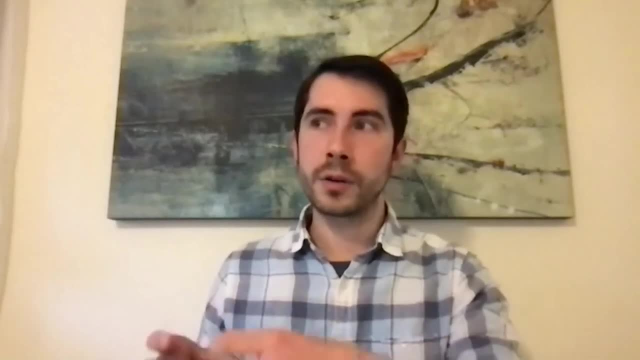 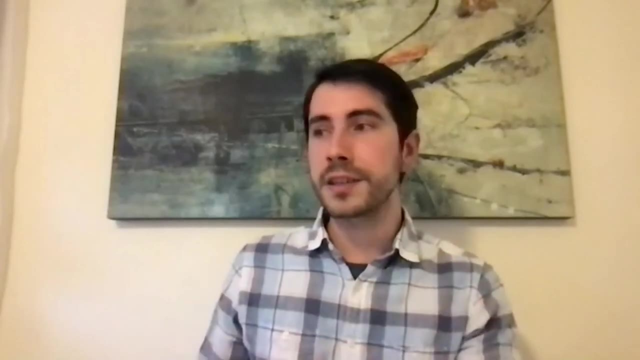 ambient, um, um, predators that come through like sharks and stuff like that, uh, you know, like. as for the species that are like coming in and out of the marsh, uh, you know, every single day. uh, blue crabs are right at the top, right there, Um, uh, they are at the top of a, of a. important trophic cascade here in the Southeast where um you know, if their, if their numbers go down um their prey, uh a snail can overgraze marsh grass Um. another interesting thing that blue crabs do um in the mid Atlantic, is they um outcompete uh, green crabs They they eat. green crabs and they keep green crab numbers down And I write this obviously you know uh a big uh topic of of interest in in New England and and uh you know marsh ecology in general. on. the East coast is, uh, is green crab stuff And, and you know the the research that I've read is that if there's blue crabs around, there aren't going to be- uh, there aren't going to be- blue crabs. there at least aren't going to be as many green crabs in the marsh. They might go somewhere else or something like that, But um, you know. so these sort of like this is, it's a really interesting thing, as, as blue crabs, you know this novel, uh, uh, you know, important like. really powerful predator that eats a lot of different things. you know, I guess, uh, I guess the, the, you know- marshes are cool from an ecological standpoint, um, because there's a lot, of, a lot of fun things to do. And then you know that, uh, you know, is, is, is like expanded. you know, 10,, a hundred times when you think about their importance to. uh, you know, have a good night everyone, Thank you.